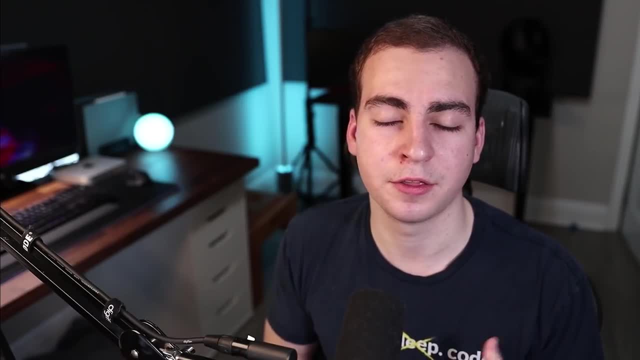 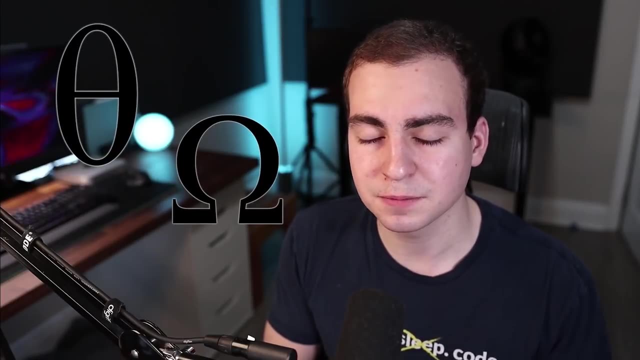 on the whiteboard. Now I will mention that I'm not going to be covering other time complexity analysis. So we're not going to be looking at a big theta, big Omega space complexity. We are simply looking at big O notation, And in a second I'm going to explain what that is. 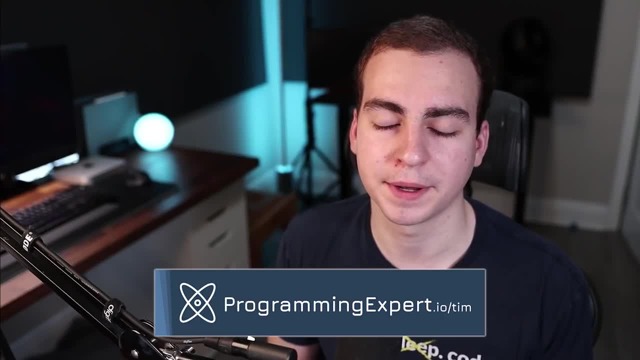 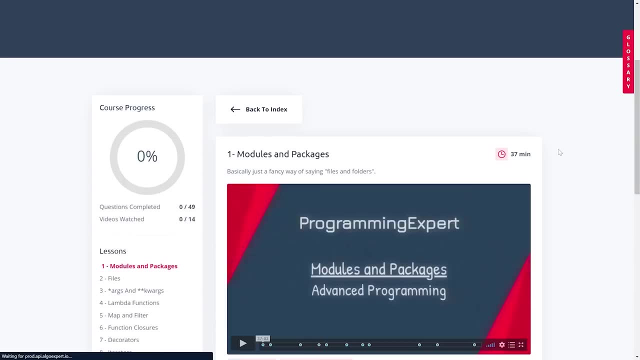 Now, before we get into it, I will mention that I do have a course. it's called programming expert. teaches fundamental programming, object oriented programming, advanced programming. tons of practice questions, tons of projects. You guys can check it out from the link in the description and use discount code Tim. With that said, let's go ahead and get into. 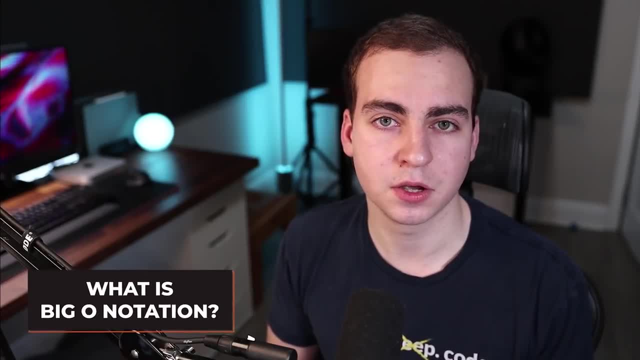 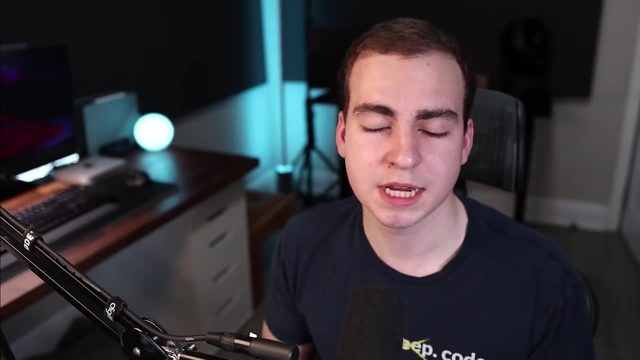 the video All right. So I want to begin by just discussing what big O notation is very generally and why it's important for programmers of all types to actually understand this concept. So big O notation is essentially a tool that we use to analyze different algorithms. 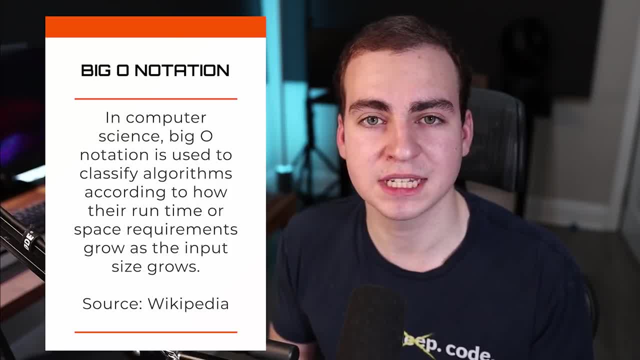 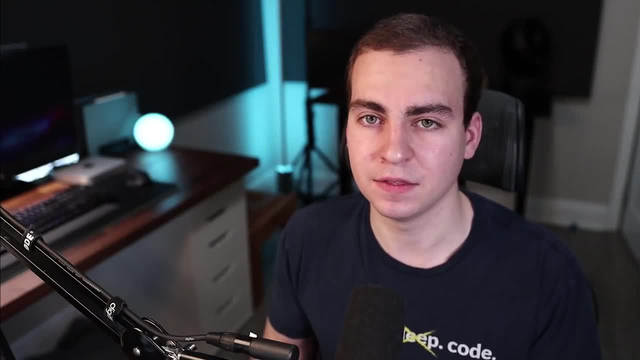 data structures and just sections of code and figure out relatively how much time they're going to take to execute, Based on the approximate number of operations that need to be completed in the worst case. understand that sounds a little bit confusing, but the idea is we want to be able to look at two 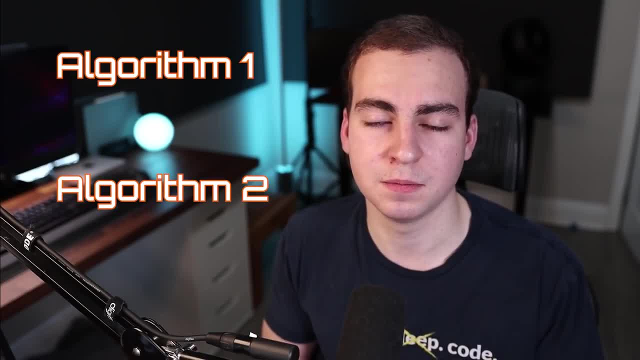 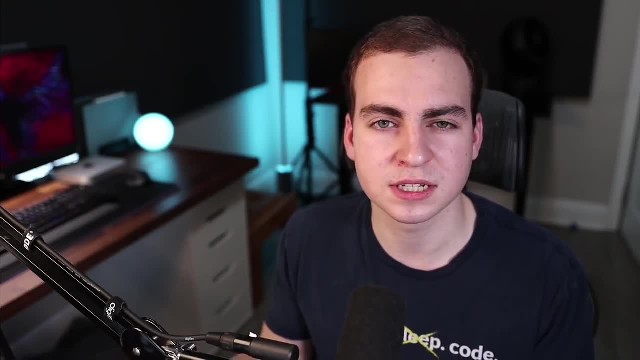 different algorithms and very quickly determine which one is going to be more efficient based on its big O notation. So big O notation again as a tool. we're using it to compare different solutions, different algorithms, different data structures. The algorithm is data structures. that 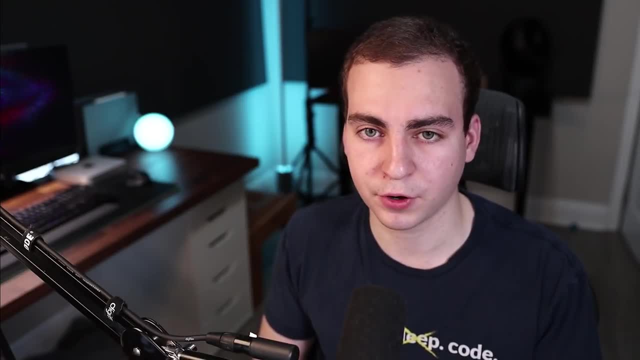 have the best. big O notations are typically the ones that we prefer because they're going to be the most efficient, They're going to take The least amount of system resources or they're at least going to execute the fastest. Now, big O. 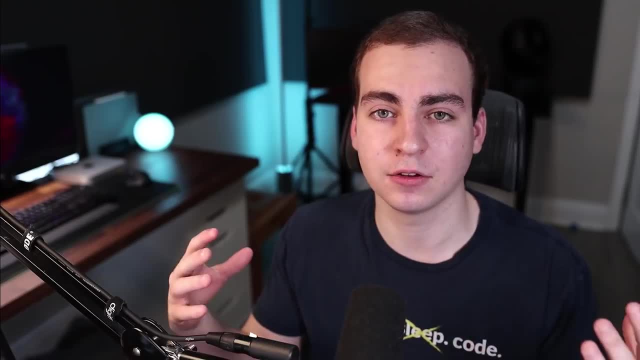 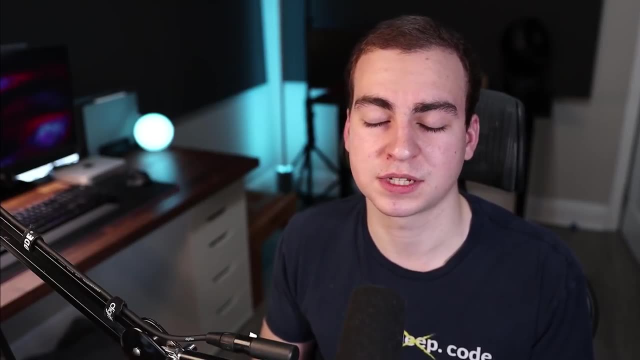 notation is really concerned with what happens when we scale our problem to a very large size. So we're not really wondering what's going to happen when we sort five numbers or 10 numbers. We're concerned with what's going to happen when we sort a million numbers If we're comparing, say, different sorting. 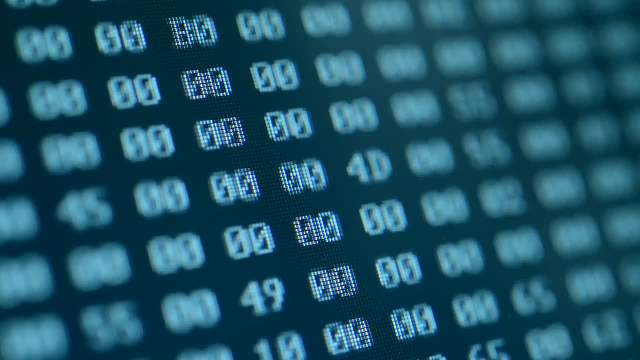 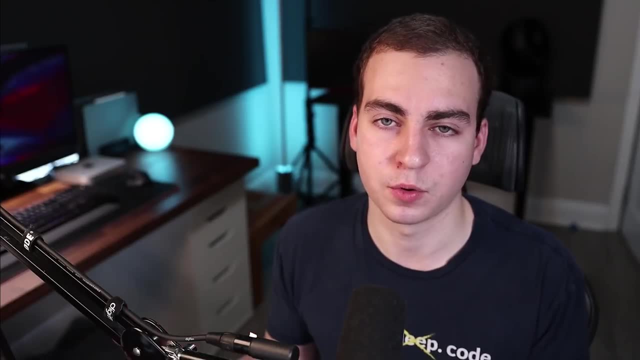 algorithms or what happens when we pass the worst case scenario of numbers to be sorted. So big O notation, worst case scenario for very large inputs. That's what we're focused on. So we're going to be looking at what we're focused on. Okay, That is a very general introduction to big O notation, The reason. 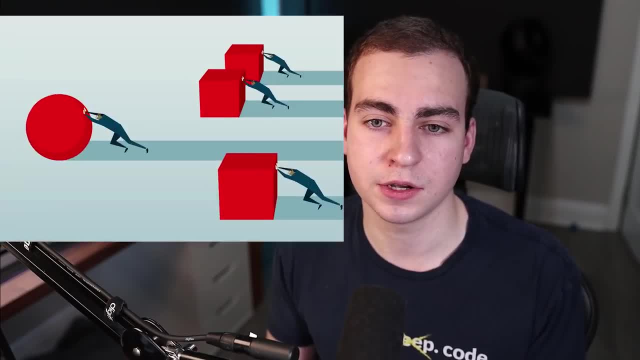 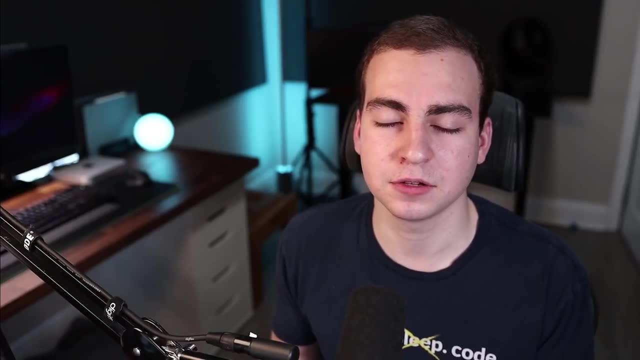 it's important for us to understand this is because there's a lot of scenarios where we can write code that solves a problem but doesn't do it in an efficient manner, And the only way we know what's not happening efficiently is if we understand relatively how many operations this code takes. 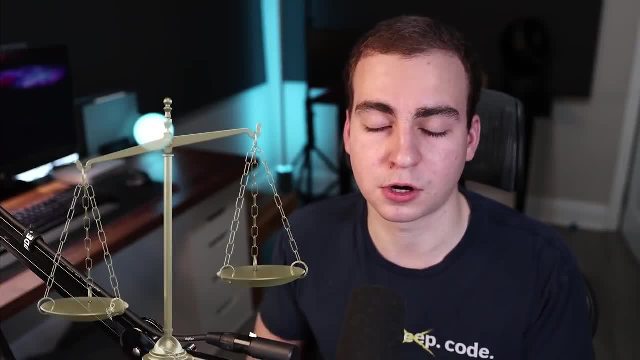 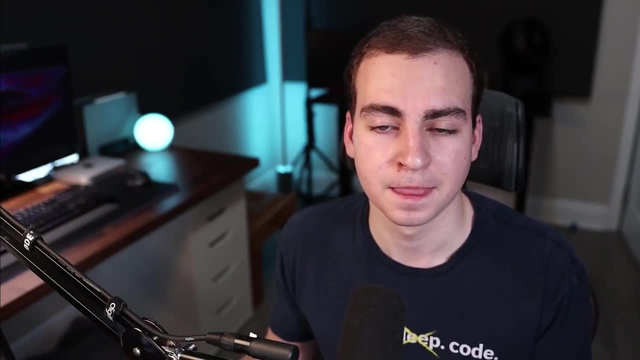 compared to another, more optimal solution. So this is our comparison method. without this method, you really have no way of understanding. you know how long your code's going to take to execute, And that means that it might work for a small input, but if you pass it, say a thousand. 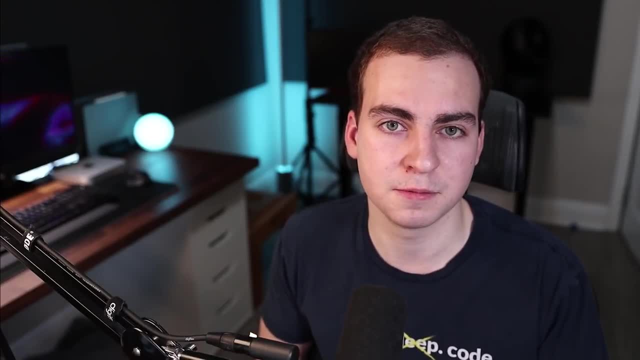 numbers, or 10,000 numbers, or a large list of strings, or whatever the input type is, it may take a really, really long time to execute and may even be in feasible. There's a lot of algorithms that you and me have probably both written in the past where if you fed them, say, a million numbers, they 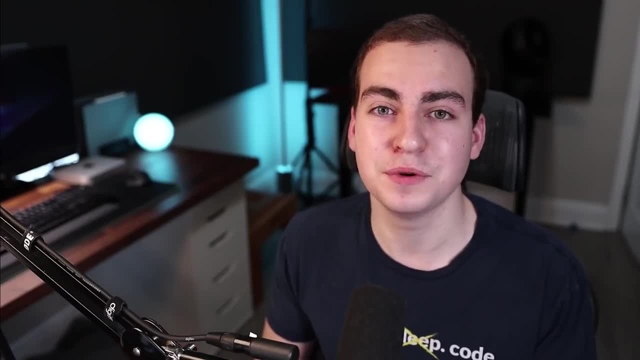 may actually take years, decades, hundreds of years to execute, based on how inefficient they are and just the math that goes on behind the scenes here. Anyways, we're going to start looking at a ton of things. We're going to hop over to the whiteboard and start explaining to you kind of the theory. 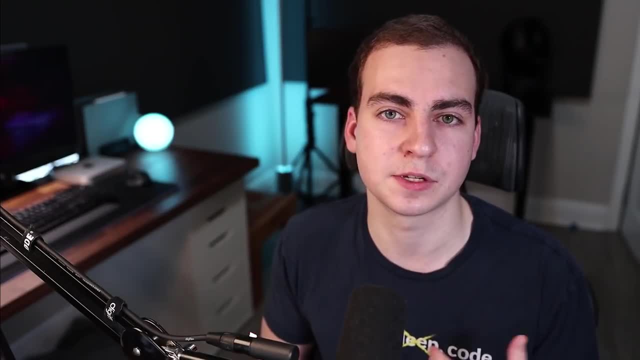 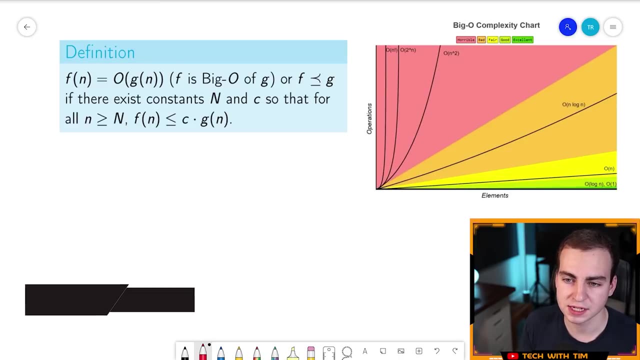 behind big O and how we find the bigger notation of specific algorithms. All right, So I'm here on the whiteboard. I'm going to ask you to please not be too intimidated by the math that you're already seeing. It's going to be really simplified once. I start going through a few examples So, as I 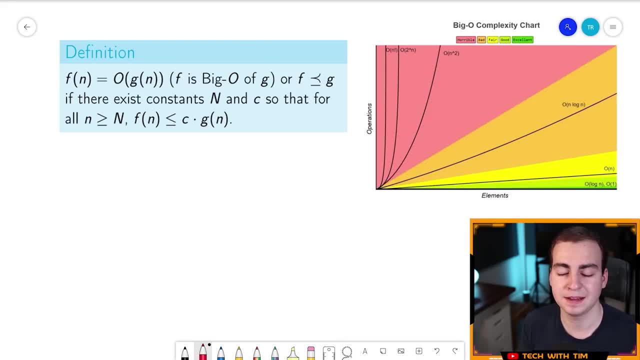 mentioned before, when we're talking about bigger notation, to actually find the bigger notation or the bigger function that represents an algorithm or a data structure, whatever it is, we need to be able to figure out the approximate number of operations an algorithm is going to take. Okay, So 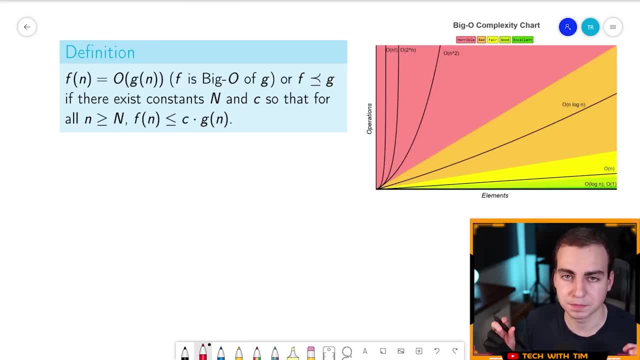 the first step that we always do when we're analyzing something for its bigger notation, to try to compare it against something else, is we figure out the approximate number of operations that this algorithm takes. We're then going to use those to simplify and find the big O function, or 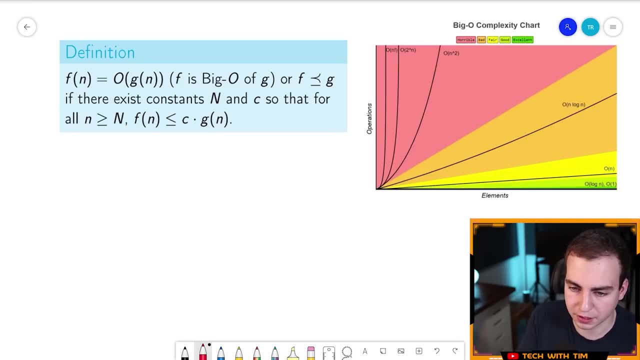 the bigger notation. Okay, So let's write a super simple example here. Let me just get clicked into the screen and we'll start going through. So I'm going to say total is equal to zero. I'm going to in N. I'm going to explain what N is in a second, and hello cats just decided to join me here. I'm 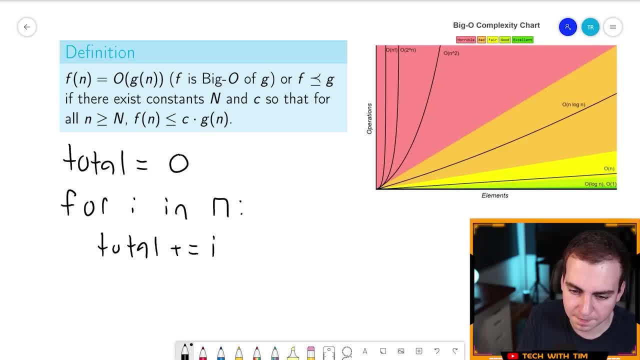 going to say total plus equals I, and then I'm just going to print: Okay, So this is my elk. Now, the first thing to discuss here is N- you're going to see this a lot- and refers to the size of our input. So, as I mentioned before, when we're talking about bigger notation, we're really 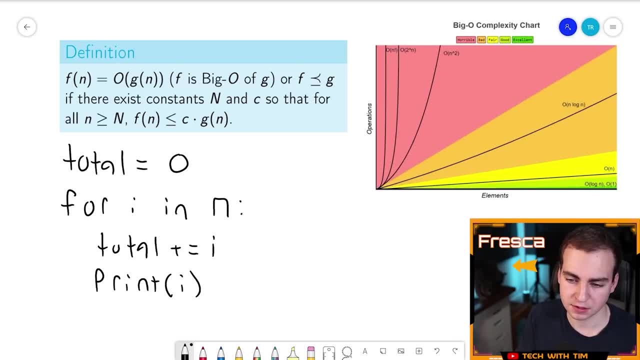 concerned with what happens when we have really large inputs. So N is just a placeholder to represent the size of our input And we write our big O, Oh function and the number of operations relative to N. So in this case, here if we're counting the 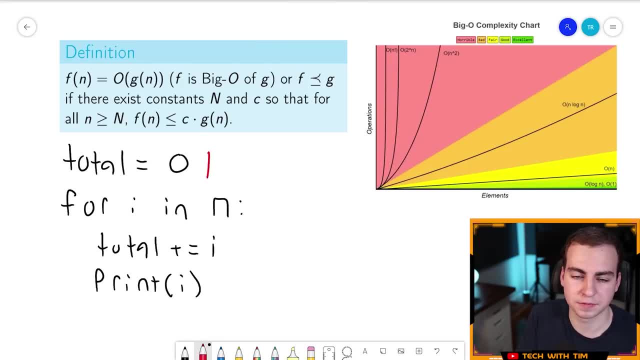 number of operations that are going to occur. we have one operation to define the variable. We're going to have N loops. It's going to happen N times because N is the size of our input, right? So I'm going to say N, and then we have two operations happening inside of the four loop. 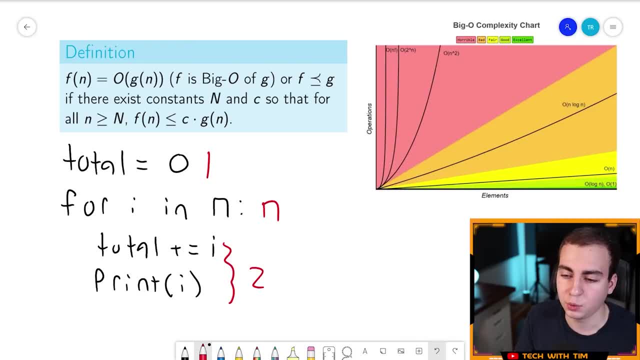 So if this four loop happens N times and we have two operations, we have a total of two N operations happening in the four loop. So we're going to say two N plus one is the number of total operations that this algorithm is going to take. 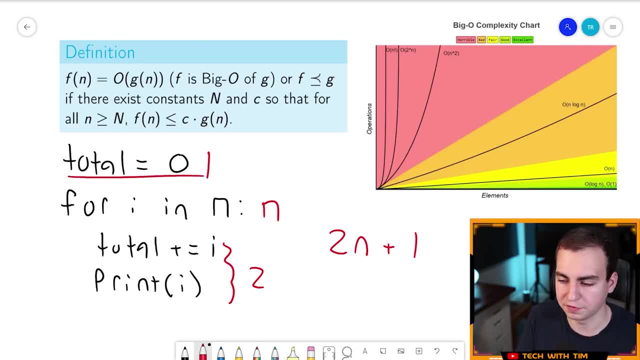 Cause we have one here and then N times two, two N. hopefully that is clear. So what we're going to do is we're going to write this as what's known as our F of N. Okay, I'm going to start going through this definition in a second. Let me just erase this part here and 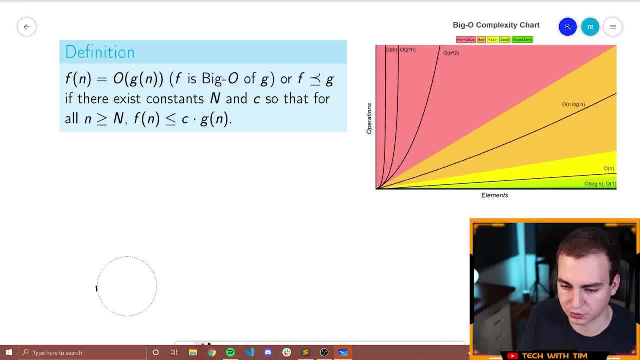 move over the two N plus one. Okay, So actually we'll just rewrite it over here. Okay, So F of N is going to be equal to two N plus one, and F of N is going to represent the number of operations that our algorithm takes. So now let's look at this definition. 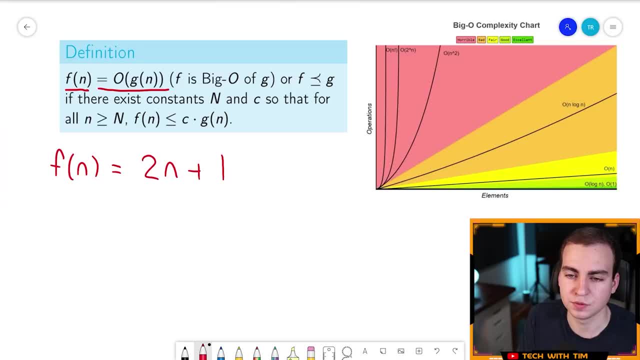 So this says that F of N is equal to the big O of G of N. So where F is big O of G, you can read it that way: If there exists constants, capital, N and C, so that for all N greater than or equal to uppercase N, this inequality is true. Now it's important to note. 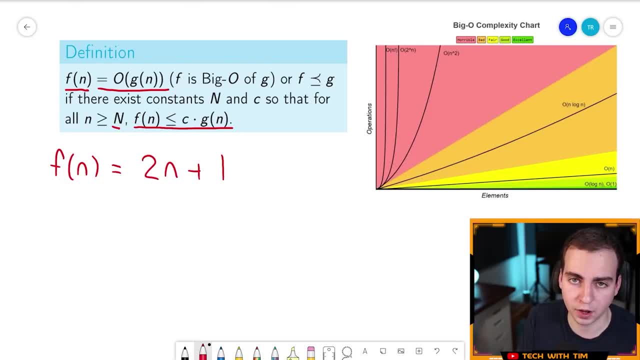 here that C and capital N have to be at least one. So one or greater, uh, and we'll go through this makes a bit more sense. So let me just write out this inequality We have: F of N needs to be less than or equal to C times G of N. So just to stop and explain something here: G of N is the function. 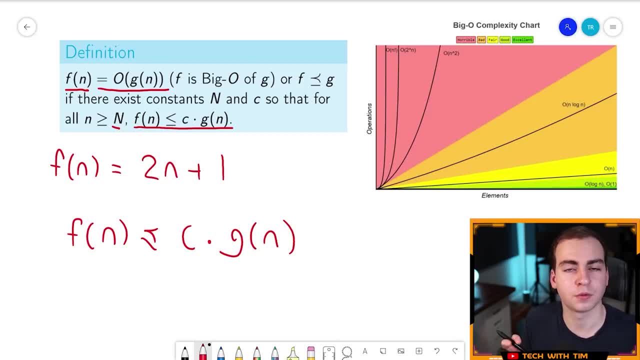 that we're looking for, which is going to be the big O function or the big O notation of F event or of our algorithm? Okay, G of N is really what tells us approximately how long this code is going to take to run, based on the input in this case. And okay, So everything refers to N again. 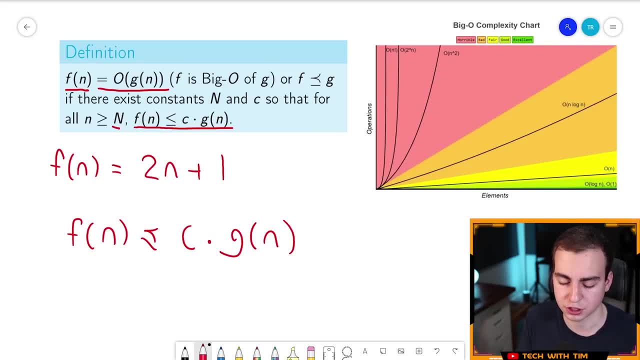 we're really concerned with what happens as N gets to a very, very large number. So we need to find something that satisfies this inequality, And we want this right-hand side here to be greater than or equal to N would be as close to N as possible. The reason I'm saying that is: 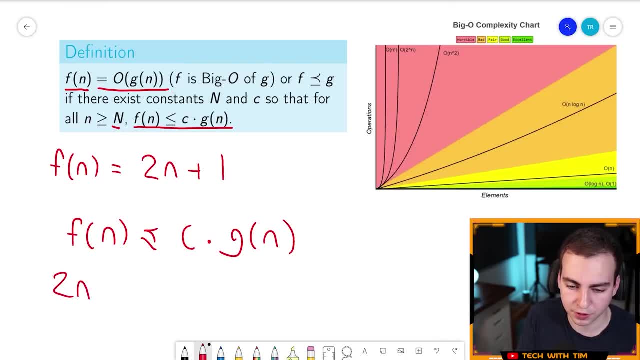 because any of you who are kind of working this out in your head already can probably realize that if I substitute in two N plus one for F of N here, and I say less than or equal to C times, you can pick some very, very massive function, maybe something like N to the exponent four. 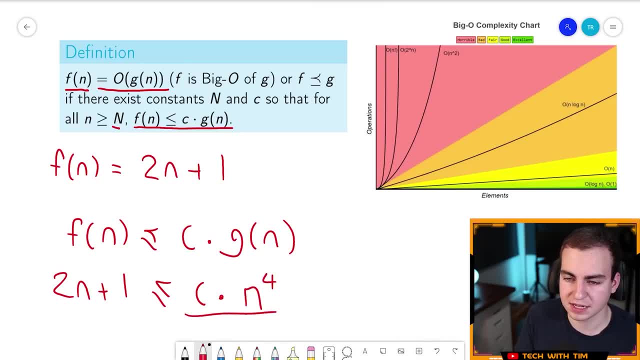 And well, this is going to be true. It doesn't matter what value I pick for C, and doesn't matter what value I pick for uppercase N. This is always going to be true. So I don't want to just pick an arbitrarily large function. 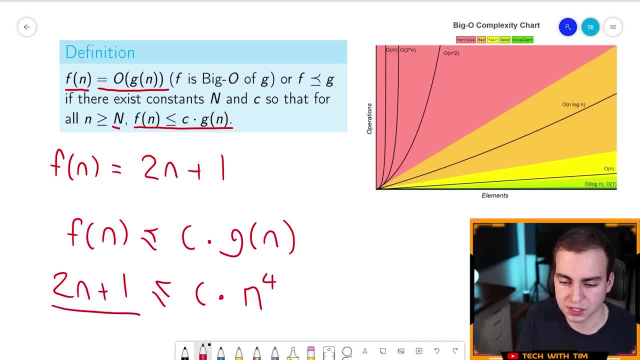 I want to find a function that's as close as possible to this one right here. That's still makes this trip Okay. Uh, again, I know this is confusing. We're going to keep going through it. There's just a lot to get through before you can really even look at an exam. So number of 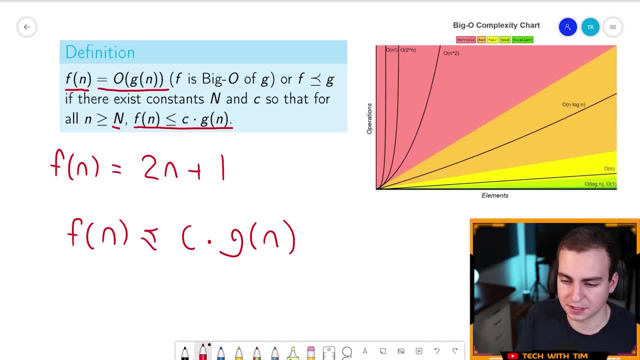 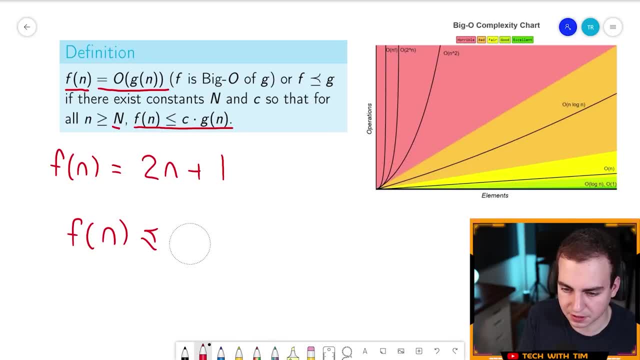 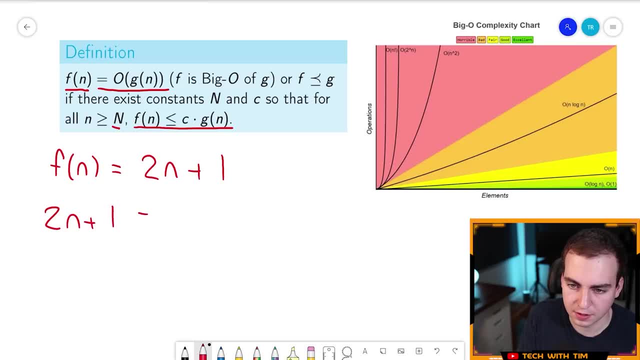 Okay, So let's now write the inequality again: two N plus one less than or equal to C times G of N, And this is four and greater than or equal to uppercase N. So there's three things that we need to find to prove this true. Now what I'm going to do is just randomly pick a function. 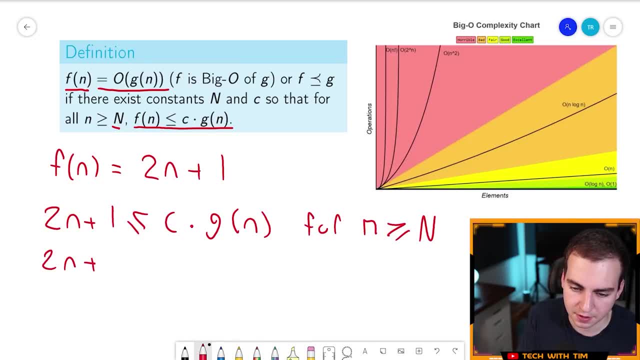 for G of N and show you how this works. So I'm going to say: two N plus one is less than or equal to C times, And then the function I'm going to pick for G of N is simply N. Okay, Just the regular linear function. I'm picking N. So now that we have this, and again, 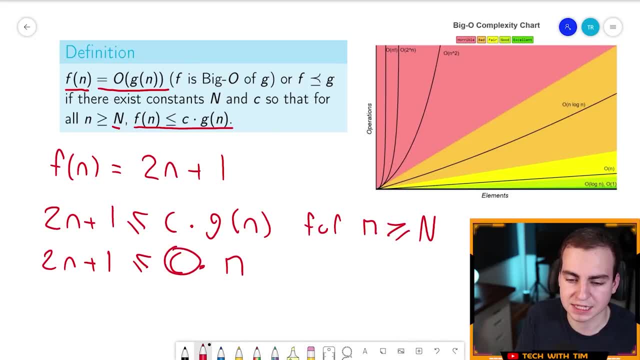 this is going to be for here. I'm not going to rewrite that. We need to find some C that makes this true. And if we find some C that does make it true, as well as some uppercase N, then we know that this is kind of our big O function. That's what I'm going to be calling it. All right, So 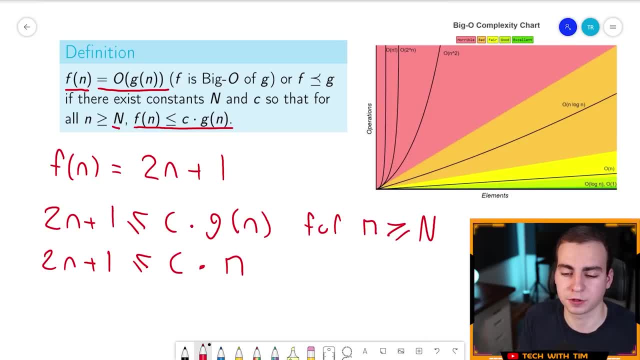 for C. we can find this pretty easily. We can just pick a very large number, right. I can pick a number like 10.. I can pick a number like even three. here That'll make it true. Essentially, Anything other than two or one is going to make this true. And remember: C has a minimum value of 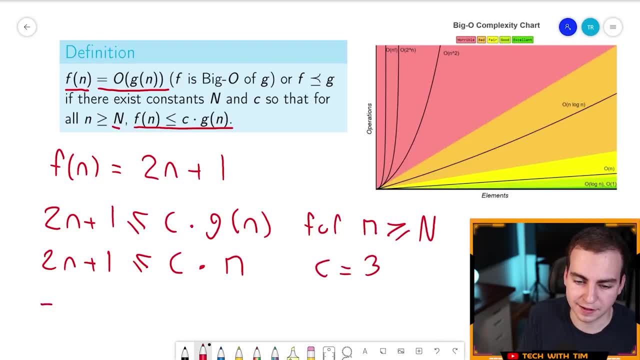 one. So if I pick C equals three, then that gives me the inequality to N. plus one is less than or equal to three N. Okay, great. And then I need to just find some value uppercase N where all N values pass that or equal to it. make this true And really I can actually pick the value one for this. 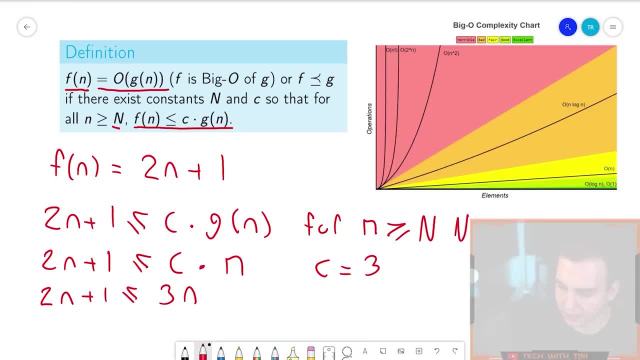 and it will make this true right. So if I pick this, so N is equal to one, then we can just plug in one and we'll see that this is all He's going to be true. So when I plug this in, I get three less than or equal to three. So that's. 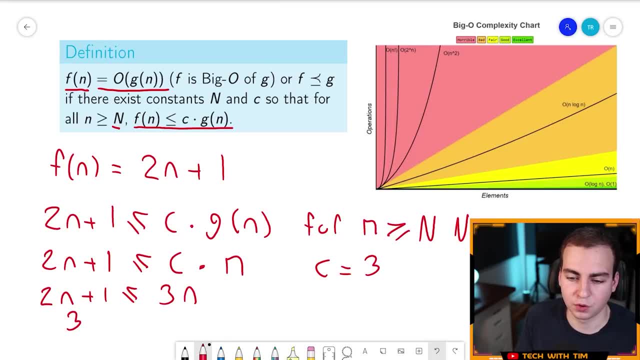 if one is for N and if I were to plug in two, three, four or five, so on and so forth, you're going to see that this side here is always going to be less than or equal to or- sorry, greater than or equal to this. Now, what does that mean? That means that G of N is the big O notation of F. 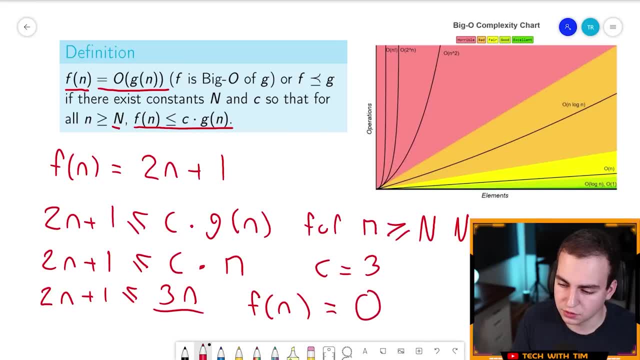 event. So I can say F of N is equal to the big O of N, And that's how you write this. Say F of N is equal to big O of N, or the algorithm has a time complexity of Big O of N. Okay Again, I know this is confusing, but I've just showed you very, very quickly how we 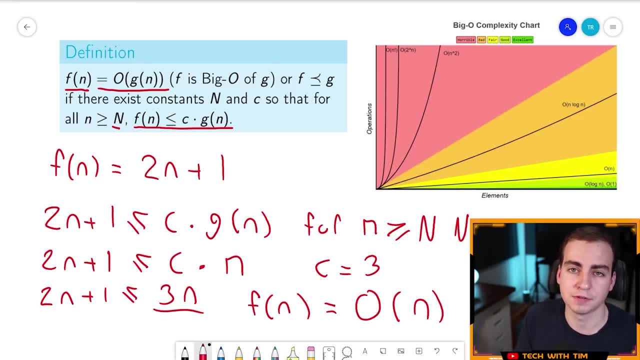 kind of use this mathematical definition to find a G of N. Now, what does G of N really mean? Well, G of N means that, as the input increases, the amount of time that our function takes to execute increases linearly- Okay, Increases on a straight line, as N increases in a linear function way. 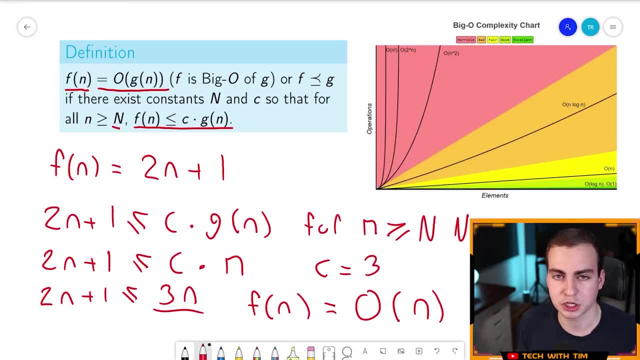 the amount of operations increase. So if N is one, we have one operation. If N is two, we have two operations. It's not telling us the exact number of operations, because we know that's two N plus one. It's telling us relatively what happens to the amount of time it takes for us to execute. 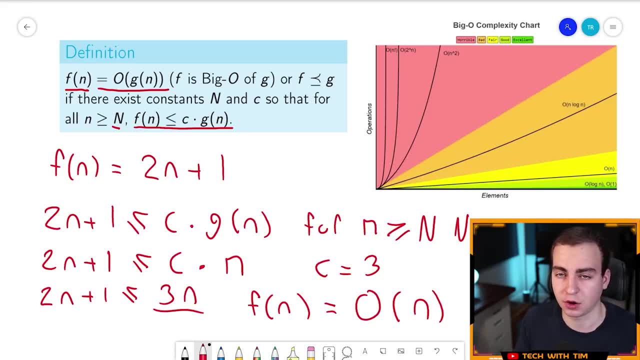 when the input value for the function gets increasingly large. That's the point. Hopefully this is coming across. That's what we're doing with big O of N here. So yes, big O of N is actually less than two N plus one. That's fine. We don't care about the exact number of operations. 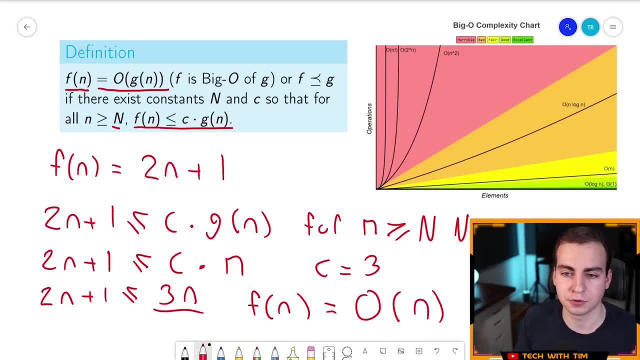 We care what happens to the amount of time it takes when the input increases. And now that we have this function N, we know that it increases linearly the amount of time. So let's clear all of this And let's just go through one more example here and look at some of the big O functions. 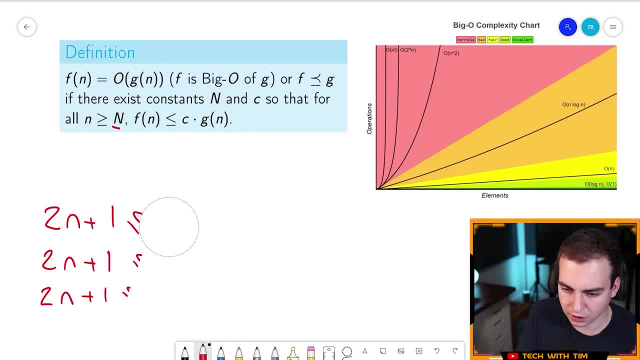 which you can see on kind of the right-hand side of my screen. Okay, So let's say we have a function here that is something like two N squared plus N plus one. Okay, This is the amount of operations that it takes. We'll say that this is F of N. should have wrote it in the other way, but that's. 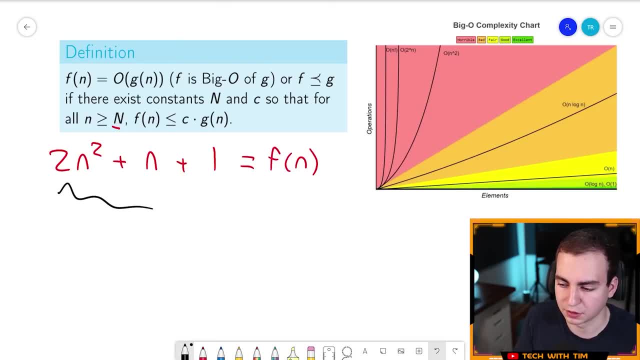 fine, And I'm going to write the rest of this in black here. Uh, just so you're aware. Okay, So now find a G of N for this. So what do we do? Well, we're going to write this out to N squared plus N. 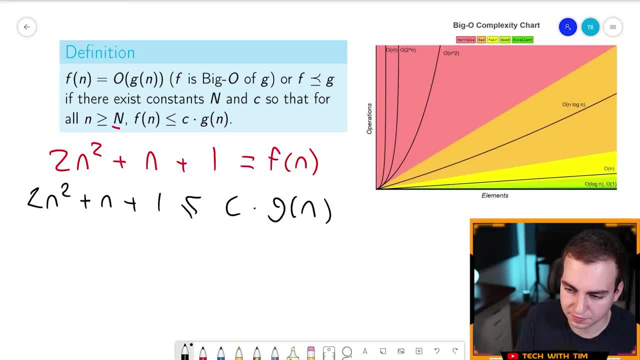 plus one is less than or equal to C times. G of N for N greater than or equal to N. Okay, So now let's pick something for or pick something for G events. right, So two N squared plus N plus one less than or equal to C times. What if we pick N now? if we pick N immediately, we're going to. 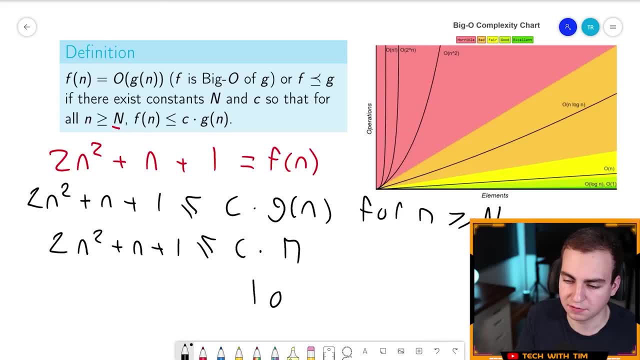 see here that it doesn't actually matter what constant we give. Even if we give a constant like a thousand, when I start passing really, really large values for N, N squared is going to exceed C times N very quickly, right? So if I pass even a huge value for N, uh, like you know, 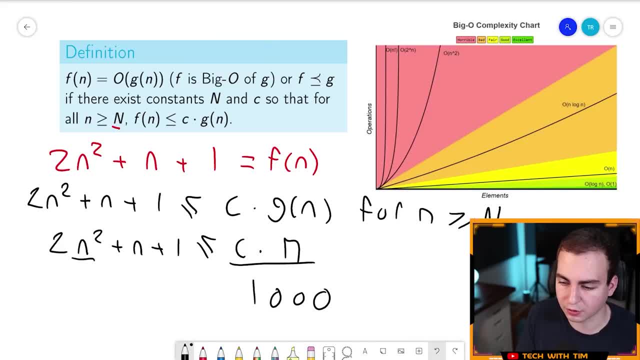 a thousand, 10,000, you're going to see that this side here is going to be a lot greater than this side here, even though I'm multiplying it by a thousand. Now, that's not something you're necessarily going to prove, but you just need to be able to look at that and kind of figure that out. when I 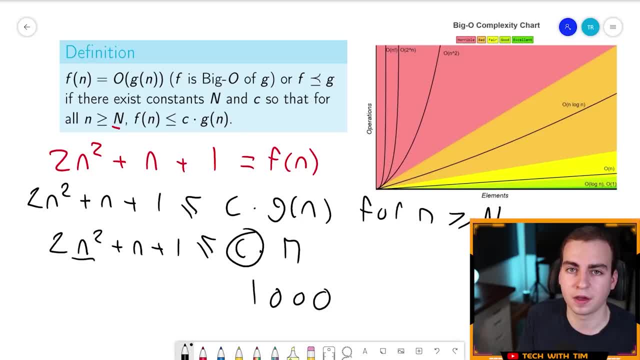 have an N squared and I have an N over here. doesn't matter what the constant is. This is always going to outgrow this side Eventually when we get to a very large number of N. so that tells me that I cannot find some C and I cannot. 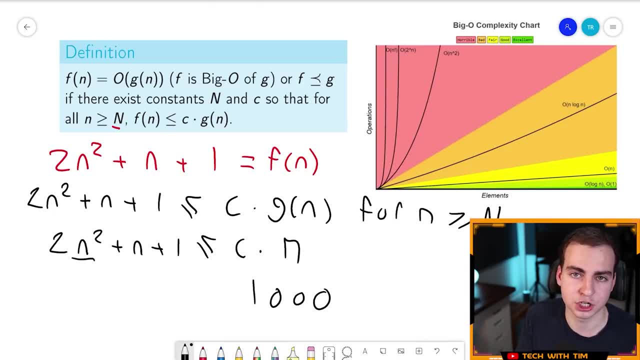 find some N, And so N is not going to be a valid function for G of N. So now, instead, let's try N squared. So now, if I have N squared, I'm actually going to be able to prove that I can find some. 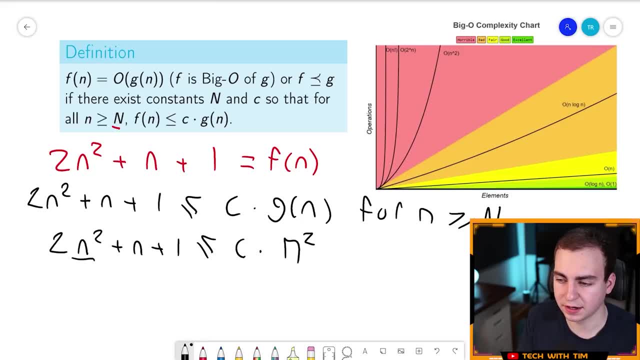 constant C. So to prove this again, I just need to find some C and I need to find some N. So let's look for a number for C. let's just pick a thousand, Okay, So if I say C is equal to a thousand, 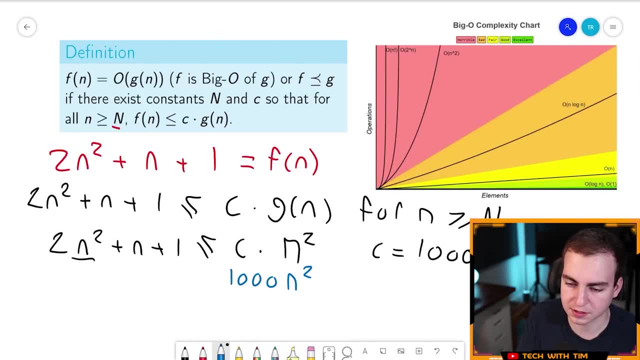 now we can plug this in. So we're going to say a thousand N squared- And I don't know why I'm writing these in different colors- but I just am going to say two N squared plus N plus one. Now it actually doesn't really matter what value I pick for. 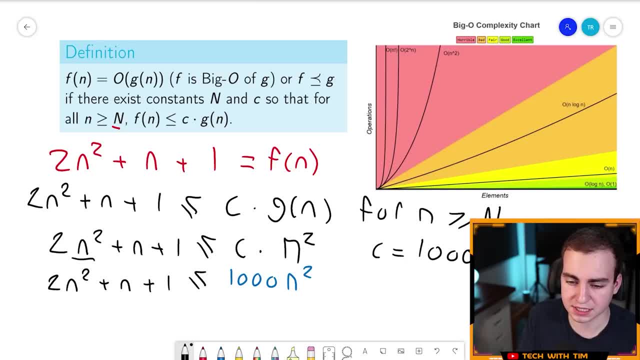 uppercase N here. In fact, I can pick any value and you're going to see that we get the correct inequality here. Okay, Because I picked a large enough number for C. now you can make a smaller number of C. It doesn't matter what number you're picking, You're just picking. 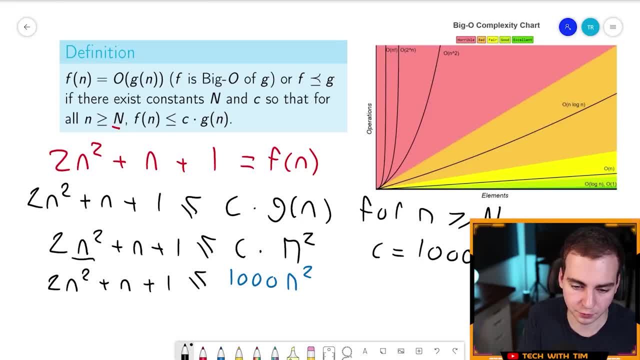 that to prove that this inequality is true. So, for example, if we plug in, say, one right, we have two, one plus one plus one. That's going to give us four. And then this right is going to give us a thousand. So this is larger. If we pick two, this is going to give us 4,000.. This is going to be a. 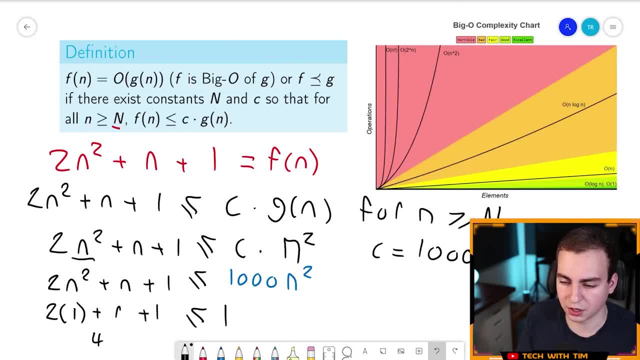 much smaller number. So you're going to see that this side is going to be greater. So there we go. We now know that the function here is going to be N squared. So what we can do is we can write: F of N is equal to big O of N squared. Now you might start be starting to realize a pattern here. 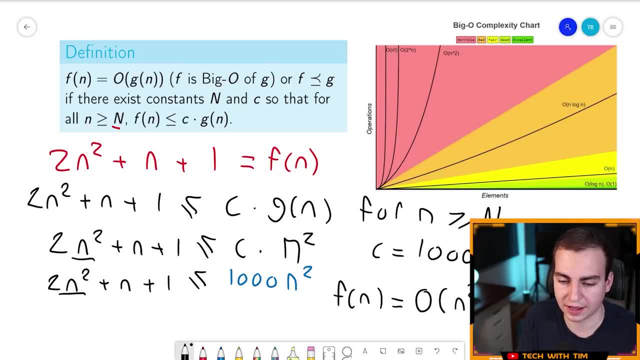 And the pattern is: you can essentially look at the largest term when you have things being multiplied together and understand that that is going to be what the big O function is. Now there's a few tricks and I have to go through a bunch of them. 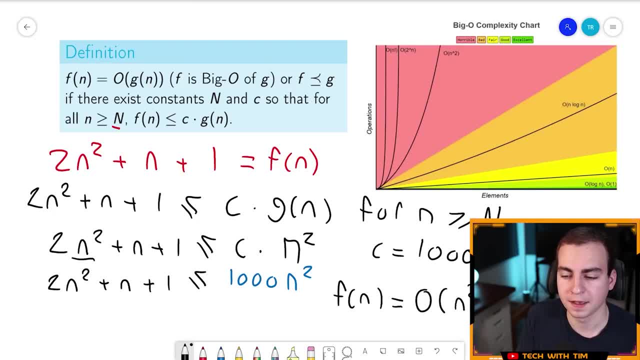 but the point is here: when we have something like two N squared plus N plus one, if my uh function G of N is simply N squared, I'm going to be able to find a large enough constant that it doesn't matter what the other terms are here. It's always going to be greater than this. 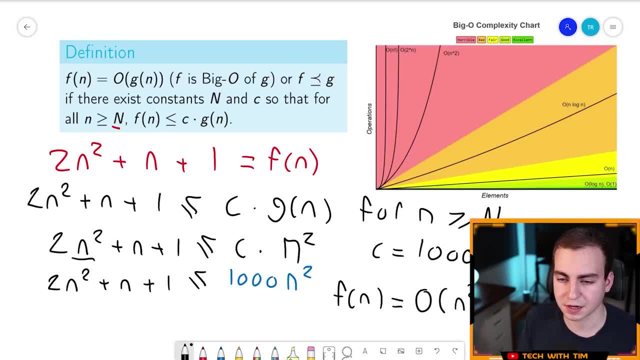 So let me just stop here for one second, go through this example again and make sure it's clear, Cause I get this is confusing And this is something that you have to look at a bunch of times for really starts to actually make any sense. So I have two N squared. 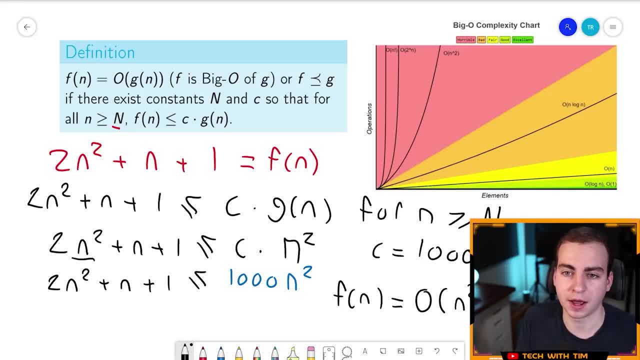 plus N plus one, That's the number of operations that my algorithm takes. Now I'm trying to find a simplified function that is going to give me a general concept of what happens to the amount of time or the amount of operations required from this algorithm as the input grows. very 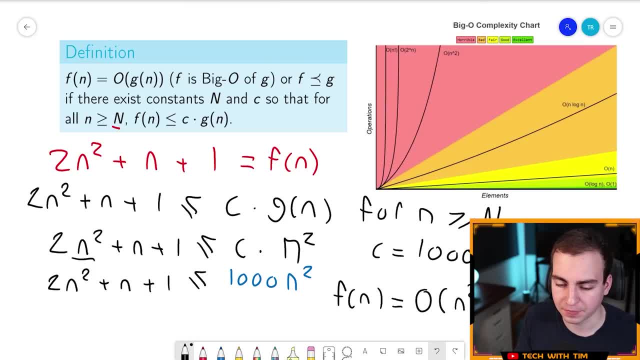 very, very large. So again, we're thinking of really large values of N. So when the values of N grow really large, what's going to happen is this term right here is going to be dictating the number of operations that are occurring. 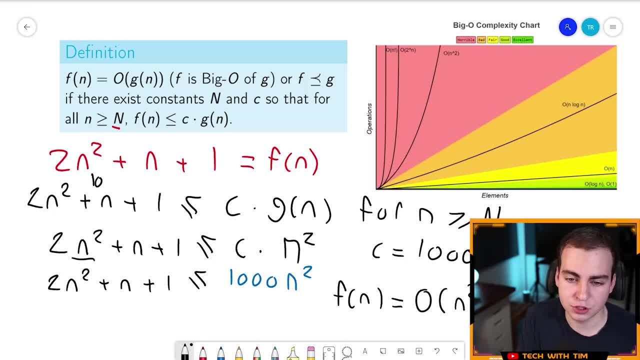 If you pick a value, even something simple like 10, right, The two times N squared gives you 200, the N gives you 10 and the one gives you one. So these become increasingly less important. The N plus one as N squared gets larger and larger, And the same thing happens with this. 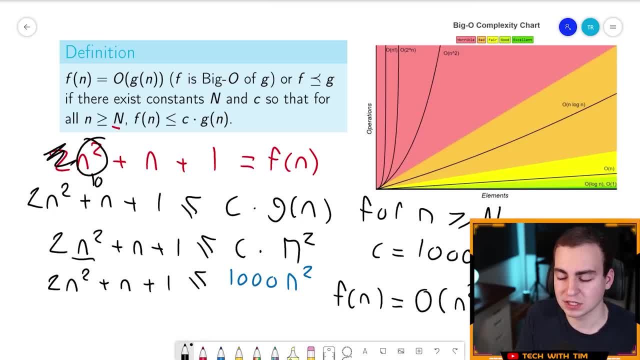 two here. this becomes increasingly less important as N squared gets larger and larger and larger. right That, that's really the point here. as N gets larger, all of the N squared gets larger Of the constants that we have here, and one and two are going to become less important. Now the N 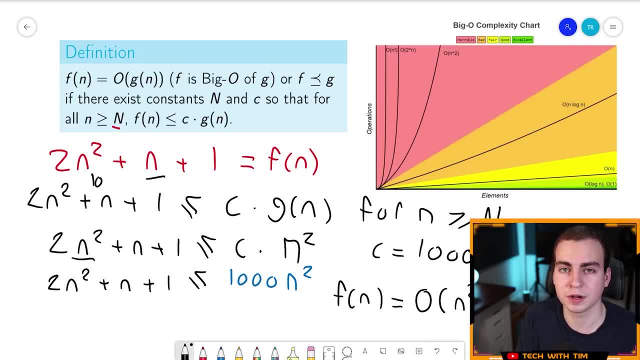 is not a constant, I know, but it still becomes less important because N squared is much, much larger than N. That's what we're looking at. So what we do is we get the bigger notation of N squared, because this is the term that most accurately represents what happens to the amount. 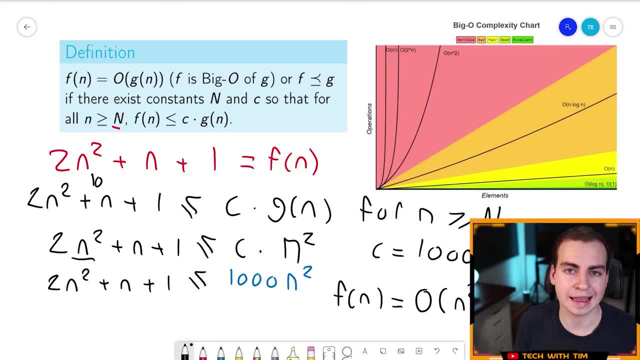 of output or, I guess, the time to execute our function as the input increases. And again, the way we did that is we're using the math. here to prove this, I'm going to show you a bunch of shortcuts. You don't have to do this math every time, but it's important just to see kind of how this works. 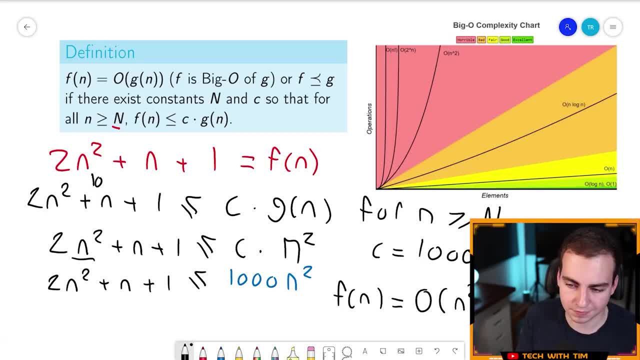 So you understand the math that goes behind this and how you prove- uh, you know- that your bigger notation is actually correct. Okay, So now let's just look at a few more functions, and we're going to do them in a really fast way, And I'm going to show you a few shortcuts that are going to 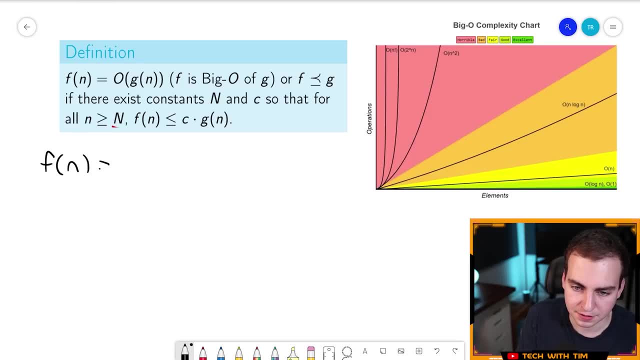 make this seem really easy. So let's say we have F of N is equal to three, and let's go with N cubed plus and squared plus. And then we're going to go: uh oops, let's go ahead, This log base, two of N. Okay, So notice, these are all pluses, right? So I have three N squared. 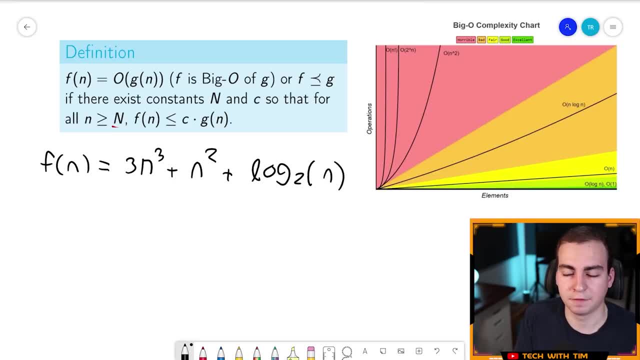 plus N squared plus log base two of N. Now a few shortcuts that you can keep in mind. here is: whenever you have uh terms that are being added together, So additive terms, you can essentially cross out and remove every single term and constant. That is not the largest term that you. 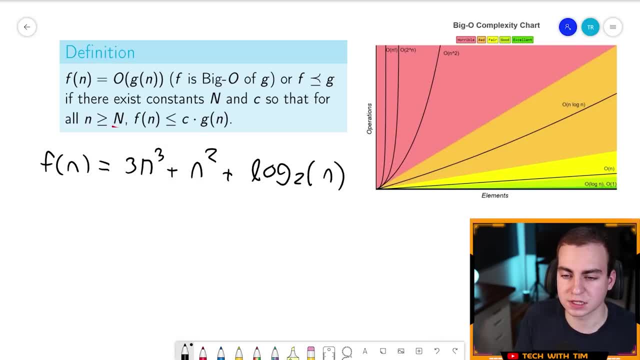 have in the expression. So again, the reason that you can do this is because, as N increases and reaches infinity, cubed is going to dictate the amount of operations that this is going to take. Let's just plug in a value and have a look at it, Right, All right, So let's just plug in 10 here. 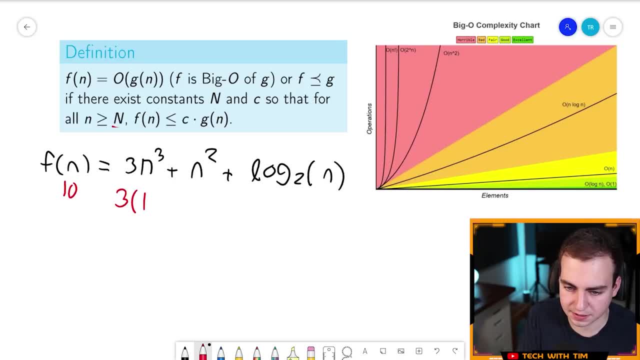 and see what we get. So we're going to have, I guess, three times a thousand plus this is going to be a hundred plus approximately 6.6.. So if we look at this, we're going to see these terms right. Even the three become increasingly less important as N gets large and then isn't even 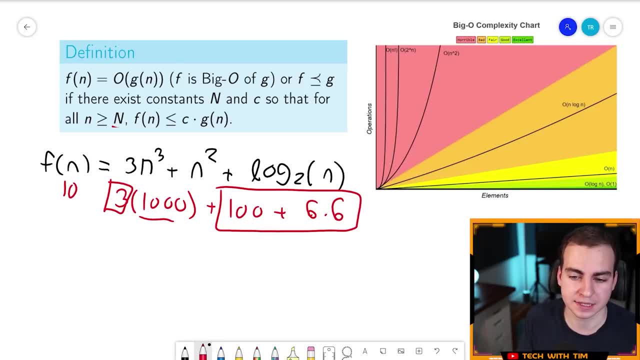 that large And it's 10.. Imagine what happens now when N is 10,000, 10 million. the N cubed really carries the number of operations, And so we don't care about these ones right here And we can cross them off when it comes to our big O notation. Now to be able to actually cross, 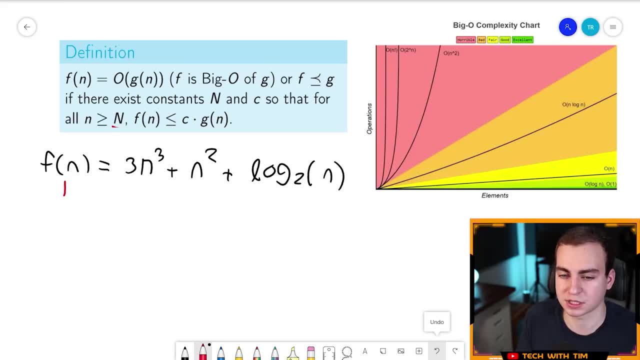 these off. you can do a bit of math to kind of prove that you can cross them off. So what I'm going to say here is: let's assume that N squared and log base two of N is equal to N cube. So the reason I can assume that is because N cubed is greater than N squared. Let's assume that N. 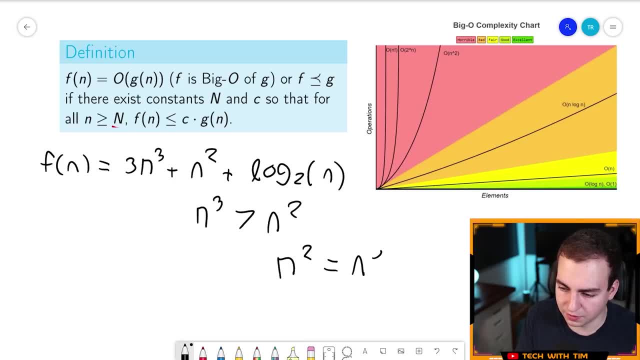 squared is equal to N cubed. Now I know this is Is Not sound math, but just assume the N squared is equal to N cubed. If it is, then what I can do is change all my N squared terms to N cubed. So if I change N squared here to N cubed, which is larger, 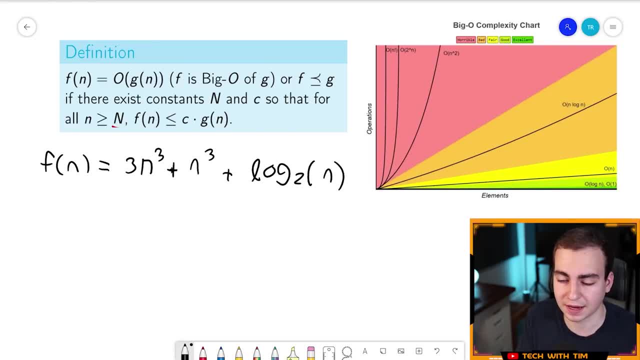 than it. So it's valid for me to do that because I'm adding something in that's larger than N squared. And then I changed my log base two of N to the same thing and cubed. What you see here is we end up. now, if we factor this, we get five and cubed. Now again, the five is a constant. We. 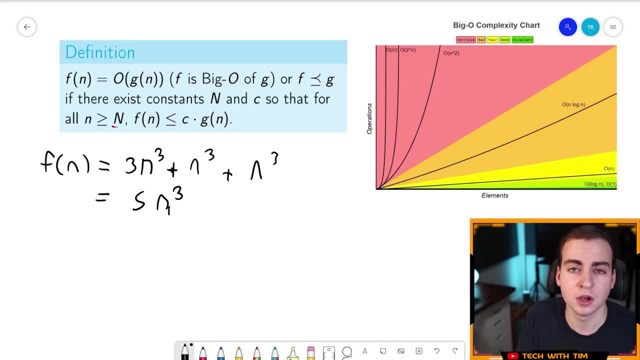 don't care about the constant, because we don't need to know the exact number of operations. We just Want to have the function that tells us what happens as the input gets larger. So N cubed is that function. So we simply strip off the five and we say that the bigger notation here is N. 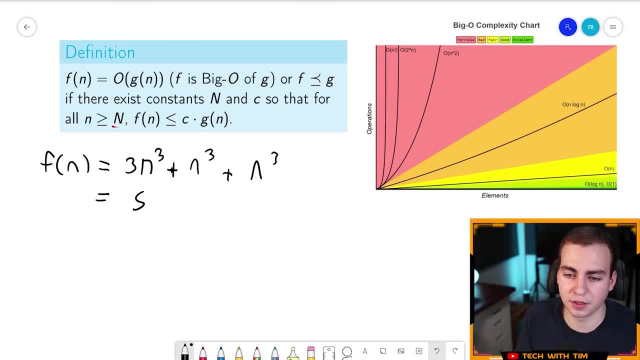 cubed. That's the way that we do this. So if you take every single other term that you're adding- it's very important that you realize we're adding these terms here- and you say, okay, well, if it's smaller than N cubed, let's assume it's N cubed. Now, if we add all of these together, 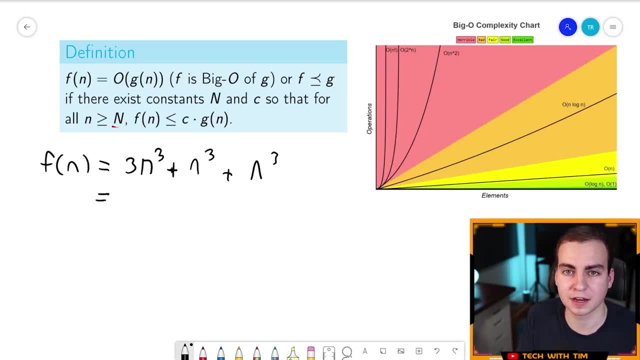 I not factor, So I said fact, for if you add all of them together we get five N cubed. We know we don't care about the constants, because we're just looking for a function And to give us, uh, the relative amount of operations. then what we can do is cross off. 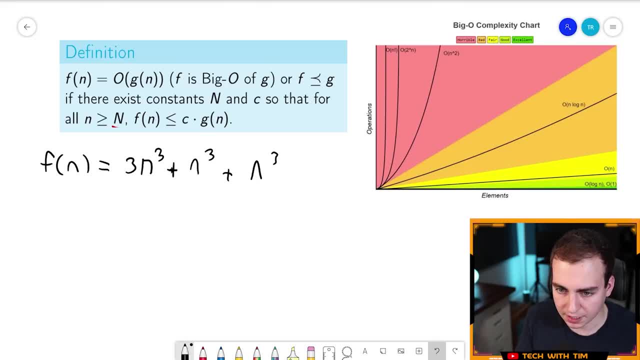 the constant, which would have been five, and we're left with N cubed. Okay, So that's one example. Let's now look at another example that has to do with, uh, multiplying terms. So let's now say we have something like three N and we're going to multiply this by the log base, two of, and then 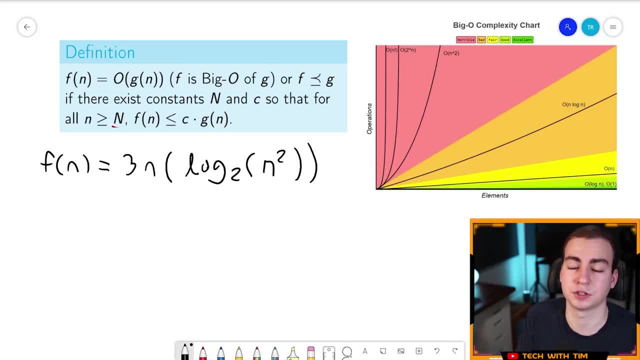 this'll be N squared. Okay, So this is actually what we have. Now, what we want to do is simplify this and find G events. We can find the big O notation. So for this function here, the first thing that we know we can do is remove the constants. Again, we can remove them because 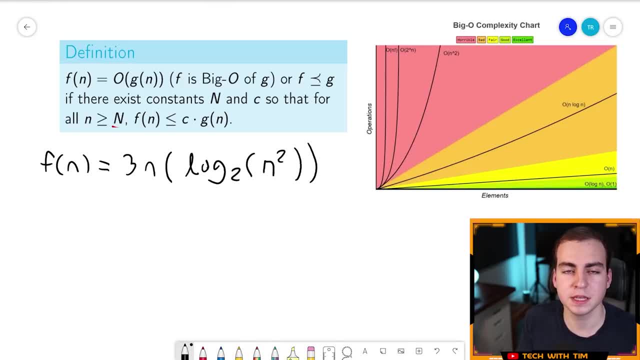 we don't care about constant values, We only care about a function based on the input that tells us what happens to the number of operations or the expected kind of running time of the algorithm based on the size of the input. So we can remove the constant. So we remove the constant three. 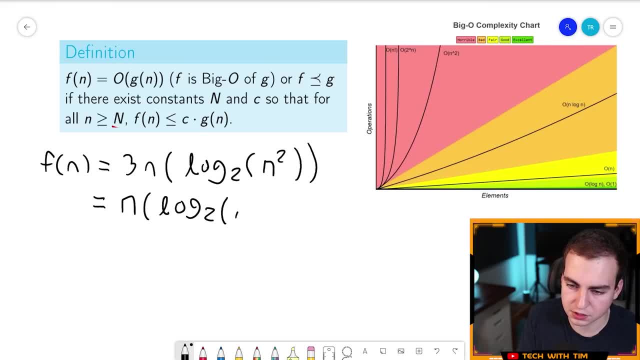 and that leaves us with N multiplied by log base, two of N squared. Okay, Now we don't really know how to handle this N squared inside of here, And I'm going to show you how we can simplify this even more. You could technically say that this is the big O notation. right now We can get even simpler. 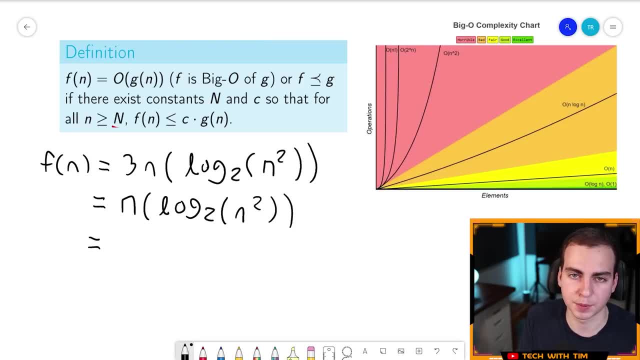 We can take this two out based on using exponent rules, and I'm not going to drive these rules for you. I assume most of you probably know this already, At least if you're in high school. let me write log properly. Uh, we're going to be able to take the two out right before the log. 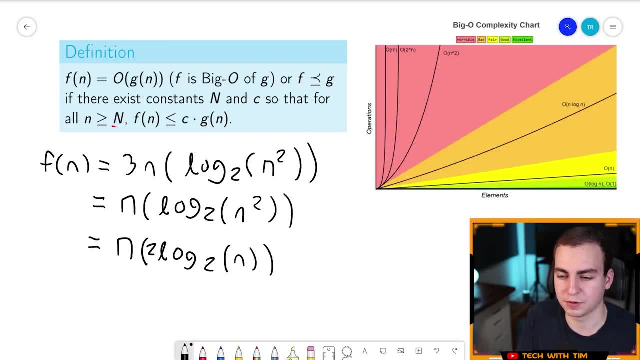 And then we can put this here Now again. the reason we can take the two out is because whenever we have something to the exponent inside of a logarithm, that exponent we can simply put as a multiplication to whatever the logarithm is. 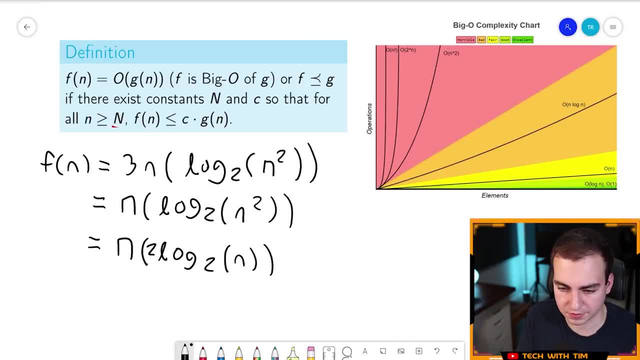 Of the base of that number. Uh, and so that's what I'm doing. So I'm saying to log base two of N. I can take the two out. Now, the two is what a constant. We don't care about the constant. 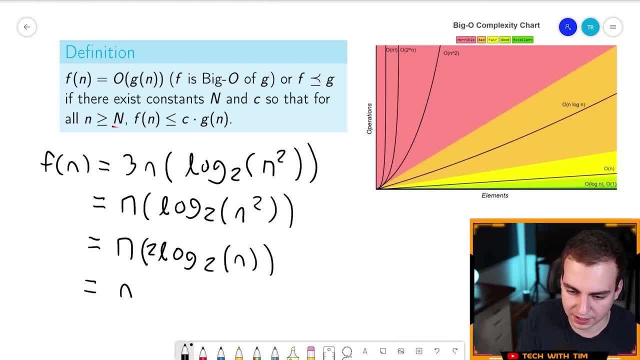 so I can remove the constant. Okay, So now, if we continue, I get N and then I have log base two of N. Now can I simplify this anymore? No, I cannot. I cannot simplify because we are multiplying these terms, not adding them. If we were adding the terms together, 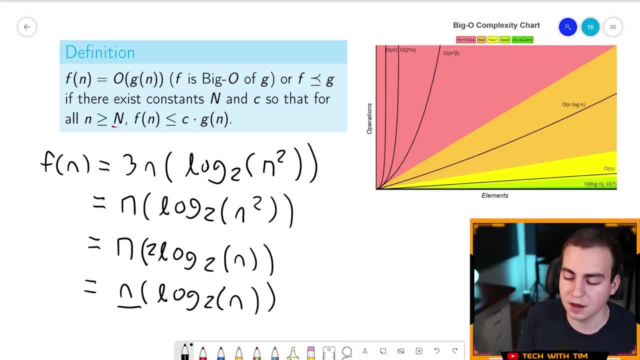 I could remove the log base two of N because it's smaller than N, but I cannot in any way here find a way to actually write this as a constant multiply by N, like previously. if I had N plus and then I had log base two of N, I can say that since log base two of N is smaller than N, 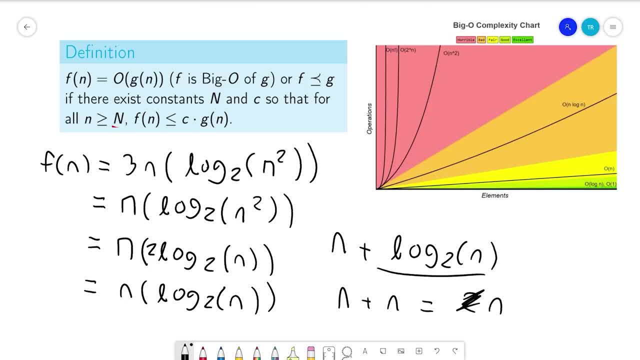 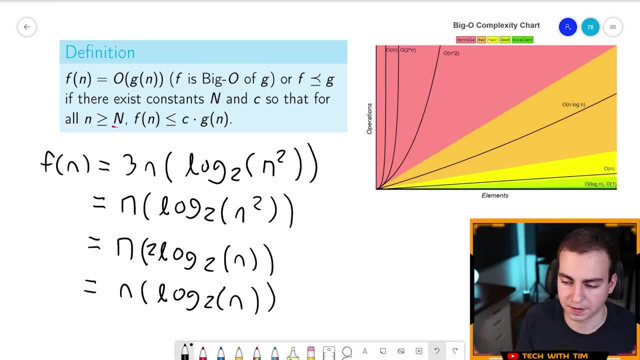 I can write this as N plus N. that gives me two N, and then I can cross out two. but here, since we're multiplying the terms together, I don't have a way to do that, And so I can't simply remove the log base two. Okay, If you wanted the math version of that. that's why it also makes sense here. 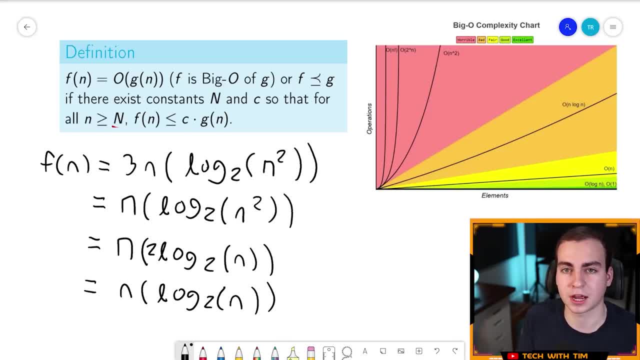 Since we have two factors being multiplied, they both really affect how much time this is taking. So we need to keep N log base two of N around. Okay, Now that we've looked at that, let's just have a look at what's on the right-hand side of my screen And then let's get into some. 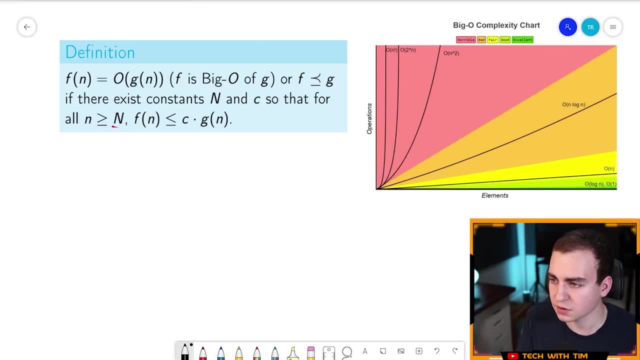 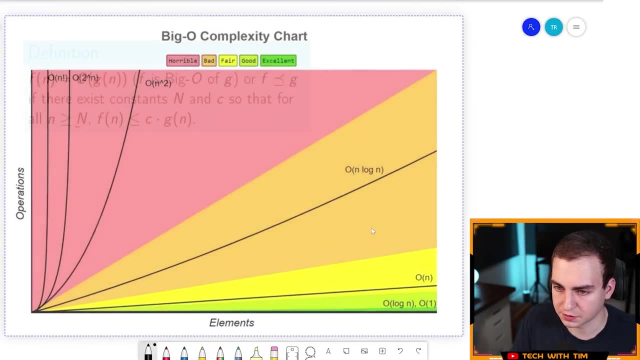 some examples, Cause I'm sure a lot of you are tired of this map. So on the right-hand side of my screen here we have the big O complexity chart. Now let's just see if we can make this bigger so that we can take up the full screen with it. Nice, Okay, So this is the chart Now. 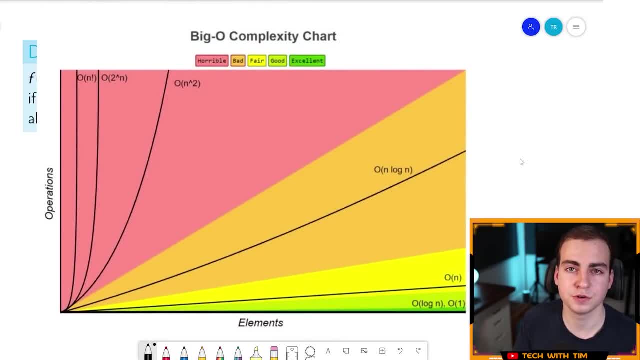 it actually is pretty good. I don't really need to explain it too much, but it simply shows you the big O functions, in which ones are better than each other, because once you find the bigger notation, that's great, but you need to know which functions are better than other functions. 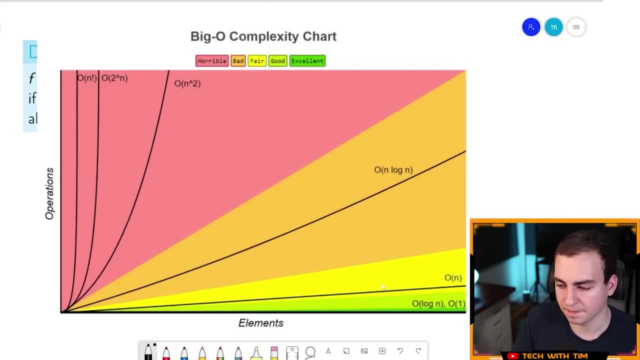 in terms of their complex. Now we've already looked at log of N. log event is great. That means that essentially, as the input increases, the number of operations we need to do is on a logarithmic basic basis, which means it's getting smaller and smaller When log is equal to a hundred. 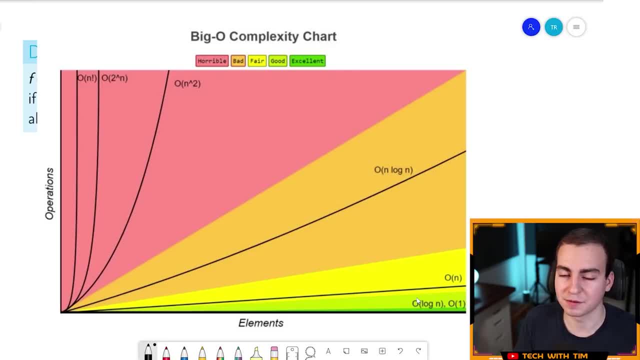 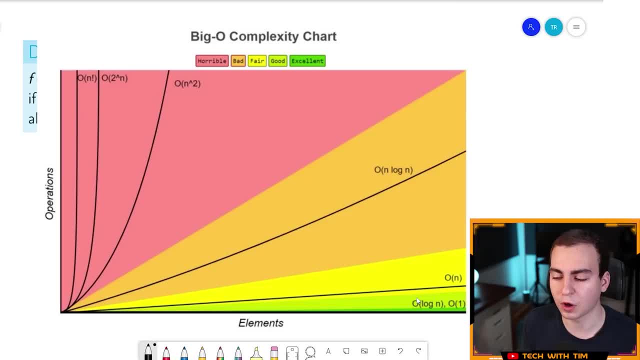 You get the point: as we get to a really, really large number, it stays really small. when we have a logarithmic, uh time complex, then we have a constant time complexity, Oh of one. This means that there's actually nothing based on the input. This would be like printing a number or uh you. 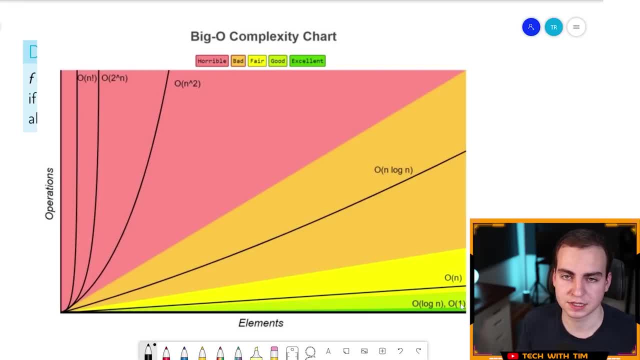 know, checking if a number is odd or even performing a modulus. This is a constant time operation. This isn't something that requires the input, So if it doesn't matter to the input at all, it only ever takes a hundred steps or 50 steps or a thousand steps- a constant number of steps. 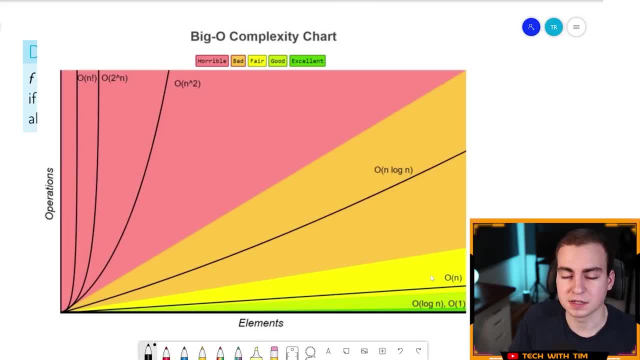 Then we have a one, a constant time. Oh, and this is linear. This is a fair or good time complexity. If you have a linear time complexity, usually that's pretty good. It means your algorithms times scales with the input, So as the input increases, the amount of operations- uh, increase. 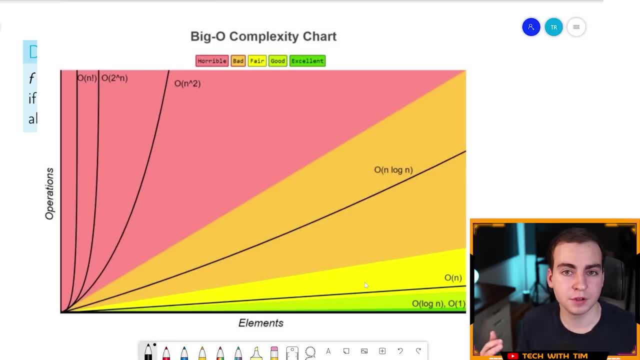 relatively at the same amount. If we have 10 inputs, we have, you know about, 10 operations. If we have a 20 operation or 20 inputs, we have 20 operations. Now it might actually be a hundred operations or 200 operations, but that's fine because it's happening linearly, not 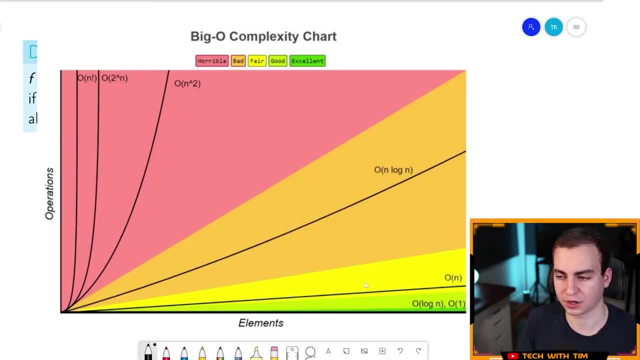 exponentially, uh, or any of the other complexities that we're going to look at. Okay, Continuing with N log N now. N log N is kind of a middle ground. here, As you can see, we're multiplying a linear time complexity by logarithmic. So it's not horrible. It's not as bad as something like: 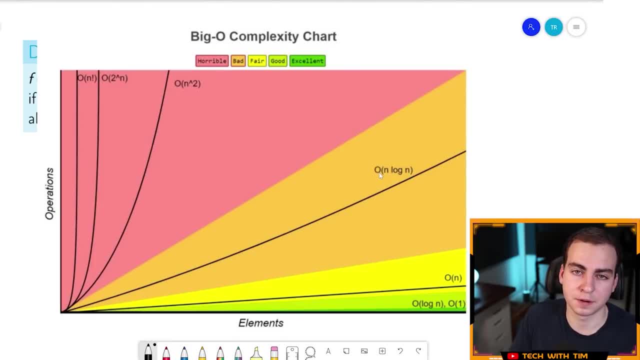 N squared but it is, you know, fair. It's going to take a long period of time If we have a lot of inputs. again, all of these are time estimates used to be compared against each other. We're not looking at an exact amount of operations or exact amount of time. So N log, N fair, time complexity. 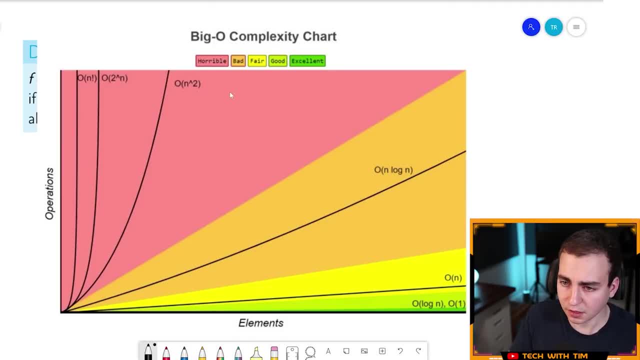 it is bad, Better or sorry, worse than a big O of N. Okay, Now we have N squared and squared is a horrible time. complexity: That means that we increase the number of operations we need to do exponentially as an increases- And I'm sure many of you have looked at exponents before- not very good when. 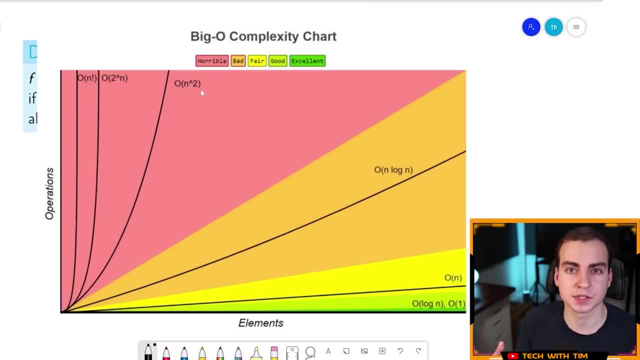 N gets to a large number. Say we had 10, we have N squared, that gives us a hundred already keeps getting larger and larger and larger. Then we have something like two to the exponent N. Now this is even worse. This is a very, very poor time, complexity, As you can see. and then we have 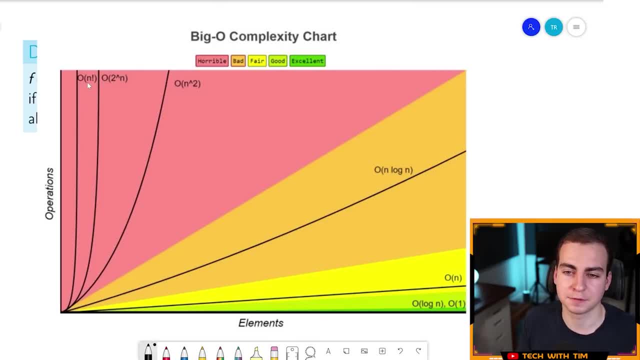 something like N factorial And we have even more complex time complexities where we have something like N factorial multiplied by two N plus M and would be another input. I'll talk about that later, but this is the general graph, So you kind of need to memorize this graph. It's pretty easy, You could just plug in some. 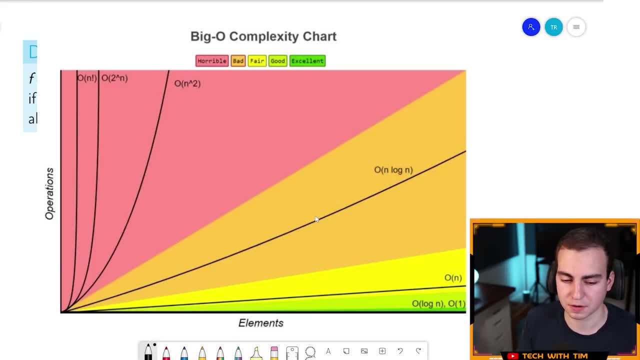 values and actually see which ones are getting larger faster, if you were unsure, but these are the most important big O functions And we're going to be using combinations of these functions when we're analyzing the time complexity of the examples I'm about to go through, So I apologize. 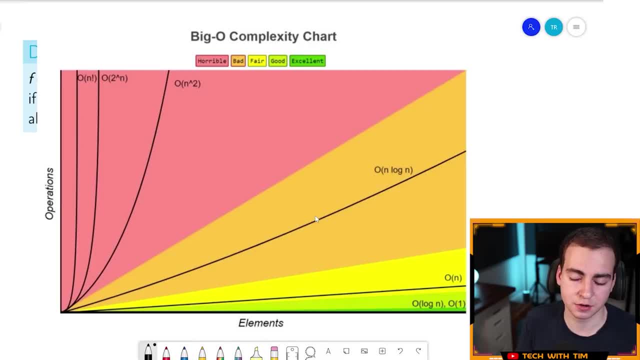 I know this was long, but I just wanted to try to explain this as best as I could. Hopefully that made sense. Now we're going to go through 12 examples and I'm going to walk you through exactly how we solve them. All right, So. 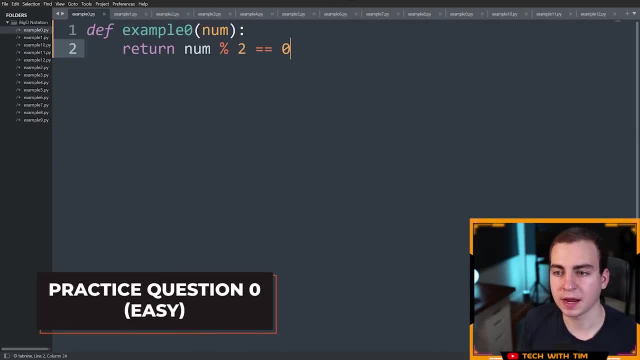 we're moving on to the first example here, example zero. I'm going to ask you right now: what is the time, complexity or big O notation of this function? Think about it. pause the video If you need to. I'm about to go in and explain. So the answer here is that this is constant time. Okay, Now I'll. 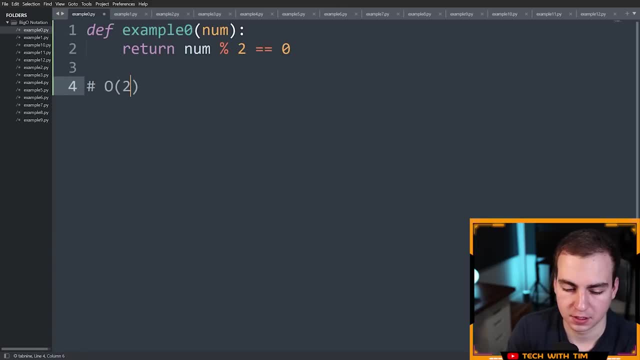 explain why it's constant time, but this is a big O of one. So inside of here, what we're doing is we're performing a constant number of operations. It does not matter what numb is, and numb is going to be N right. Numb is N cause that's our input. So whatever the size of 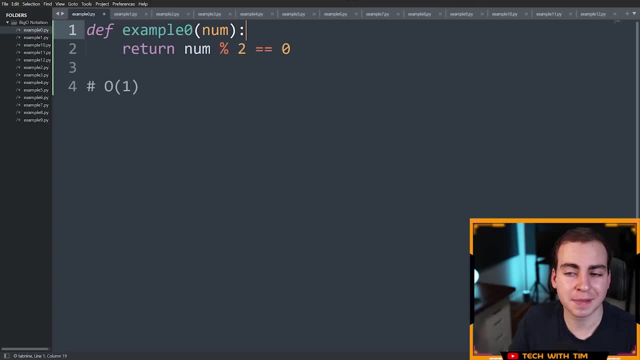 numb is. we represent that with the variable N, and it doesn't matter what this is. It's always going to take us approximately the same amount of time to perform this calculation right: The modulus of two or the numb modulus two, And we're just checking if this number is odd or even that's what. 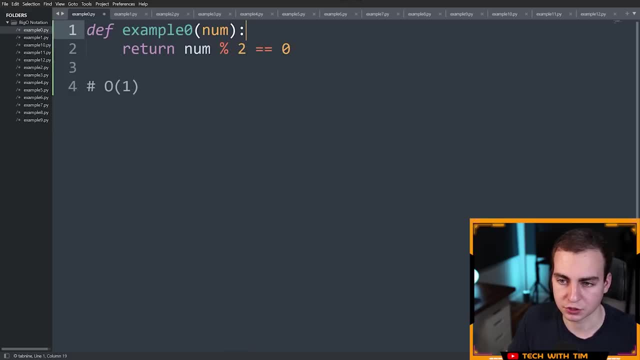 we're doing here. So this is a constant time operation, fairly straightforward. Now I want to mention that If I did something like X equals one, Y equals three, whatever, this is still a constant time operation. I don't write something like O of three, I just keep it at Oh one, which means we're going. 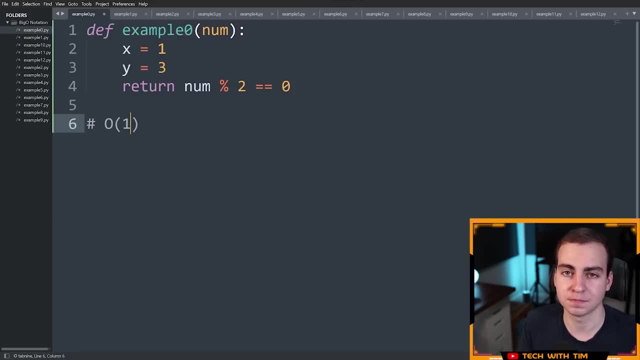 to do the same amount of steps, no matter what N is, no matter what the size of our input is. And as we go through these next examples, you're going to see that I've labeled inputs, different values, uh, you know- numbers, strings, whatever. you still want to represent them using N and is. 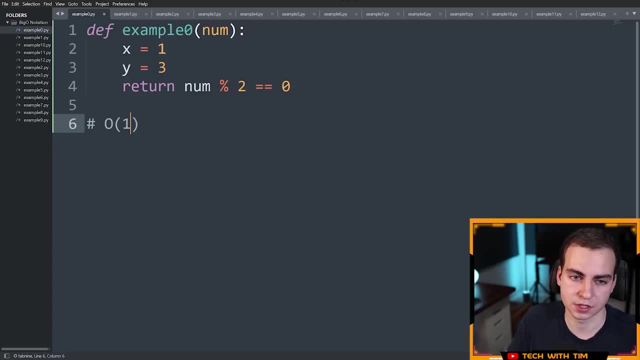 the length of your input or the size of your input in every single situation. Okay, So I'm going to go to example one. example one. we've seen this example kind of already. I have total equals zero or number in nums. total plus equals number. return total pause video. What is the big O notation of? 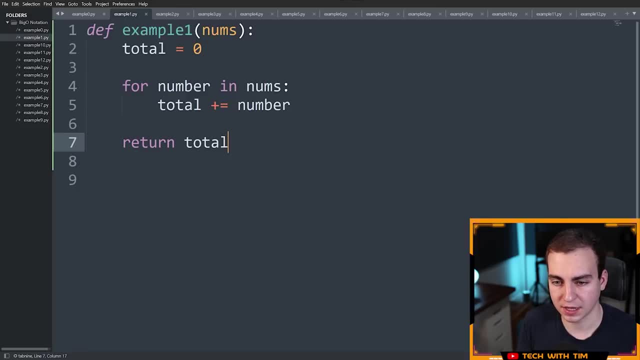 this example or of this algorithm right here. Okay, So the answer, as I'm sure many of you have gotten, and probably fairly quickly, is big O of N. now, N is representing the number of numbers that we have in nums, So the size of our input. 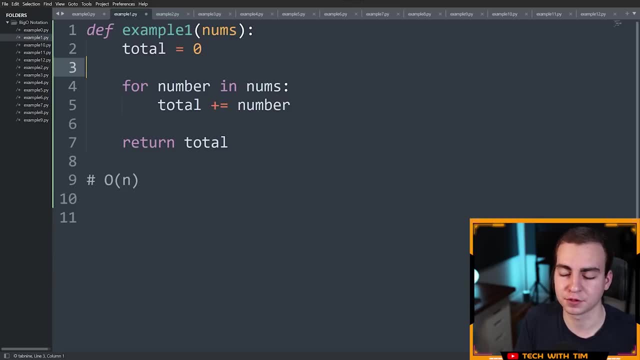 Now what we do here to calculate. this is exactly what we did in that first example that I showed you. We have a variable. This takes one, one operation right. We have a four loop. This is going to take N it. 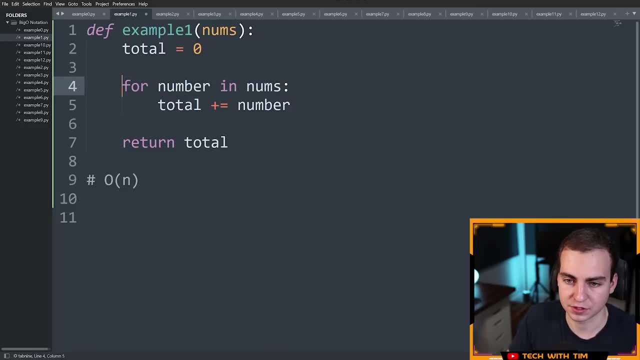 takes N, because the number of numbers is N, right? So this four loop runs N times. we're doing one operation. So what we ended up getting here at the end- you could count this as an operation, If you want as well- is something like N plus one or N plus two, whatever you want to write, Okay. 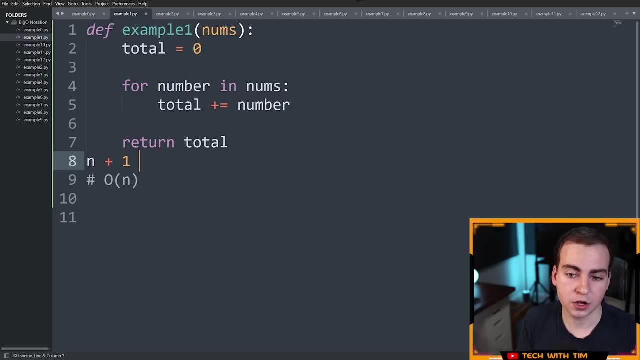 So we'll say it's N plus one. If we have N plus one, we know that we can simply remove the constants, which are one, because as N gets larger they're not going to matter, and write the big O notation as big O of N. Okay, So that's that example, Let's move forward. Okay, Now this one is: 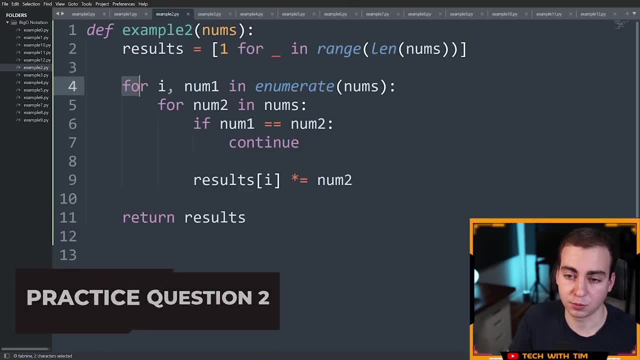 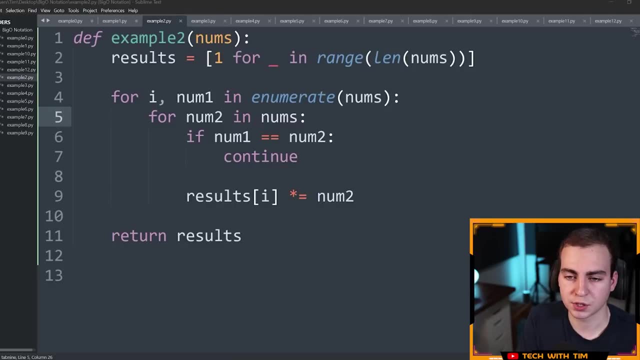 getting a bit more complicated. Now we have an example where we have a nested for loop. So again, pause the video, go ahead and read this, And it's going to get even more complicated as we go on. All right, So let's go line by line. We have results here and results. We're creating a list. 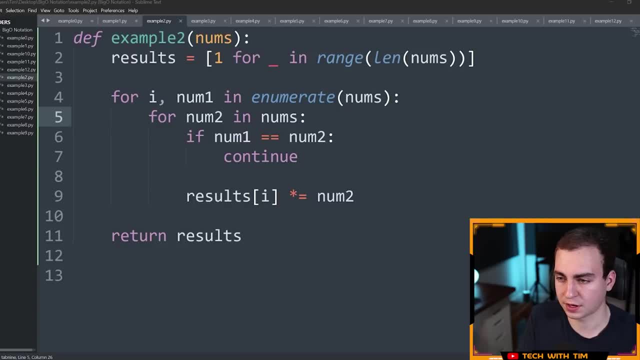 Now this list. we have a four loop here. We've got to look at all of our loops, Okay, And any operation that could be Looping, And what happens is we need to four N, right, So four underscore in range. 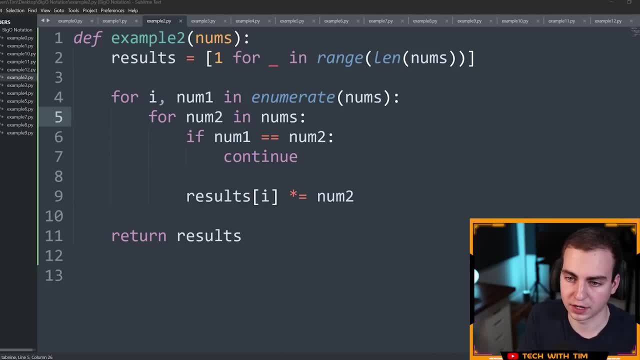 Len of nums. Len of nums really is just N or adding one into the list. So this is going to take us N to do because we're adding one N times. pretty straightforward. Move on to the next loop. Okay, Inside of this next loop. Well, how many times does it take for this loop to run? 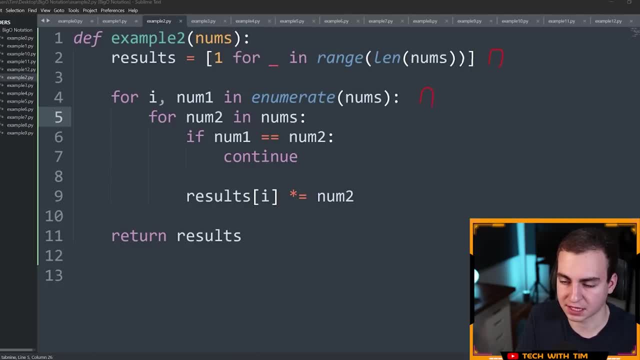 This loop is going to take N times to run because we're doing it for the size of our input, which is N. Okay, Now we have another four loop inside of this four loop. Now that means that this four loop needs to run How many times- N times- and how long does it take for the four loop? 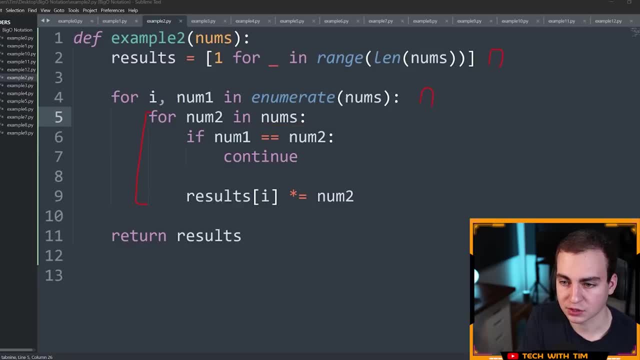 to run. Well, this four loop is looping through nums as well, And so that gives us N Okay. So we have N stuff happening N times because that's four loop is happening. Now inside of here we can count the operations. We can say: this is an operation, This is an operation And this is. 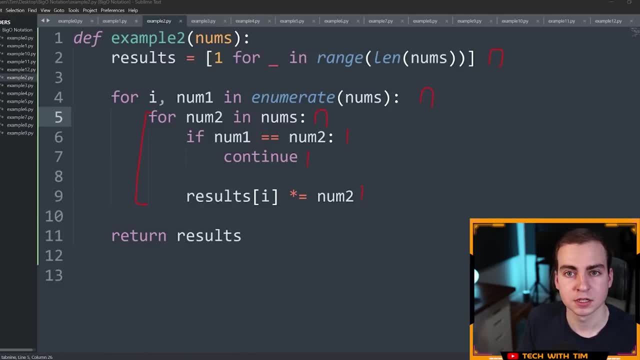 an operation. Now, remember, we're considering the worst case. So in one case, when num one is equal to num two, we're not going to perform this operation. We're going to perform this operation. However, we don't really care about that. We're not going to factor that into our calculations. 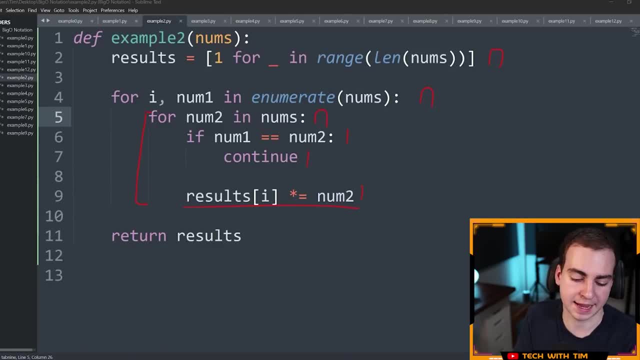 here because this could happen. right, It's happening every time except once, So we're just going to assume that this operation happens. the end times for this four. Hopefully you get what I'm saying, but I'm just trying to get through like don't overcomplicate analyzing. 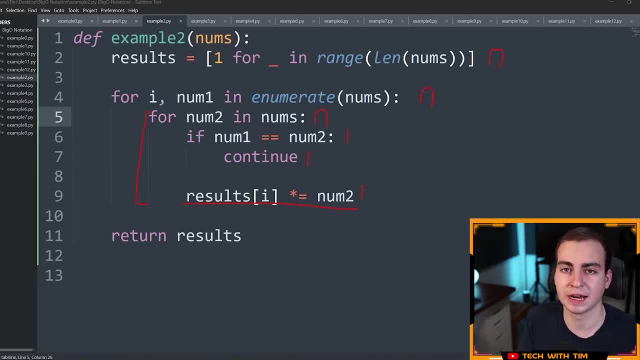 the number of operations. here We're just trying to get a rough estimate and then we can actually figure out what the bigger notation is. Okay, So we have about three operations at most. We have to perform a condition. We're going to continue. 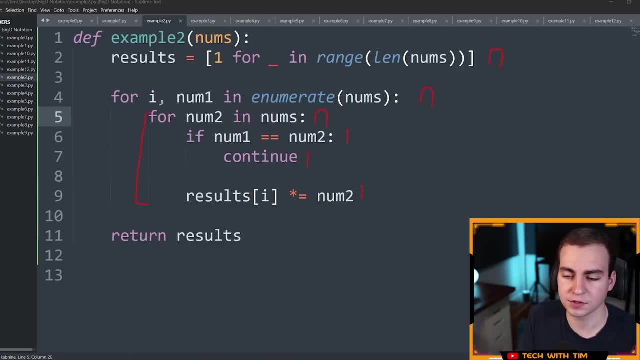 We could count that as an operation. We're going to do a multiplication. We'll just sum all of those up, even though they're not all going to happen together. Okay, So we say approximately we're going to get three operations inside of here. Then we're returning results. Okay, That's. 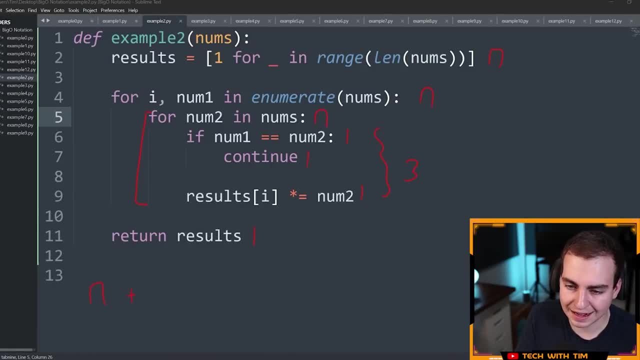 another operation. So we have N. now we're adding that because this is not inside the four loop, right. It's the next line down to N. Okay, And then how many times are how many operations are going on inside of this N? Well, we have three N, so we're going to say N, and then this is just 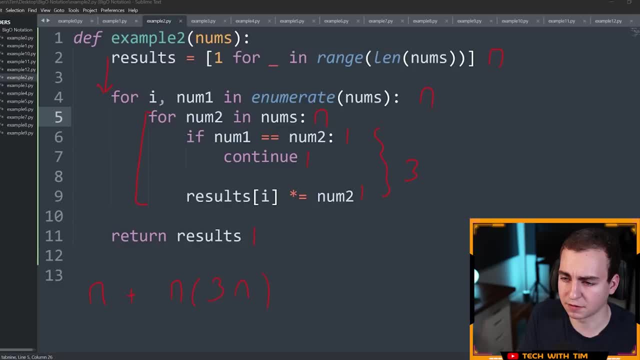 going to be multiple Applied by three N. Now I get this is a bit confusing, but what's happening is this four loop is happening every single time. this four loop runs. So we're doing this four loop N times, which means we're going to have N times N, right, Two ends there, So that's N squared And then we're 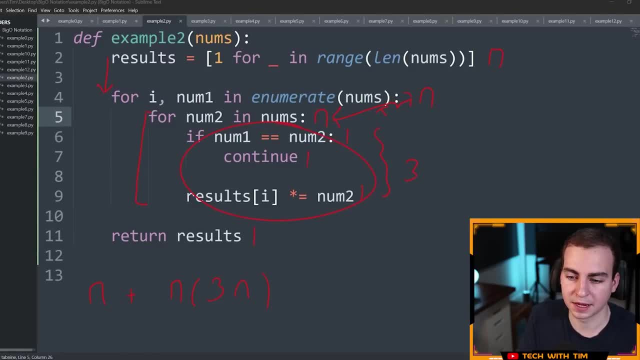 doing three operations inside of this internal four loop, And so what we end up getting is three N squared. If we multiply these all together, we're going to get N plus three N squared, And then we have one more operation here, So we add one. So this is going to be three N squared, And 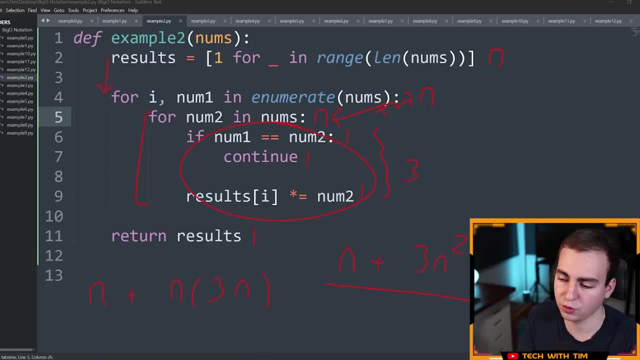 this is going to be the- you know approximate number of operations that we're doing inside of this algorithm. Now what do we do? Well, we look for the largest term, which is N squared. We cross off all of our constants And then, whenever we have a variable, we say: okay, well is this term. 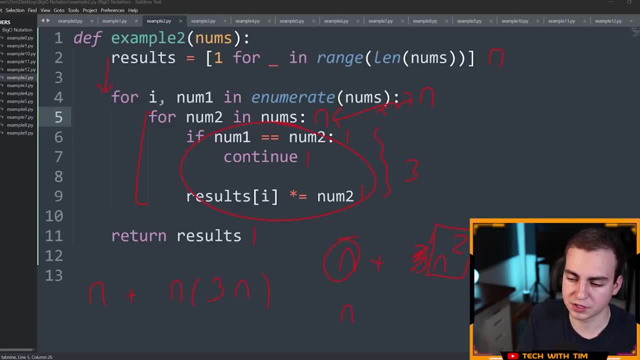 smaller or larger than this one. Well, it's smaller. So if we assume it's N squared, then we could write this as two N squared, which means I can now get rid of that, And that means my big O notation is going to be N squared. I know I made a complete mess here, but this is going to be N. 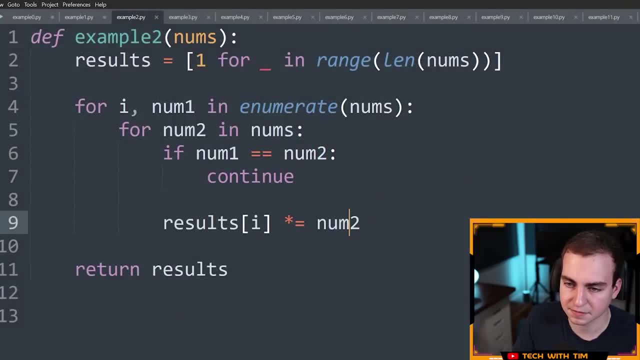 squared. Okay, That's the bigger notation. Let me get out of this mass. Let's look at it here. uh, in the code editor. So we perform an N operation. that happens, Okay. Then we go inside of here and we have an N times N operation, because we're doing this for N times. 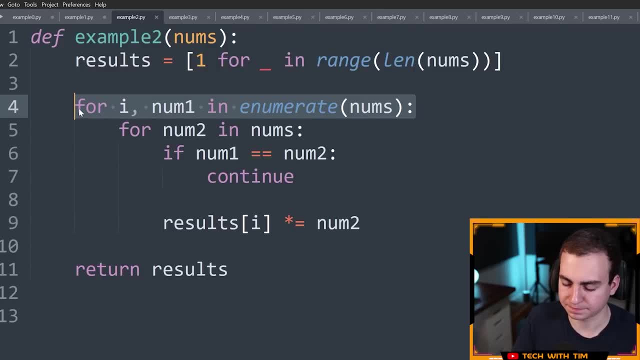 for this for loop, which happens N times, You need to multiply them together. inside this for loop, We're doing three things. So we have three N squared. That's how long all of this takes to run. So we add that to N and that's a one, and we get three N squared plus N plus one. We know the. 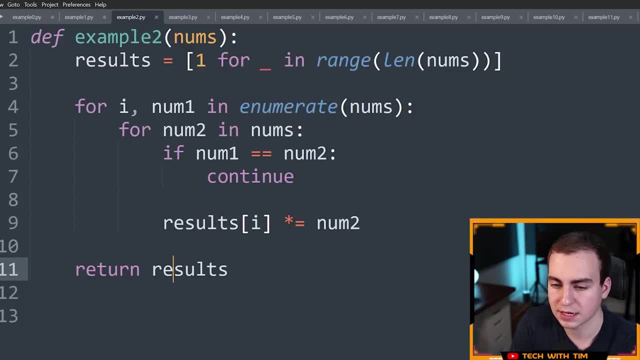 other terms are smaller, So we cross them off, and that leaves us with the big O notation of N squared. Okay, So big O of N to the exponent two. let's write that there. Okay, This is going to start to make sense as we go through. 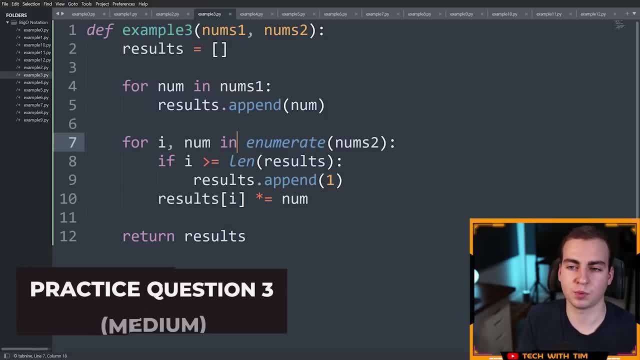 more examples, though that was an N squared algorithm. Now we're moving on to this, So let's look at this. Now we have two inputs here, So it gets a bit more complicated: num ones and nums two. Now, just like we used N to represent the size of our first input, we're going to use another. 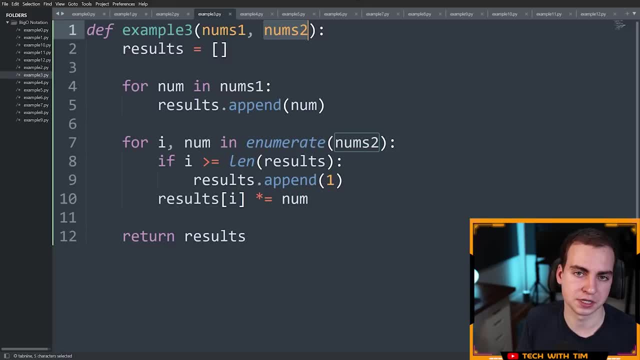 letter, in this case M. you can use whatever you want, but the tradition is N and M for the second input. So we have two inputs. You got to consider with the length of the size of both of the inputs, How long does this take? N and. 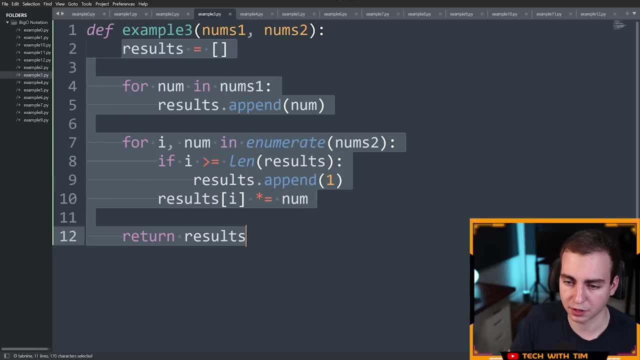 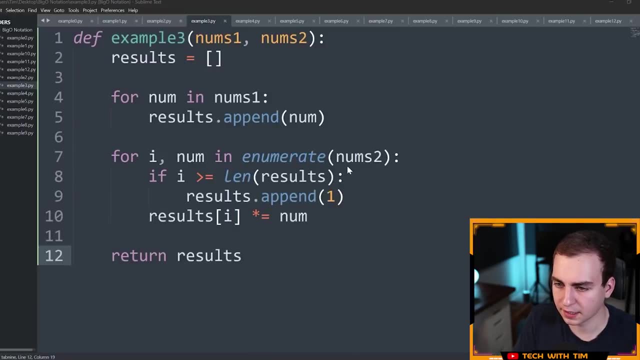 M. Okay. So pause the video if you need to, and take a guess, and I'm going to run through it. So again, let's take a full screen snip here, Let's go full screen snip and let's try this. Okay, So we have. 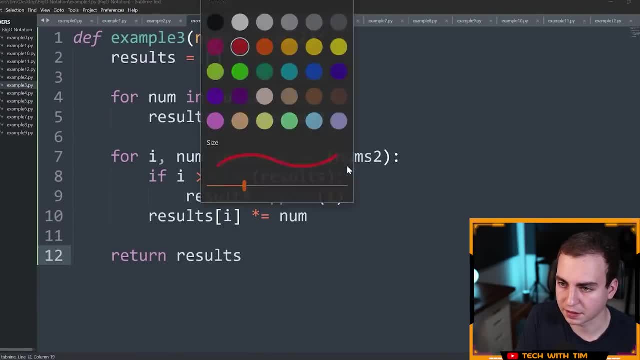 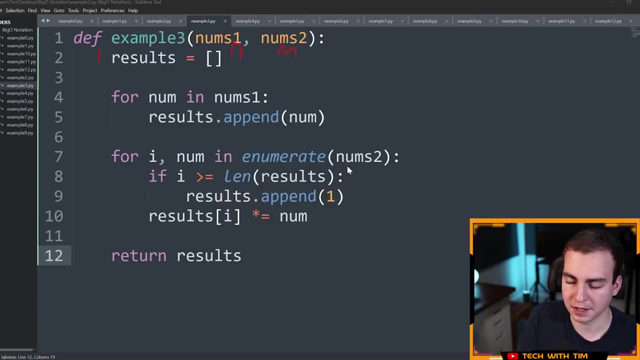 nums one, nums two. So for nums one, can I change the pen color here? Actually I think red is fine. We'll say this is N and we'll say that's M. okay, Results: one operation for num in nums one. Well, 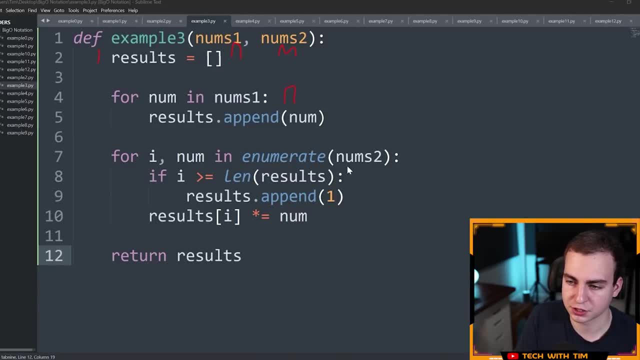 nums one, that's N and M N. So this is going to take N. How many operations are we doing? Just one, So we can say this whole thing just takes N time. Okay, Nums two: this is M right Size of that input inside of here. How many? 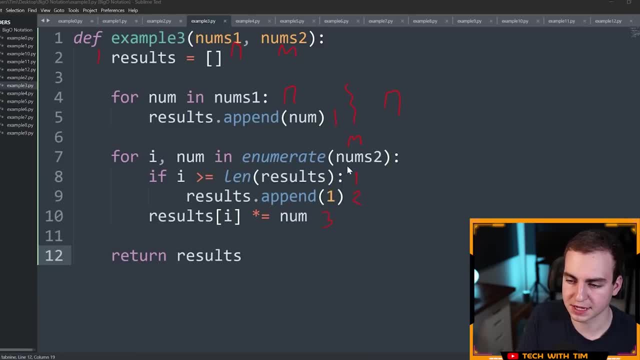 operations are we doing? Just quickly add them up. Doesn't need to be super precise: One, two, three operations, Okay. So this is going to be taking three M time. results: that takes one. Let's add these all together because they're not inside of each other, So we can just add them together. So 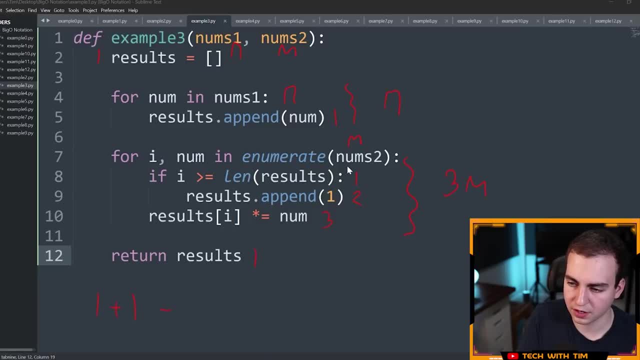 we're going to have one plus, we'll add the other one down here. So one plus N plus three M. Okay, Now we need to cross off all of the constants. So we get rid of one, get rid of one, get rid of three. What does that leave us? N plus M. Okay, We can not simplify this. 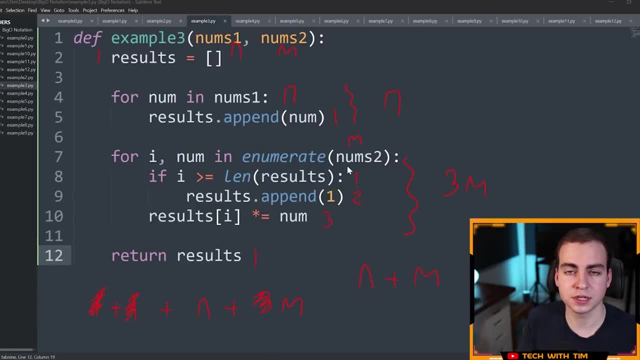 any further because N and M are going to be two distinct variables representing the two inputs that we have to our function. So you're going to see this a lot. You have multiple inputs. You need to use a different variable to represent each input And then that tells you the approximate. 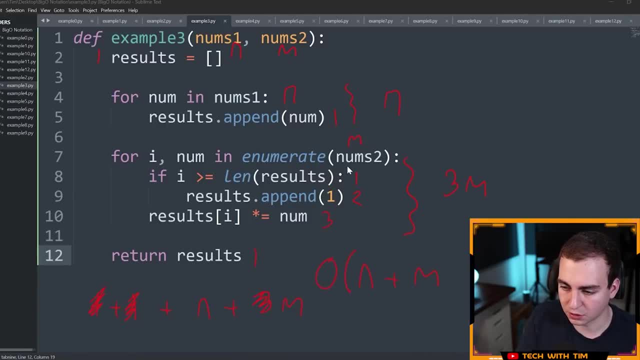 time, complexity of the function. So again, we're going to write this as big O of N plus M. If you want to do this really quickly, all you would do is look for the loops that involve N and M. So we see we have a loop here with N, So we have a. 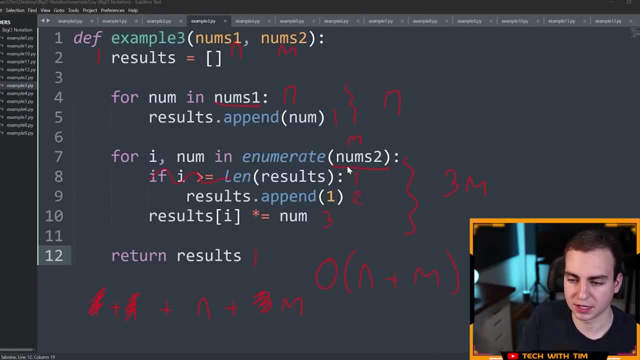 loop here with M, boom, All we do: N plus M. That's all we need to look at Now. we can look inside of these loops and try to see if there's more looping. If there's no looping and it's constant time operations- which all of these are here, that we don't have to consider them, We just cross them. 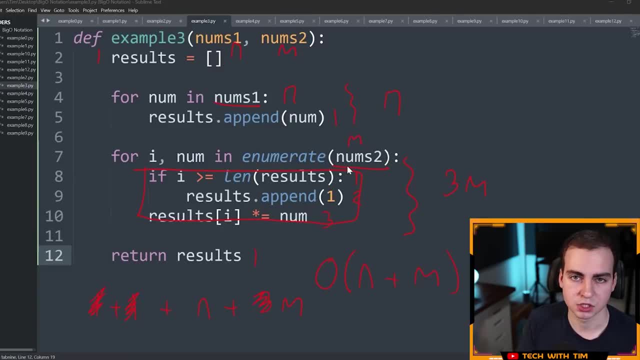 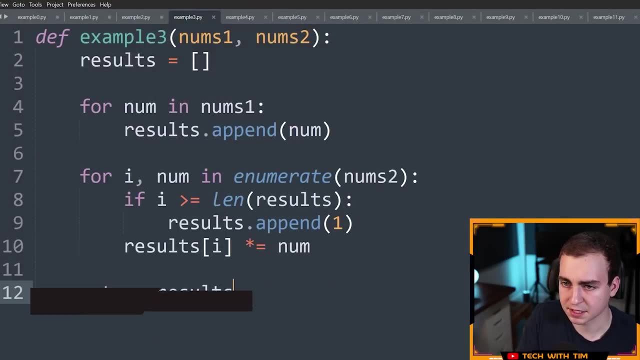 off because they're constant. Every loop it's going to take the same amount of time, So we don't need to consider it. It's not based on the size of the input. Okay, So O N plus M. Okay, Let's continue to example four. I got a ton of examples to keep practicing. 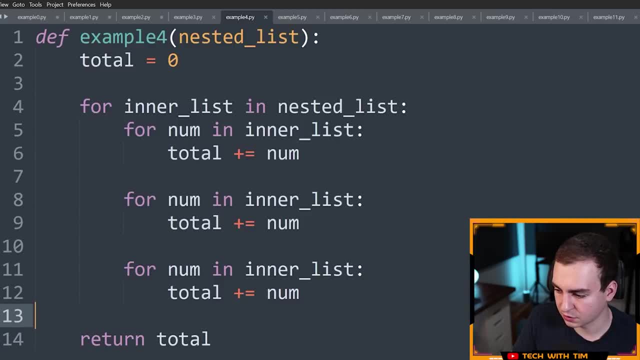 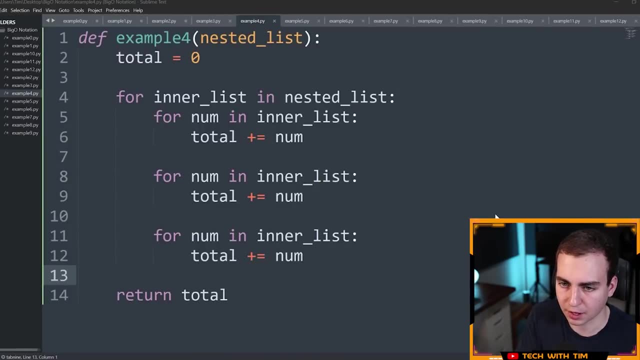 this, Okay. So now we're doing a bunch of stuff here, So let's again go to the full screen snip. You guys can pause the video if you want and take a guess at what the time complexity is. Okay, So we have example four. we take in a nested list. Now the nested list is going to 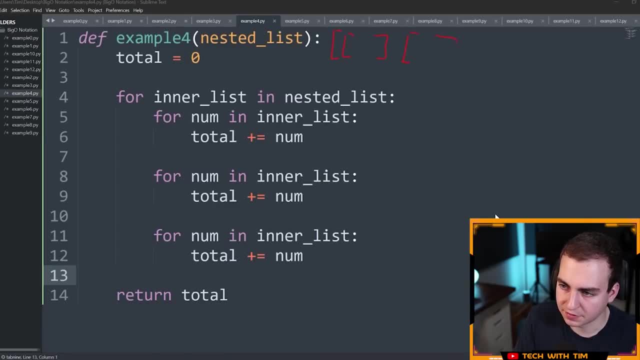 be something like this: right, There's going to be a list inside of another list, and this can make it a bit complicated. So when we're dealing with a nested list, what we're going to do is assume that the list has a height and a width. Now we could draw this in kind of more of a square. 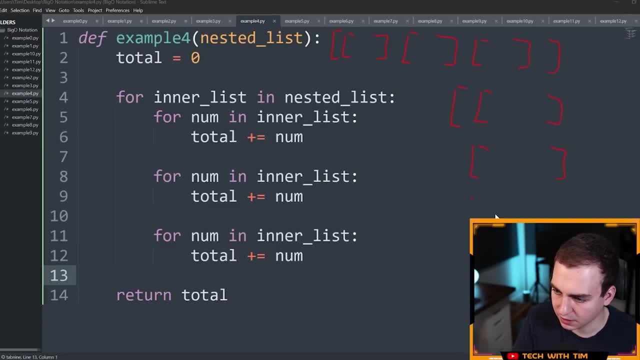 fashion, but it might be something like this: Okay, And what we would get here is this would be the height, So the number of lists inside of the list, and then the width would be the number of elements inside of each list, And we would assume that would just be the same. Okay, So we 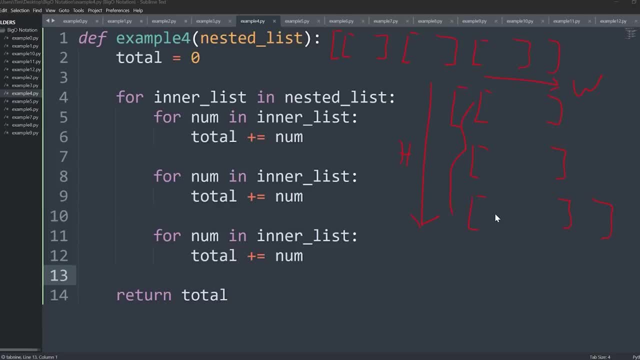 have height and width, and those are the two variables that we're going to use for the time. complexity here, because we need to represent the number of elements in the interior list as well as how many lists We have. Okay, So let's look at this. We have one operation. I'm going to stop counting these. 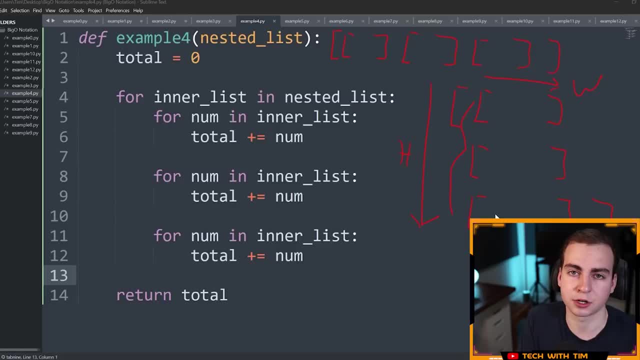 now, because we don't need to even consider them in our operations. We're going to cross them out. Anyways, it's just one single operation, It's constant. It doesn't matter, We can just stop looking at it, because it's not going to be based on the size of the input. However, we have a four. 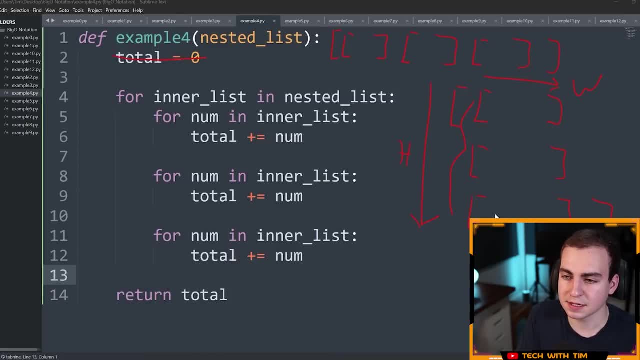 loop. We say four inner list in nested list. Well, nested list, uh, we're getting all of the inner lists. So how many of those lists do we have? We have H of those right, H nested lists, Okay, We. 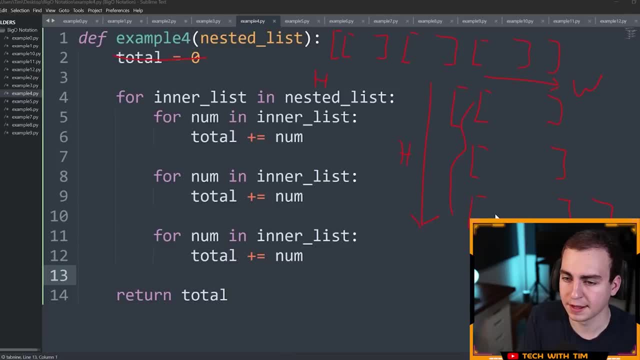 could write that lowercase H doesn't really matter. Then what are we doing? We're looping through the inner list. Now, the inner list is what well it's going to be w, whatever the width is or the number of elements in the inner list. 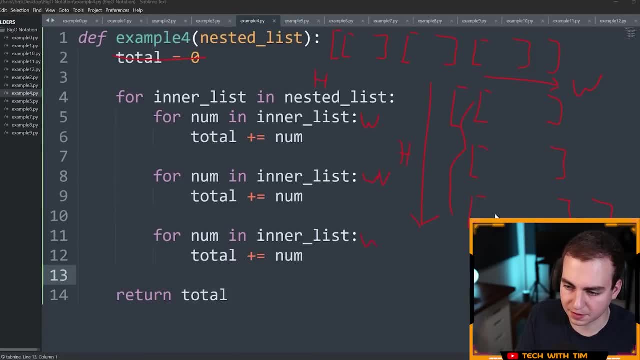 So we're doing w here. We're doing w here because it's the same thing and we're doing w here. So we have H times three w, right? So inside of here three w operations times H, So we get H, and then this is multiplied by three w, So that gives us three H w. 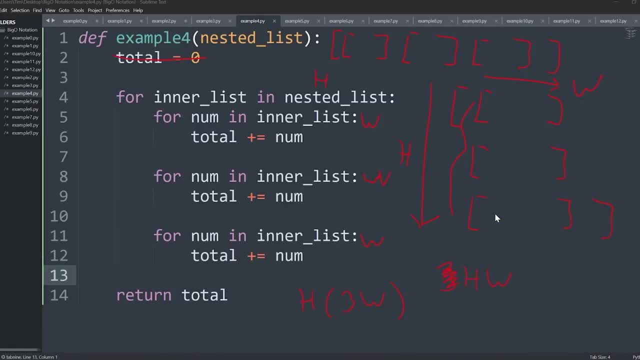 And what do we do? Remove the constants and we get H w. Okay, So we can write this as run out of space here, big O of H w, And you know we'll just make it uppercase to stick with what we have. 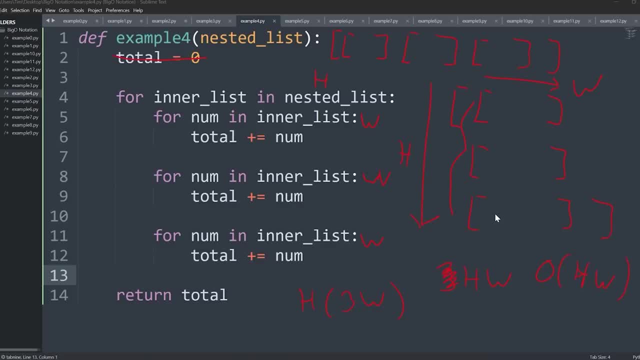 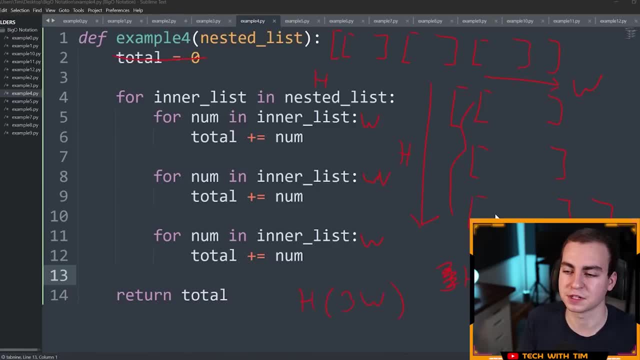 obviously doing this with no one giving me any feedback. It's a little bit difficult to know if people are following or not, but I think this is a decent explanation. We have H inner lists, So we have H times. We're going to do this for loop, right here And then inside of the inner list. 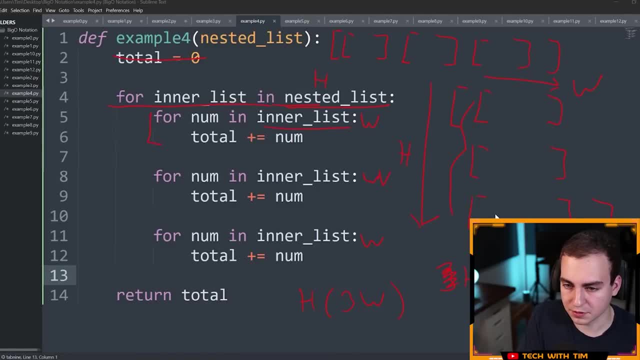 we have w elements, right. So we're doing this for loop w times, this for loop w times as well. So we're doing three w for every H, So that's going to be H times three w for the number of operations. We have a constant in there which is three. We don't care about the constant, We remove. 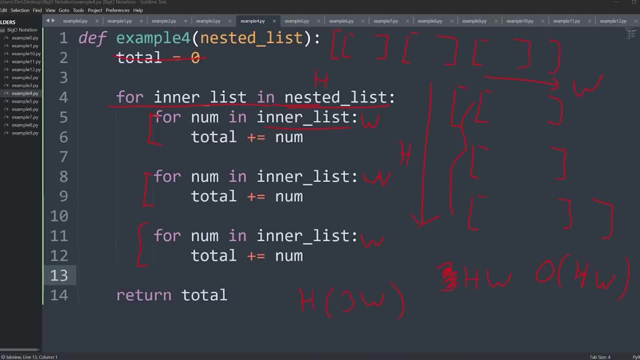 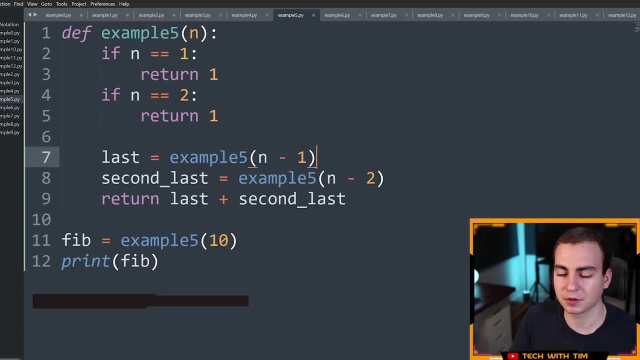 it and we get w times H- Great, Okay. Next example, example five. Now this is a recursive example. I'm going to be a bit more difficult here. What I would recommend you do is try this with a very small value. So try. 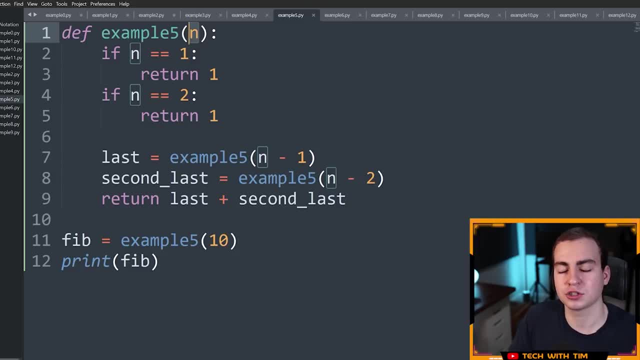 this with number three, or try this with a value two and see what actually happens when you give it kind of these small values and how many operations end up happening in that case. Okay, So I'm going to go to the screen snip now and let's look at this. Okay, So this is a recursive example. 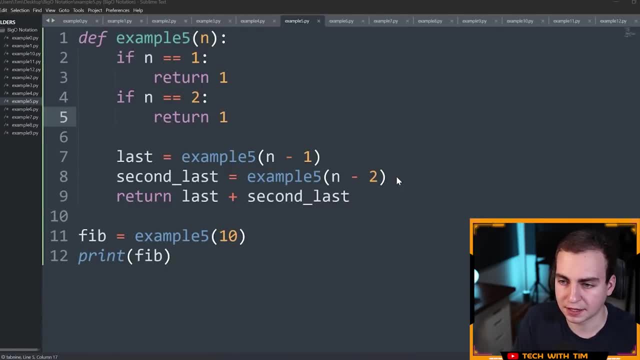 It's actually a very famous problem. It's the Fibonacci sequence. Now I will just tell you that the bigger notation is two to the exponent N, but we want to walk through why we're getting two to the exponent N. So we need to understand how this code actually works. So we're going to. 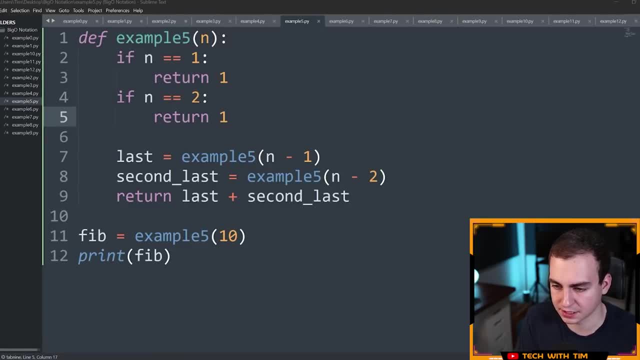 deal with a lot of recursive stuff. when we're looking at time, complexity analysis And the important thing to look at here with recursive functions is how many recursive function calls are happening in every step. So we want to figure out essentially how many times is this? 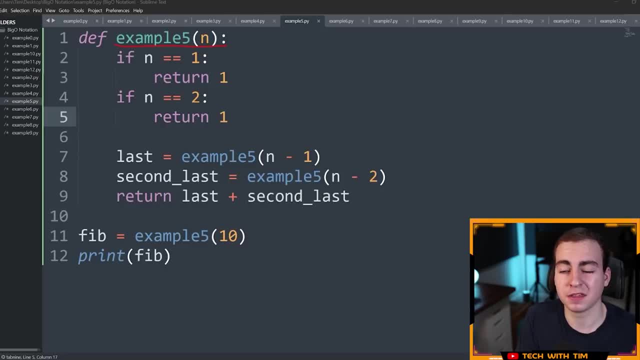 function going to run, And then we want to multiply that by the number of operations occurring in the function. That's how you deal with recursive function calls: How many times does the function run? multiply that by the number of operations inside of the function. 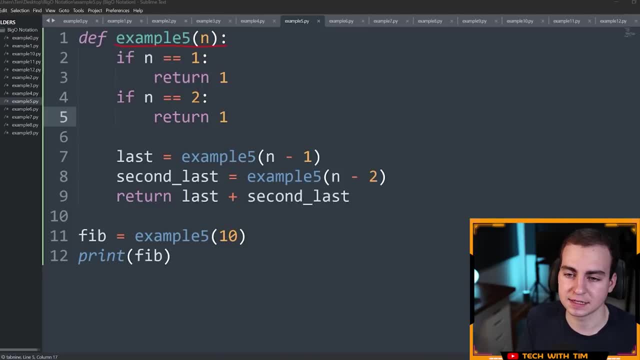 Now, the first thing we're going to look at here is the operations of the function, because that's the easiest to figure out. So we have, these are constant time operations, right? So we don't need to consider them. These all take constant time. Okay, All that, So we 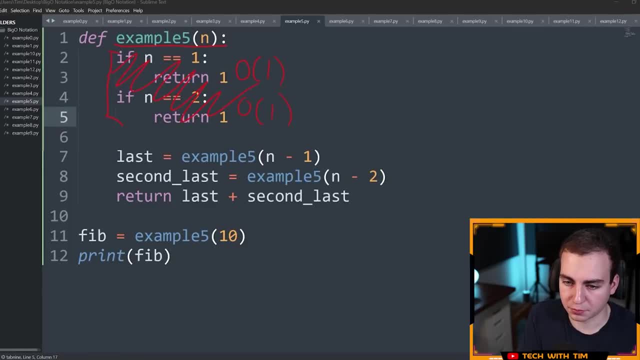 can kind of cross all those out. We don't even care about those. Now, this operation right here, this is a recursive function call. So we're not going to consider that, because that's going to have to do with how many times the function runs. again. recursive function call. And then we have 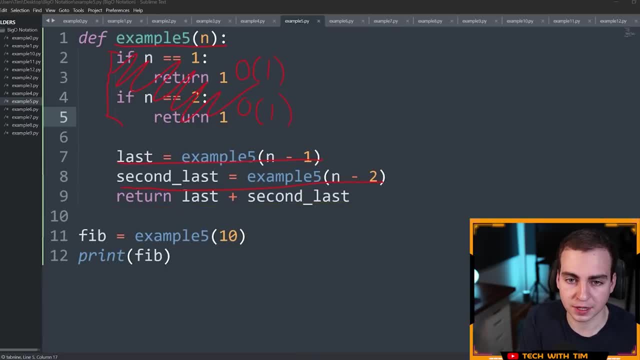 another constant time operation that we don't really care about. So if we're looking inside of the uh, the actual function itself, we'll just say that the function takes constant time to execute. However, how many times is the function going to run? Well, that's based on. 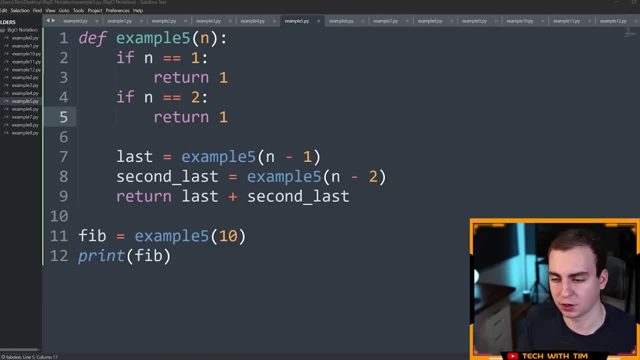 these recursive calls. So once we figured that out, we'll know the time complexity. So let's just do a simple example here with an input of size five. So if we have five, then what we need to do is we need to call the function at four and at three because we have 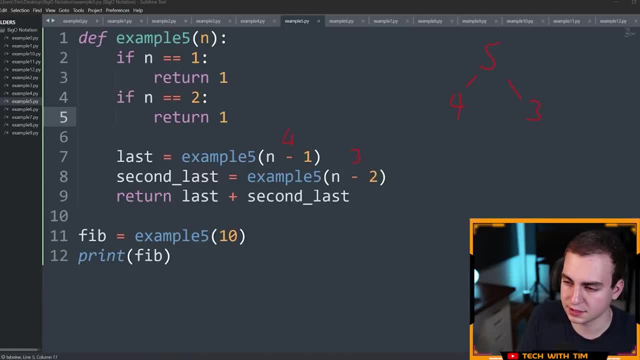 four here and three here when N is five. Okay, Those are the two function calls we need to make from four. We're gonna have to make the function call three and two. by the way, I'm not making these in the order they're going to be done. I'm just trying to write out the whole tree from three. 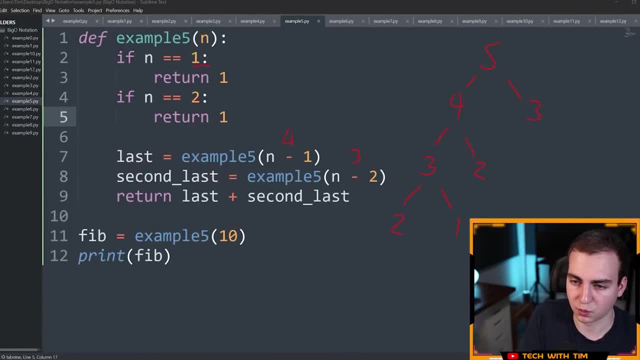 We're going to have to call two and one. Okay, Cause our base cases are one and two. So whenever we hit one and two, we're done. So, done, done, done from three, We're going to have to call two. 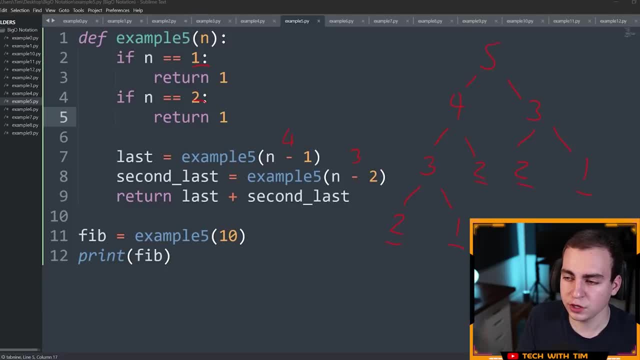 and one. Okay, So this is what our tree looks like. So what you should be noticing here is that we're going to end up getting a time complexity of two N. So the reason why we're getting two N here is because for each input to the function, we're doing two recursive calls. 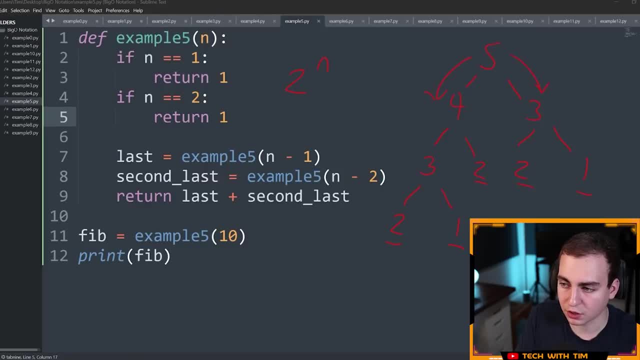 So if we start at five and we do a call to four and we do a call to three, we've done two calls, And then, from these numbers, we need to do two calls as well. Now we are going to end up doing less than two N operations. However, this is the best function we can use to approximate. 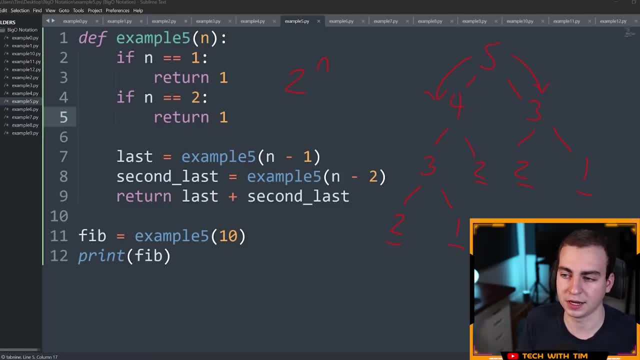 how many operations are going to occur in this function or in this algorithm. So we have two recursive calls. The calls are going down by any minus one and N minus two, So a constant value. they're decreasing by, not something like divided by two, divided by four, which would be 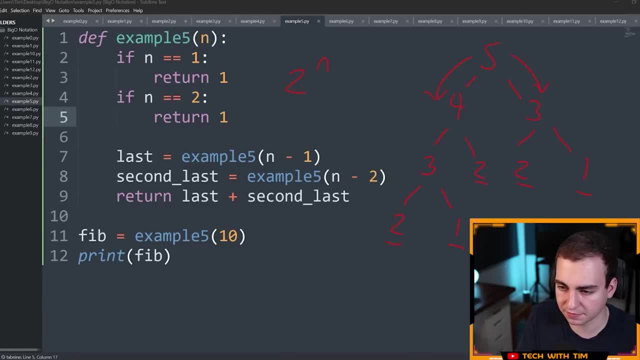 much different. We'll look at that in a second. We're reducing these by constant value, So the most amount of steps we're going to have to do for every input is two, And that means we're going to have two to the exponent and potential steps. Now, if you want to prove that to yourself, 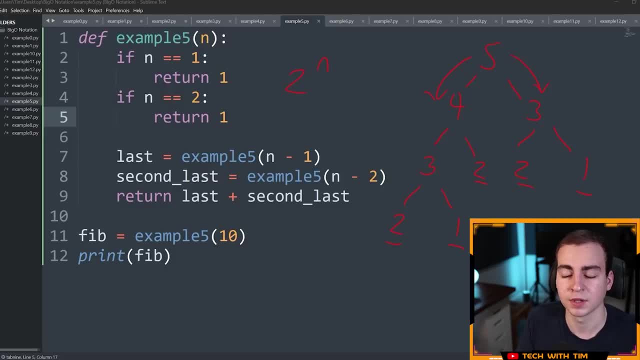 keep expanding this tree. look at six, look at seven, look at eight, look at nine and you're going to see how many operations you have to do and how we expand in this way, In an exponential way. Okay, So two to the exponent. N is the time complexity here. This is 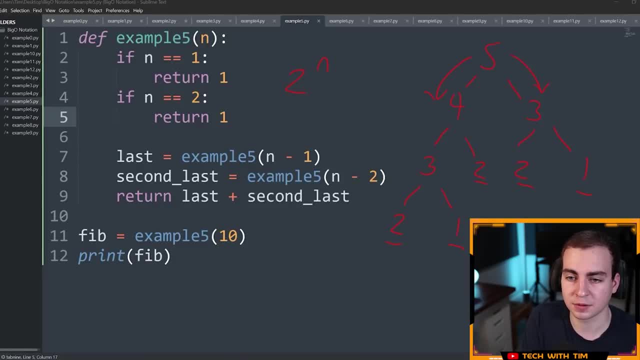 kind of just a complex Do you have to be familiar with. and again, the way I determine this is how many function calls I can have at most. Now, again, I will have less function calls than this, but this is the most approximate function I can use for the big O notation. So we have big O of. 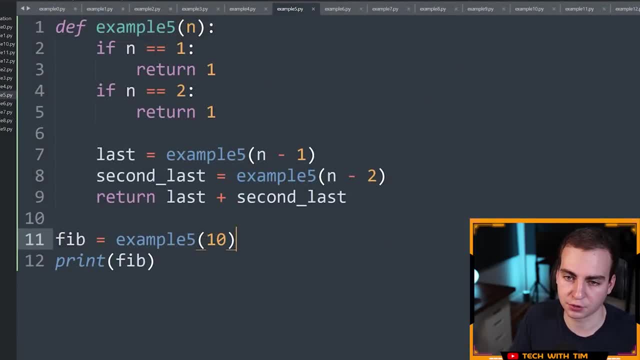 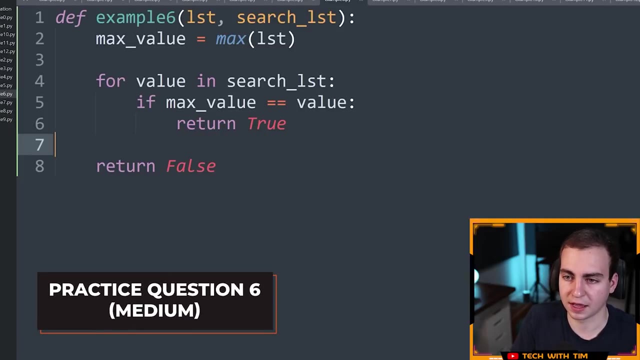 two, N, all kinds of other videos on the Fibonacci sequence that can probably explain that as well in more depth. So let's write the comment of big O, of N or, sorry, two, to the exponent. Okay, Now let's go to example six. All right, Example six, So this one. we have LST and search. 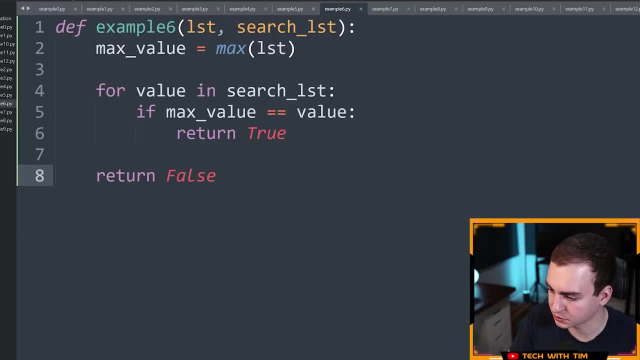 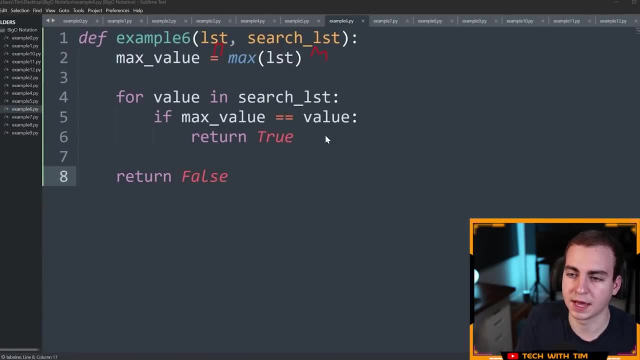 list. Actually, let me go back. I don't know why I keep it, keep going full screen here. Let's go and take a snip. Okay, So we're going to call LST here and, and this will be so two different. 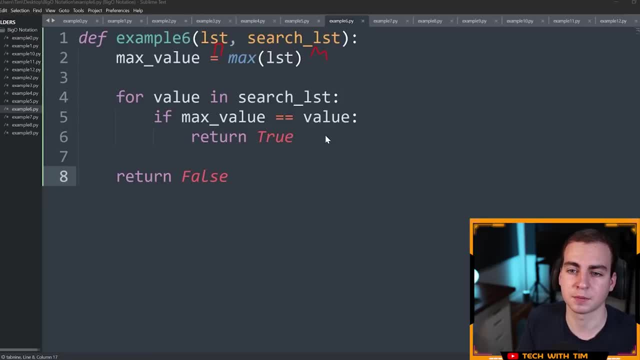 inputs. We have two lists. Go ahead, pause the video, determine the time complexity. Okay, So let's get started here. So the first thing we need to do is we've got to look at this operation here Now. a lot of you are going to say that this is a constant time operation. 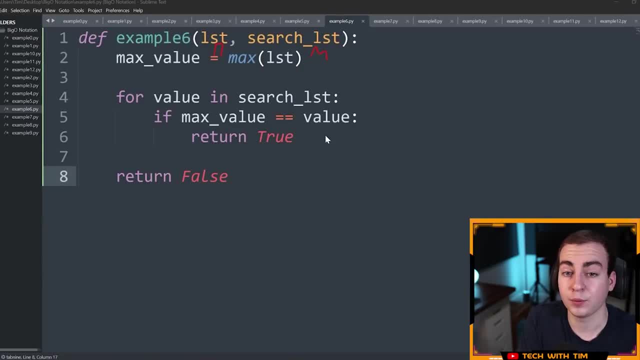 Just happens in a one. right, We just count this as one operation. Now we can not, because what max actually does in Python is it loops through the entire list and find some maximum value. So you gotta be careful here Whenever you're using internal language features like built-in. 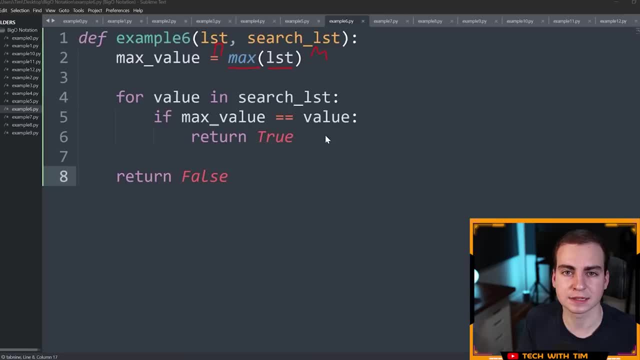 functions, max, min, stuff like that, even, uh, you know, slicing an array, for example, slicing a list, you need to actually consider what's happening on the lower level and how long that's actually going to take. So if I want to find the maximum number in the list, the only way for me to do that is to search through every LST. Okay, So let's go ahead and take a look at this. So let's go ahead and take a look at this. So let's go ahead and take a look at this. So let's go ahead, and. 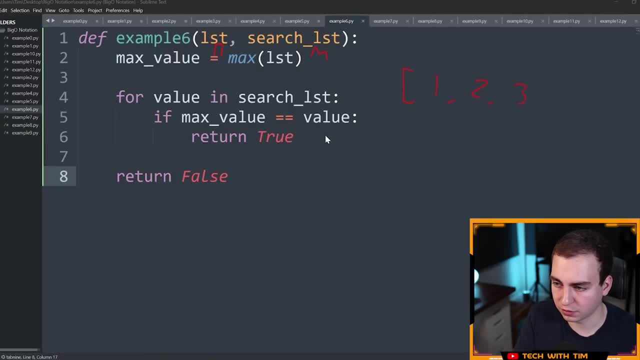 find the minimum element in the list. So if I have a list, I have 1,, 2,, 3,, 4, and I'm looking for element two. Okay, Yeah, It only takes me two steps to go through this, but I still need to say: 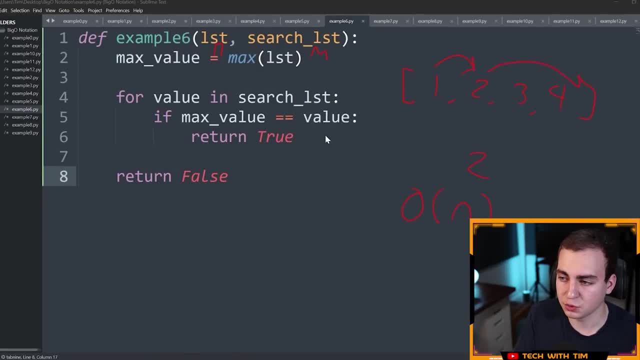 that this is going to take me Oh and time, because if the element two was pushed to the very end of the list, I would have to look through every element in the list to find it. So this is where the worst case comes in, right. When I'm searching through a list, I might find the element. 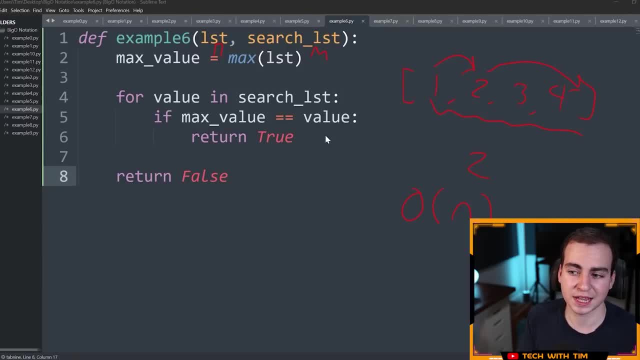 immediately, or I might find it at the very end. So in the worst case I have to assume it's going to take me and time to find the element. So I say that finding the maximum element in a list takes me Oh and time. uh, hopefully. 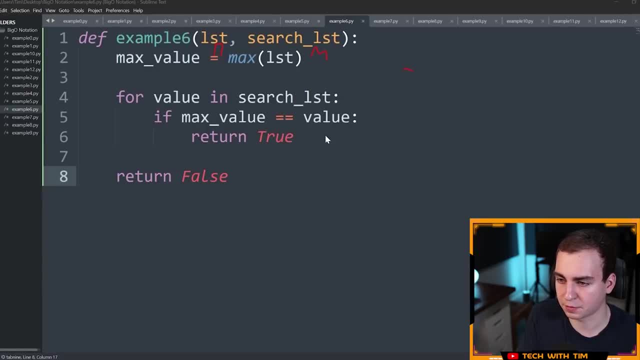 that is clear. So, Oh, and time for this first operation. So let me just write an N here, Okay, So that takes N to find the max. Then we're going to look for a value in the search list, So we're. 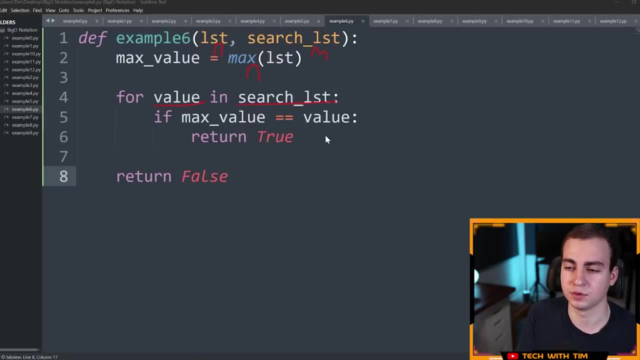 going to say for value in search list and we're going to check if the maximum value is equal to the value and return true. So this here, this is going to take us M time. Now again, this might not take us M time If the maximum value is equal to the value in the very first value that we look. 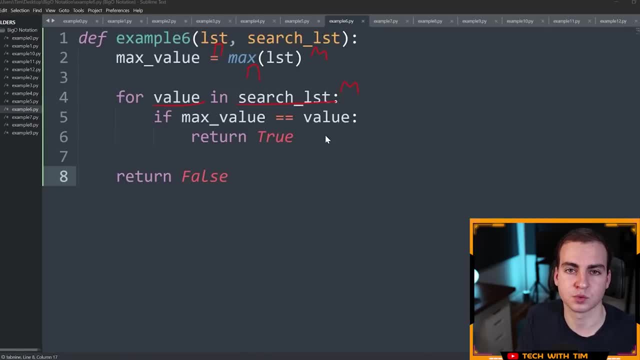 at, we immediately return: true, And this actually took us constant time. It took us one operation to do this. However, if the value that we're looking for isn't in this list, where it's one of the later elements in this list, it takes us M time to look through it. So, in the worst case, 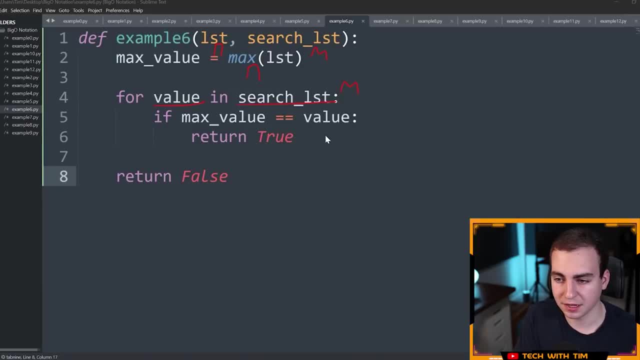 the element doesn't exist, We have to loop through every single element in the search list just to find that it's not there. That takes M time. Now that makes the total time complexity here, And So big O of N plus M. we do the first operation, which is N, looking for the maximum element in. 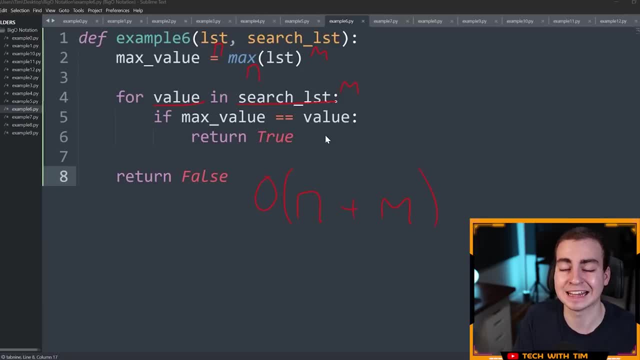 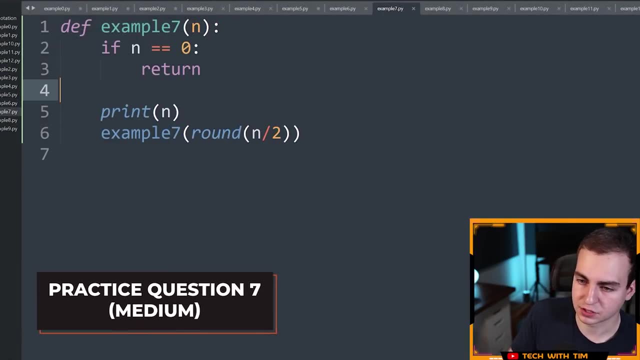 the first list And then we searched through all of the elements in the second list, in the worst case giving us big O of N plus M. All right, let's continue. Uh, example seven: Okay, So this one is a bit more complicated. again, has to do with recursion. uh, pause the video, take your. 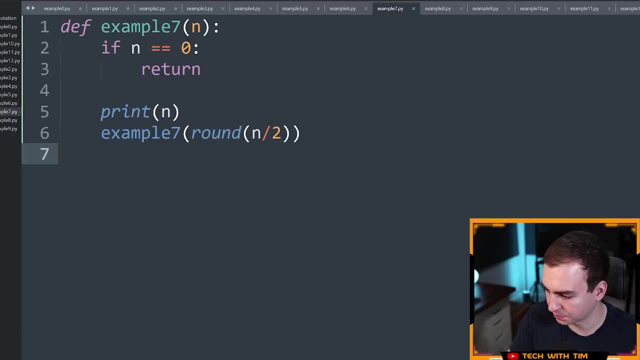 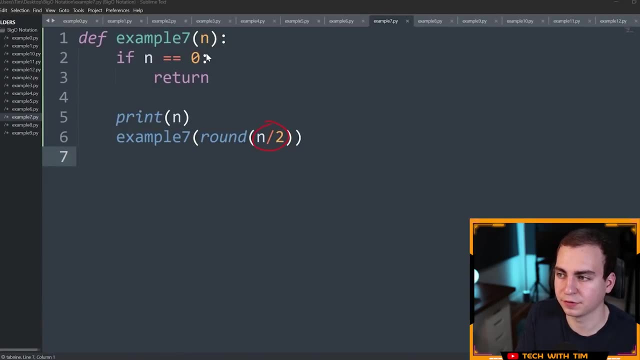 time and try to guess what the time complexity is. Okay, Let's open up our snip here and let's go through this. So for this one it is a little bit tricky, but we really want to pay attention to this N over two here and what's happening in this recursive call. So previously, 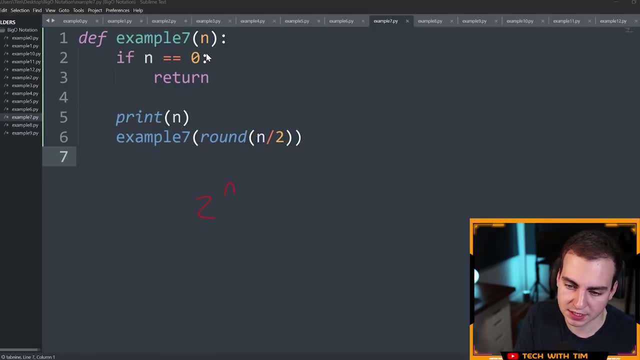 when we saw recursive calls or when that one example we saw it, we had a time complexity of two, the exponent N. Now the reason we had that is because we were calling two calls for every single input right, So each input five I'm calling, I'm calling the function twice And I was only 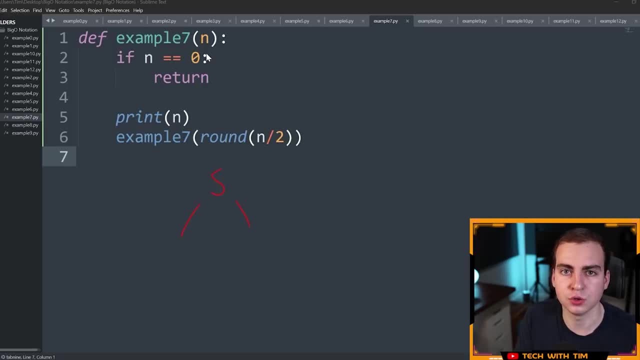 reducing N by a constant amount. I was reducing it by two, three, four, one. any constant amount that I'm reducing it by is going to cause me to get Something like two N. Now, if I had three recursive calls, I would've got three N If I had four. 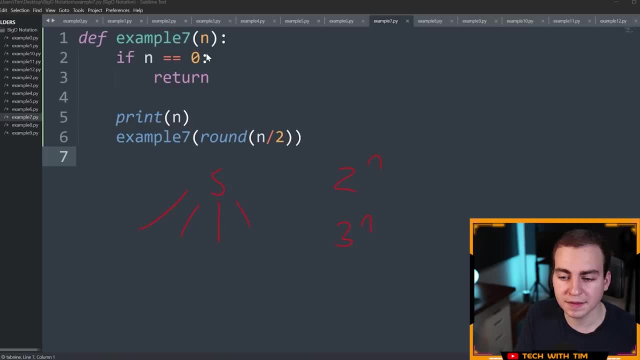 recursive calls for every input, I would've got four N, assuming that I was reducing everything by a constant value. Now, here I'm only doing one recursive call and I'm reducing this not by a constant. I'm saying N over two, So I'm actually reducing it by N, like N is a part of the. 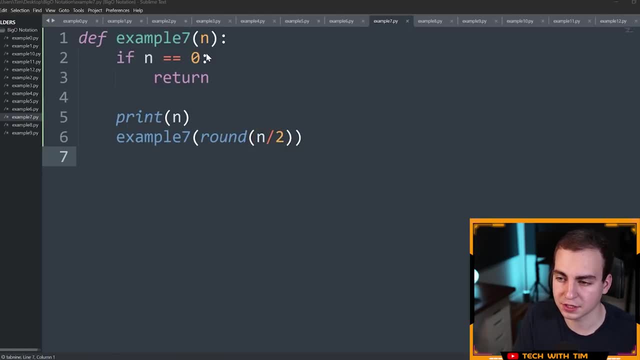 reduction factor, if that makes sense. So when I do something like N over two, you can see that I'm very quickly going to get smaller numbers. So 40 goes to 20, 20 goes to 10, 10 goes to five, five goes to 2.5, 2.5.. Let's round it. It goes to one right. 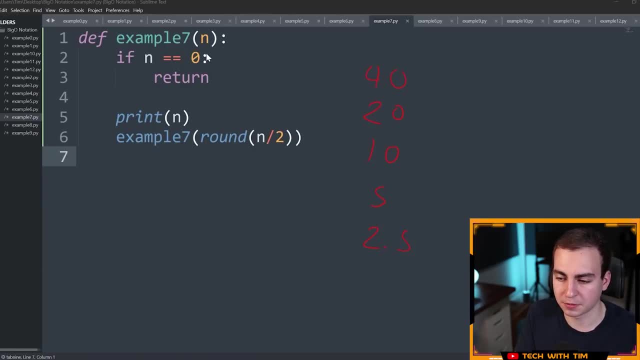 So this is how quickly we reduce from a very large number. Now this is actually logarithmic. Okay, This gives us the long base two event is the time complex Again, I'm going to continue to explain this, but you need to keep this in mind. So we have log base two of N, So N is constantly being 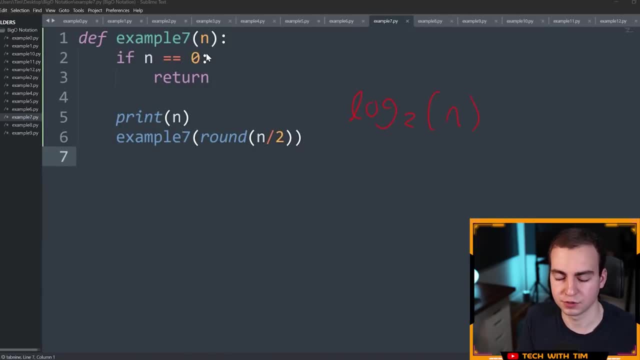 divided by two. Every time it gets divided by two, that's reducing in a much smaller N Right, And so that means we Only are actually going to do log base two of N recursive calls, or at least that's what our time. 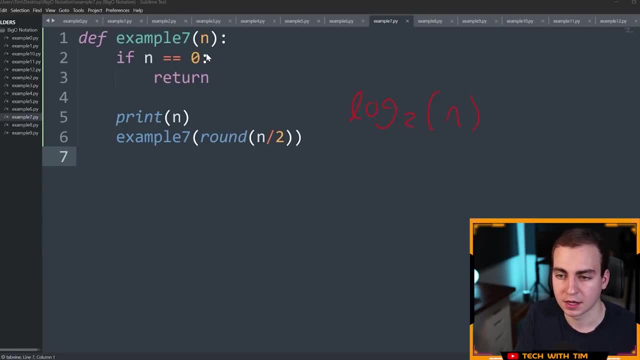 complexity is going to be, because that's how we're reducing it. So again, if we start with N equal to say a hundred, then we're only doing one recursive call and the next recursive call goes to 50.. Then it goes to 25, right. Then it's going to go to approximately 12.5.. We're rounding this, So it. 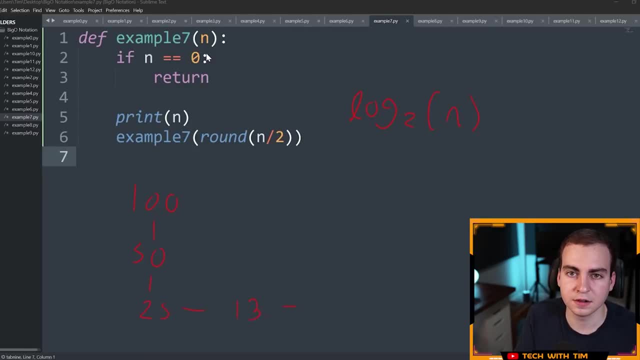 would go to 13.. Okay, That's fine, It goes to 13.. We divide 13 by two, That's going to give us approximately seven. Okay, Divide seven by two, That's going to give us approximately Four. divide that by two, We're going to get to. divide that by two, We're going to get one. So 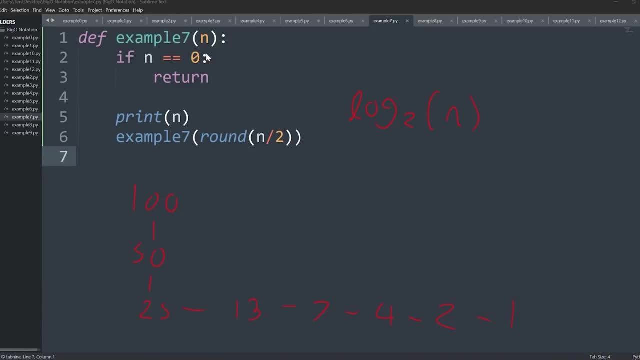 log base two event is telling us how many operations because we're reducing by a factor of two. I don't really know if I can explain this much better than that. If we had a three, then this would be the log base three of N. okay, Not log base two. reason it's two is because that's. 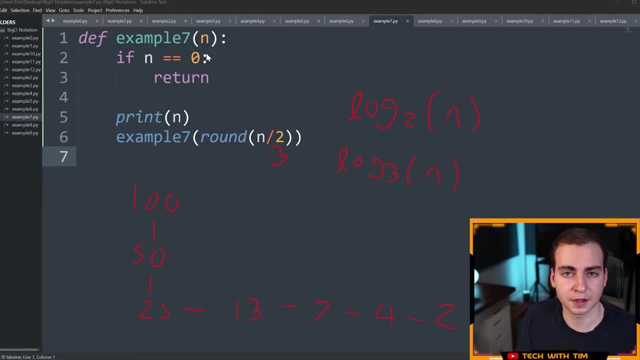 what we're dividing by. So really, you can just kind of plug in some numbers and see how many operations is actually going to take when we're doing recursive calls or we're reducing the number of operations by dividing it by two or dividing it By four, dividing it by five and N is what we're dividing it by. Well, that means we're going to 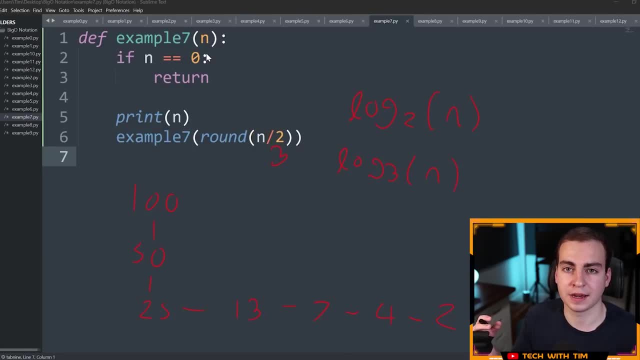 get some type of logarithmic time complexity and the larger and gets the fewer amount of operations we're actually going to have to be doing. Now, that wasn't the most accurate way to say that, but you get the point. as N gets really, really large, The amount of operations we have to do is not growing. 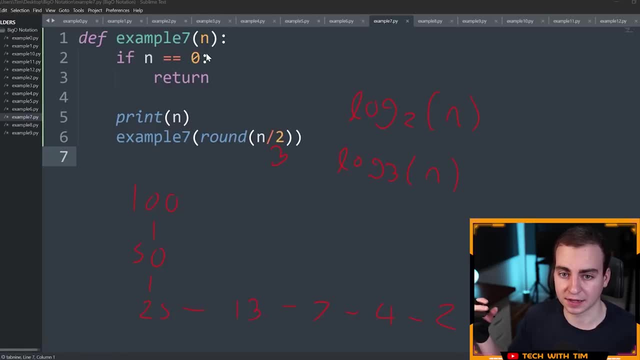 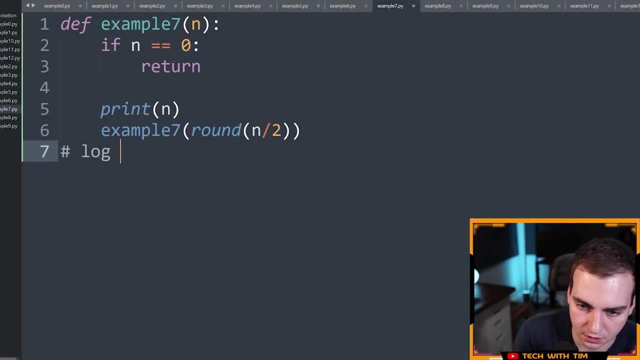 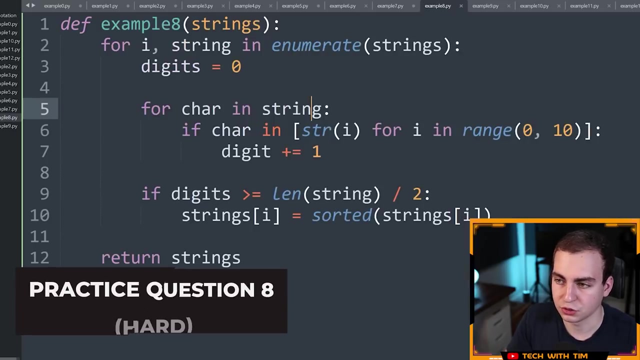 with the size of N. it's really small relative to end when N gets very large. That's kind of what I was trying to say. Okay, So that's that one. So this is simply the log of N. Okay, And this is log base two of N. don't really have a better way to write that. Okay, Now let's go to. 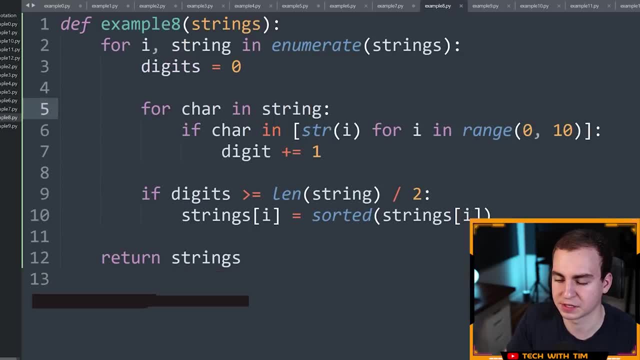 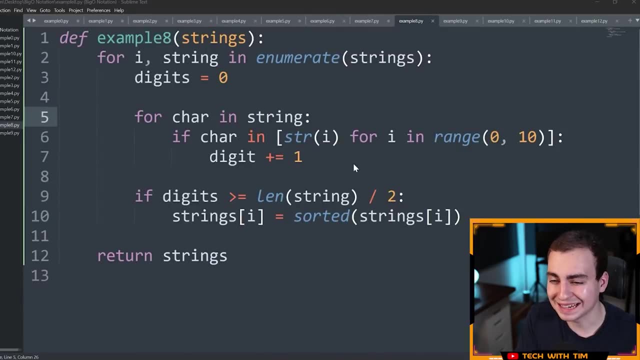 example eight. So let me get the snip here again. pause the video If you would like to try this out on your own. So you're saying we're taking a list of strings, Okay, So these are going to be multiple strings inside of a list. We're saying four, I string and enumerate strings. So 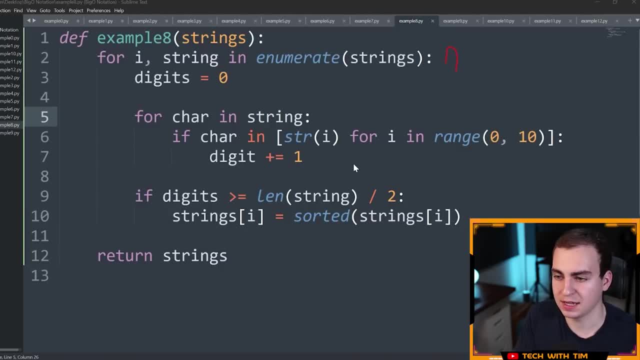 immediately, we're going to say this is going to take N time, where N is the number of strings that we have. Okay, The size of our input. Now, with strings, though, right, If we look at a string like hello, the number of characters in a string is going to dictate how long it takes to process that string. 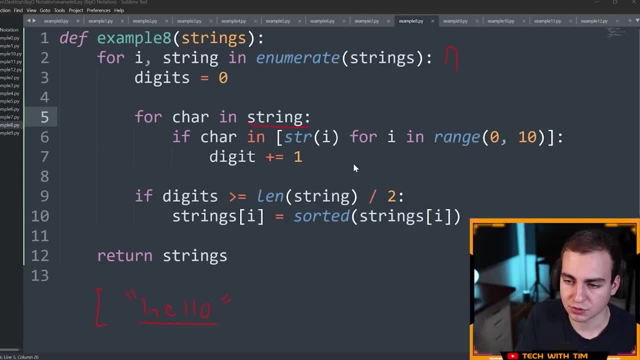 which you're about to see here. So I have four char in string. Now string is an individual string, So there's not really a good way for me to figure out how many operations is going to take for me to process a string, because I don't know the length of the string, So I need to come up. 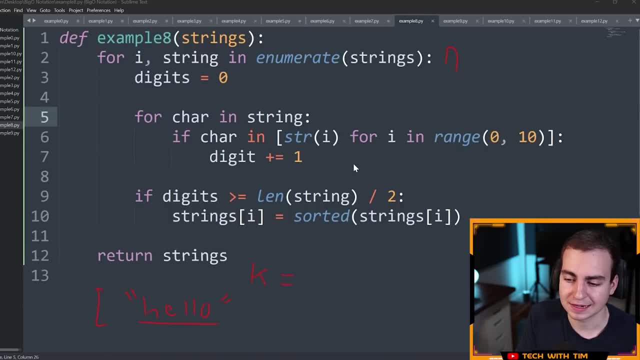 with another variable. here I'm going to use the variable K, and K is going to be the max length of any string inside of this list. So I'm going to say this is K. Now. the reason I'm doing this is because, whatever the maximum length of a string, 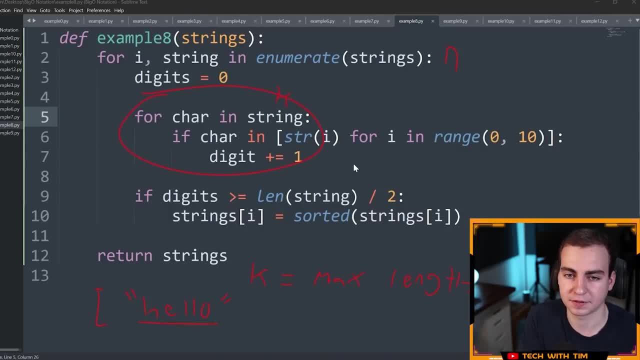 is that's the most number of times that this for loop is going to have to execute, And I'm looking for the worst case scenario here, So I can approximate all of the other strings length to K, because K is the longest length of any string that I have. So that's the most amount of times it's going to have to happen. 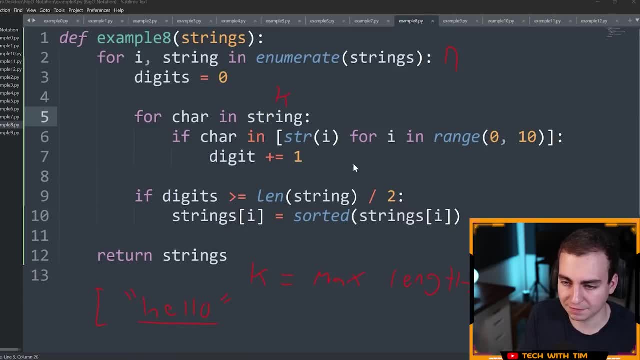 So I say it's K. now, inside of here, what am I doing? I'm saying, if char is in string, I for iron rain zero 10.. Now some of you may be tempted to include this As part of your time complexity. this is constant. This takes 10 steps every time. So, since it always 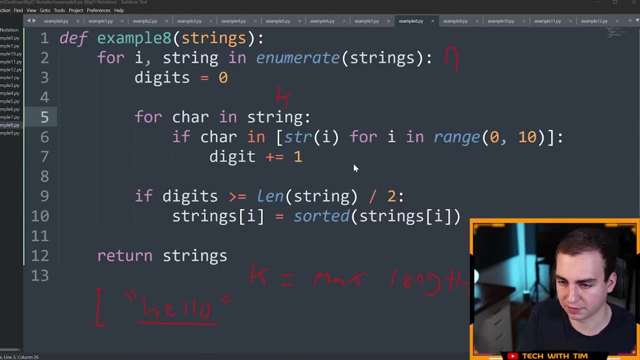 takes 10 steps. I don't have to count it, I don't care about that And I'm not even going to look at this if statement. Okay, So now we have N K, Then I have this: I have if digits greater than or equal to land of string. 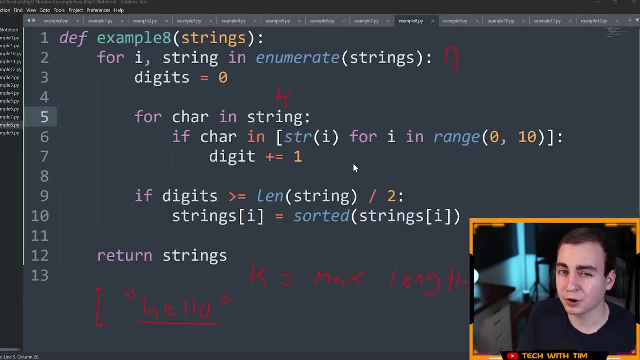 over two strings. I equal sorted strings. Now the only part that I'm looking at here is sorted. Now we should know that to sort a list, to sort of string, to sort anything, the most efficient way we can do this is in N log. 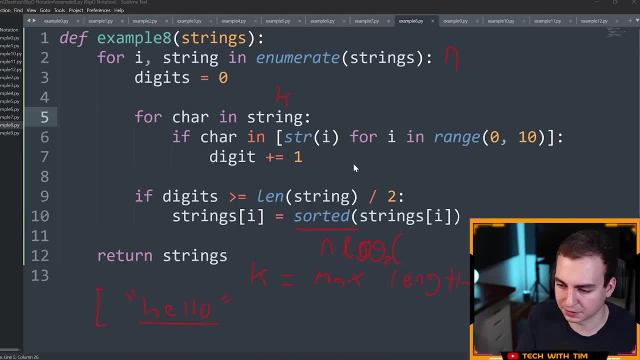 and time where this is based to Now. I completely butchered that, So let me rewrite it, And I'm also going to write it in K, cause that's what we're going to have to use here. So we're going to say K and then this is going to be log. 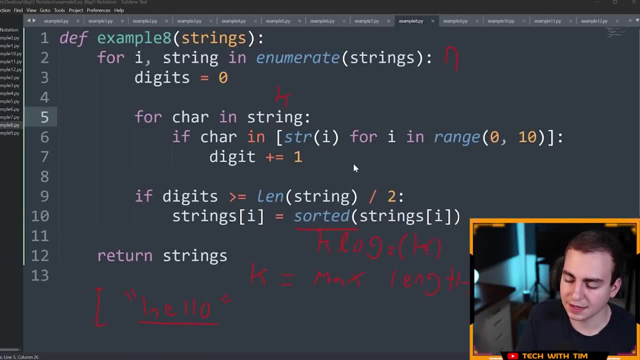 base two of K. Now, K is the length of the longest string, So the most amount of time we'll take to sort something here is K log base two of K. Now if you don't know why that's the case, you're just gonna have to trust me here. 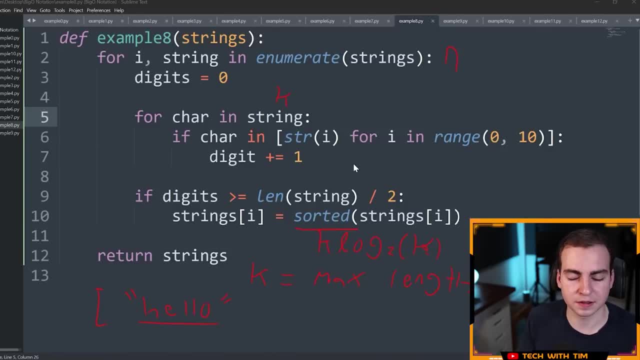 The most efficient way to sort something- uh, at least a general thing that you're sorting, not something specific- is K log base Two of K or N log base two of N. now, K is the longest length of the string that we have. We have to use K because we 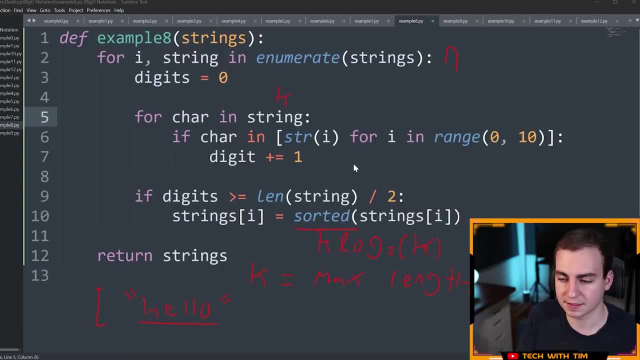 don't know how long the string is going to be. So we say, whatever the maximum length is, that's what we'll put here, because that will give us an upper bound and give us the worst case scenario. So we have K log base two of K, That's. 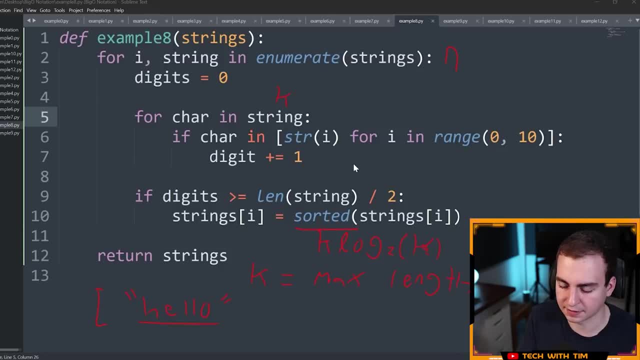 how long this takes. I know I kind of butchered writing it there, but that that's the operation. Okay, So now we figured out our operations. So we have N, we have K and then we have K, log base, two of K. So inside of this for loop right here, 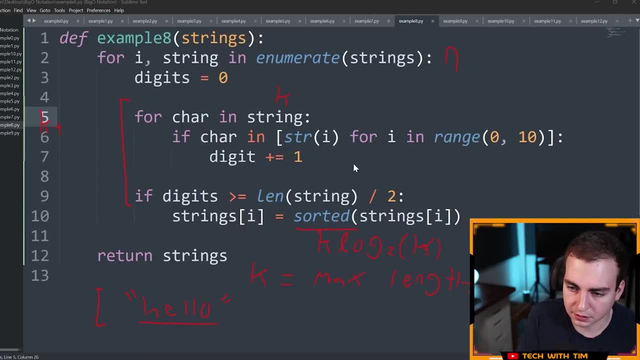 this takes K plus, and then this is going to be: uh okay, You know what- Let me clear this, because it's going to be hard to to do this case- So this is going to be N multiplied by, and then this is going to be K plus, and then K, and this will be the log base. two: 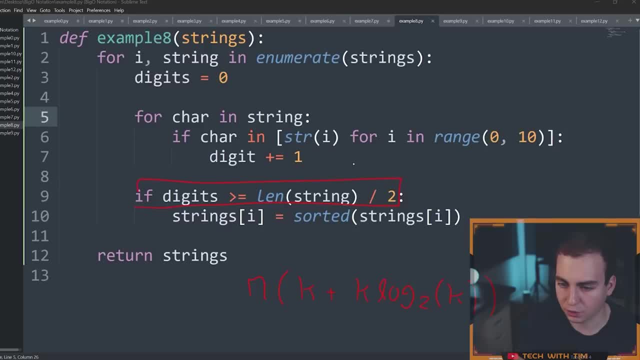 of K. Now again, this is not always going to happen, right, We're not always going to have to sort, but we could always have to sort. That's the thing, It's the worst case. So, since we could always have to sort this, we're going to have to factor that into our time. 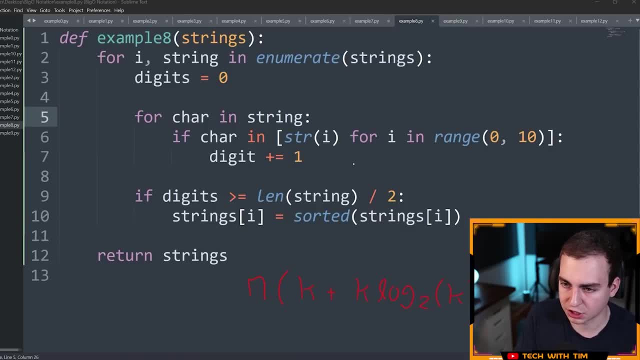 complexity and assume we're always sorting it. So we have N, which again was this, we have K, which was this, and then we have the K log base, two of K, which is here. So inside the for loop, we have the K plus K log base, two of K. Then we have to multiply that by N. 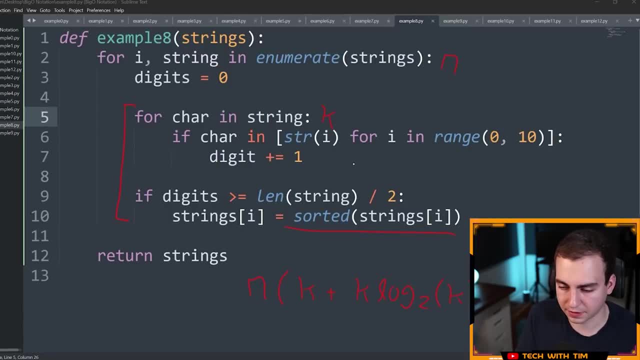 because we're going to do that at most end times. Now, though, we're able to simplify things because we have K plus K log base two of K. You can do the factoring here, and you'll see that we'll get K multiplied by one plus. 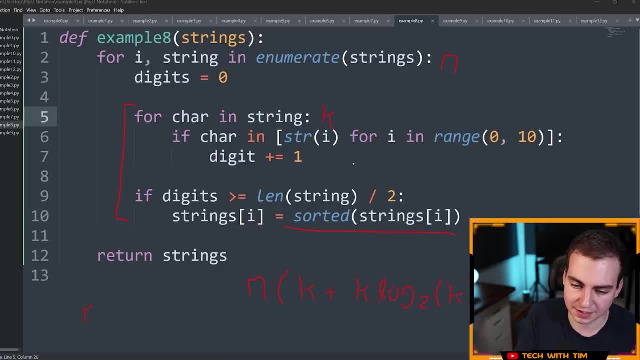 Log base two of K, which means we could get rid of the one, And so I can instead now say it's going to be N and then K and then log of K. So this is my time, complexity. I can parenthesize it if I'd like, but it's going to be N times K. log base: two of K. All right, there we go. 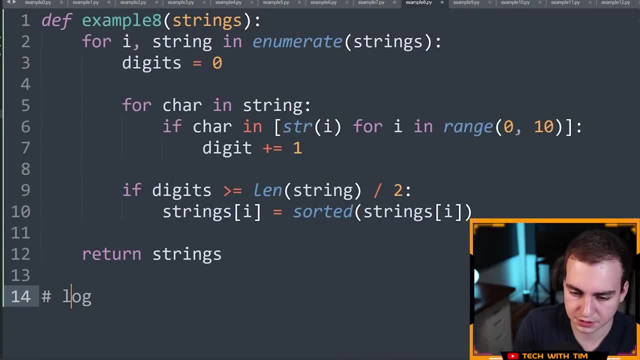 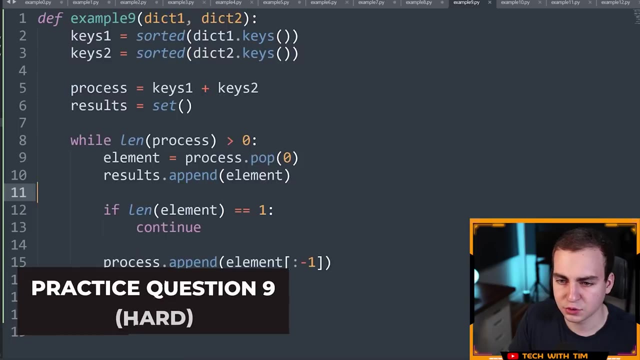 So that is that time complexity. I'm going to start going a little bit faster, just because we've looked at these a lot already. So it's going to be N K, log two K, and we can write it Like this, if we'd like, uh, and maybe even do another parenthesis, although it doesn't really matter, All right. So now let's move on to. 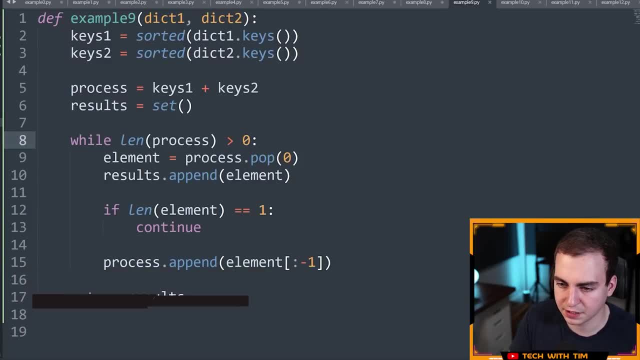 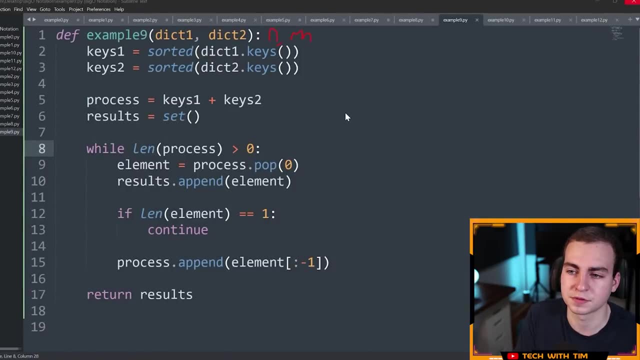 example nine. Okay, This one's a complicated one, So please pause the video and try to figure it out. but let me explain it out. We have two keys or we have two dictionaries, Sorry. So I'm going to say these are N and M in terms of their size, And these dictionaries are going to 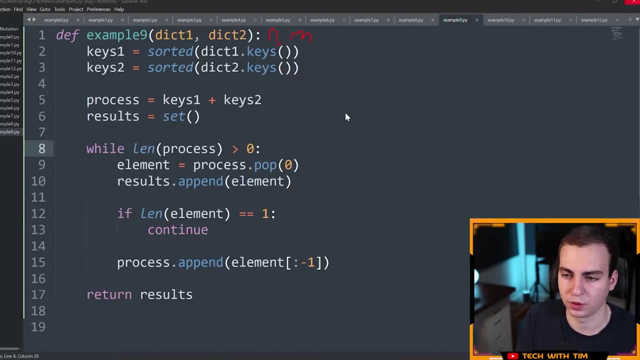 have key uh or sorry, string keys, Okay, Or keys that are strings, whatever. So I say keys one and keys two and I'm sorting a bunch of strings. Now, to sort the strings, we're just going to say that this takes N and then this is going to be. 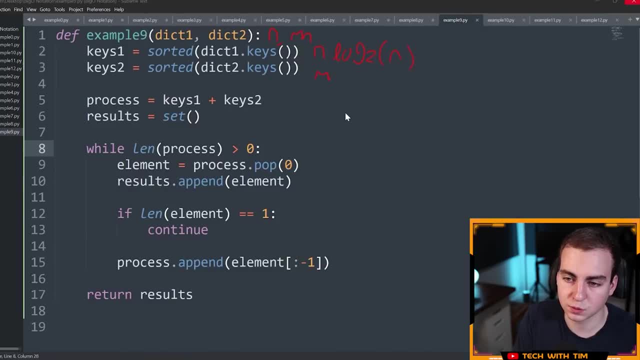 Log base two of N time. And then, for this one, since we're sorting dictionary two, which is M, we're going to say: this is M log base two of M. Okay, Now we have our process. Now we have keys one plus keys two. Now there's going to be N keys in keys one and M keys in keys two. So this is 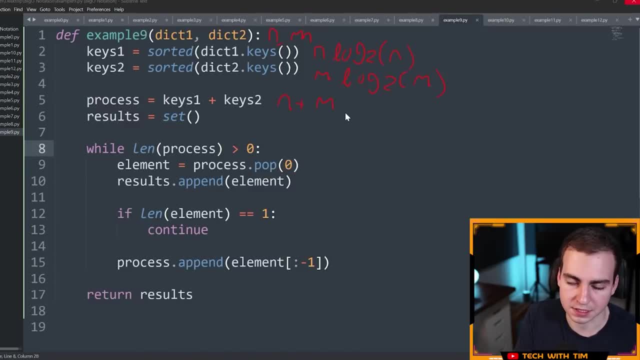 going to take us N plus M time to create that make a set constant time operation. Now we have this wallet. Now what we need to do here for the wallet is figure out how many times it's going to run and then how much or how much time it takes. Sorry, 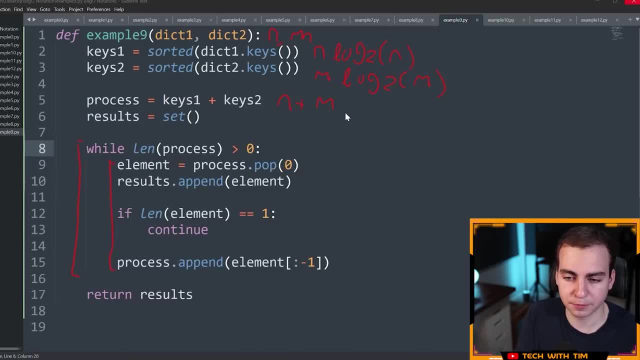 Inside of the while loop? uh, to reform operations. So how many operations are we doing in the for loop? How many times is the uh or sorry? how many operations are we doing in the wallet? How many times is the wallet run? Multiply them together. There we go, We have the 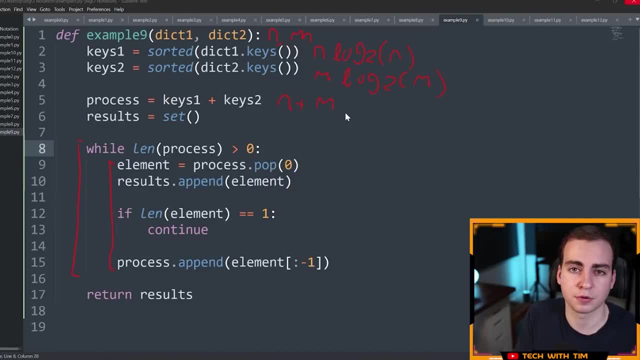 time for the wallet. So let's start by figuring out the operations in the wallet. So we have: element equals process dot pop zero. Now popping from zero immediately tells me that this is going to be a big O of N operation, or in this case, N plus M. So let me show you what I mean. 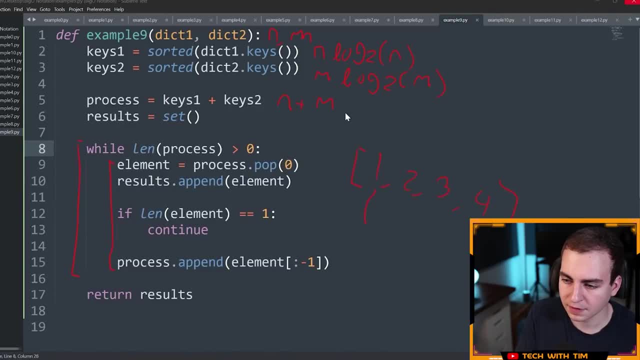 If we have a list, and let's just say we have four Elements, If I pop the first element and remove this element, what that means I have to do is shift every element over one position. Okay, To restore its position in the list. Uh, there is data structures that allow you to do this in constant time. However, the data structure list in 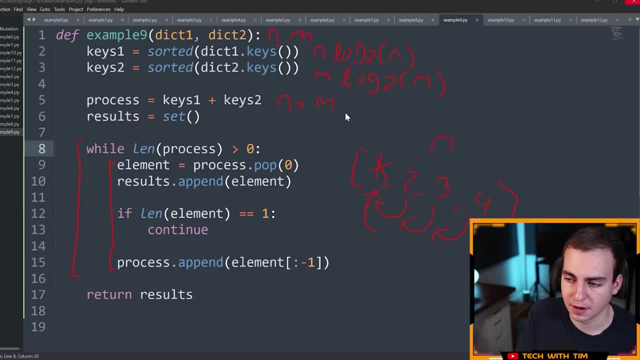 Python does not. So this is an O? N time operation, where N is the number of elements in the list. Now, since the number of elements in our process list is going to be, at most, N plus M, that means we're going to have to take- if I could- freaking erase all the 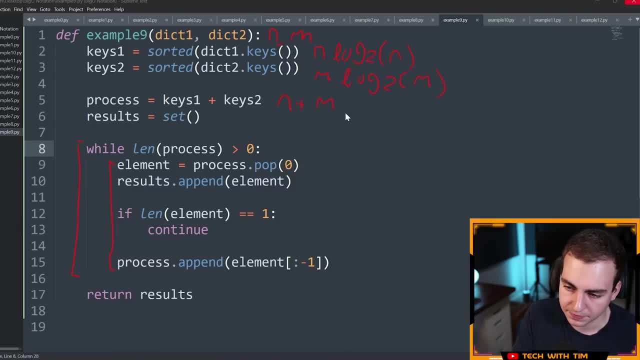 stuff here: N plus M time to perform these pops. So I'm going to say, okay, let's get this properly, N plus M. Now again, we're not always going to have N plus M elements in the process list because we're removing elements. That's what we're doing in here, But the most 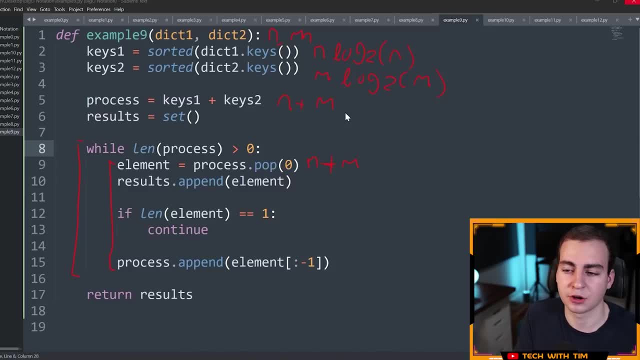 we will have when we start as N plus M. So we need to write that here as how much time this operation will take, in the worst case Continuing. we add something to the results list. Don't care about that. We're checking the length. Don't care about that. Now we have. 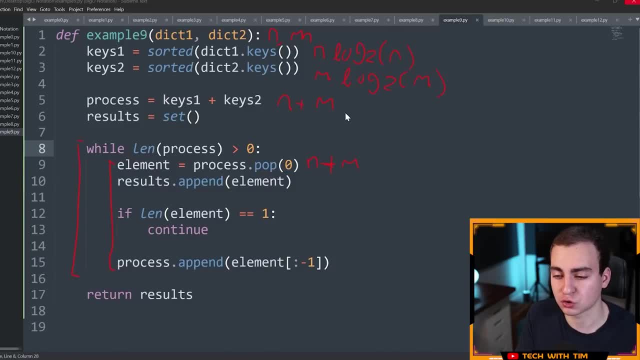 process dot append. Now what We're going to do is we're going to do a process dot append. Now what we're going to do is we're going to do a process dot append. Now what we're doing is appending a string, but we're removing the last character of the string. So what you need to realize is happening here is we are. 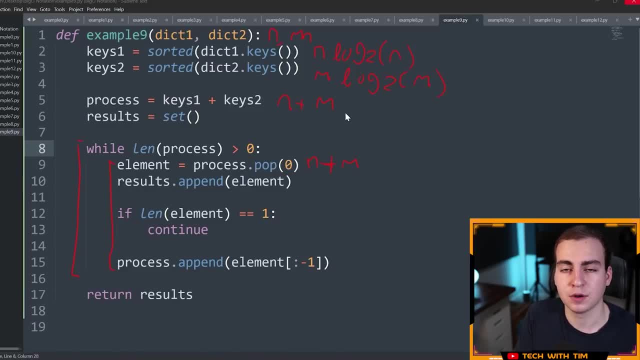 processing every single string key in both of the lists and we're going to keep adding the string itself back into the process list until it has no elements left in it. So for every string that we process, we're going to be adding that string minus its last. 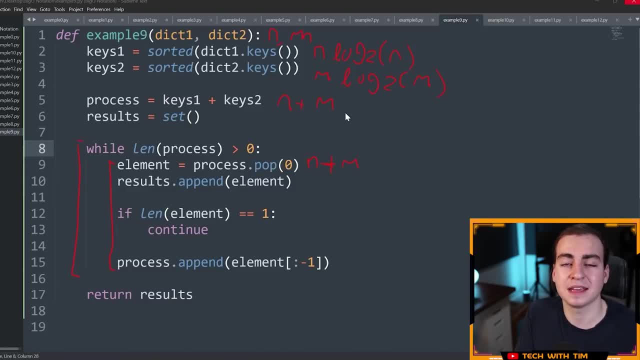 character back to the process list, whatever the length of the string times is. So if I have a basic string like high, then what I do is I strip off this last character, but I add H back to the process list, which means it needs to be processed again, causing the. 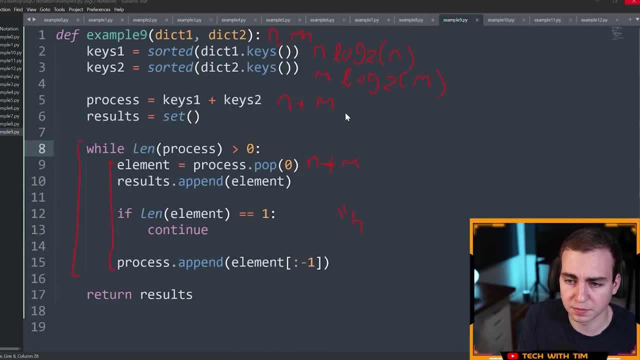 while loop to happen another time. So again more complicated algorithm here. but I wanted to show you how you come up with these time complexities. So, since that's the case now, what I need to do is say, okay, well, the while loop is going to take the existing process time. 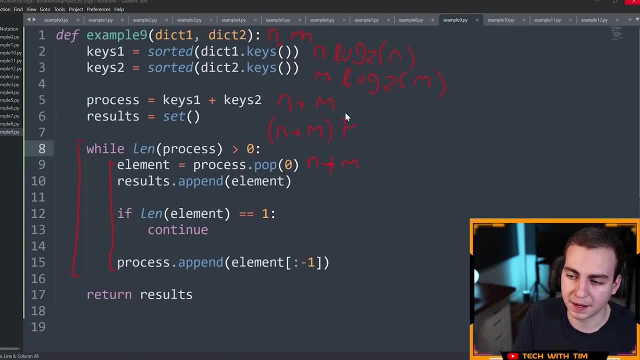 right, So N plus M, but this is all going to be multiplied by K, where K is the length of the longest string. So the most amount of times that one single element is going to be reinserted into process is K, because that is well the length of the longest string. 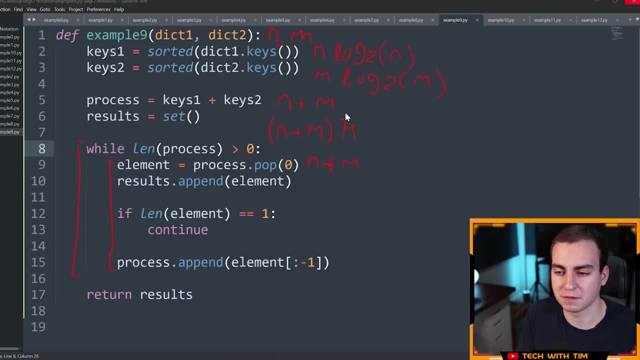 right. So if I have a string, the longest string is five. Well, it's going to take me five reinsertions- It's really going to be four, but still we're going to have to process that element five times by adding it back into the process list. So I need to multiply the maximum length of the 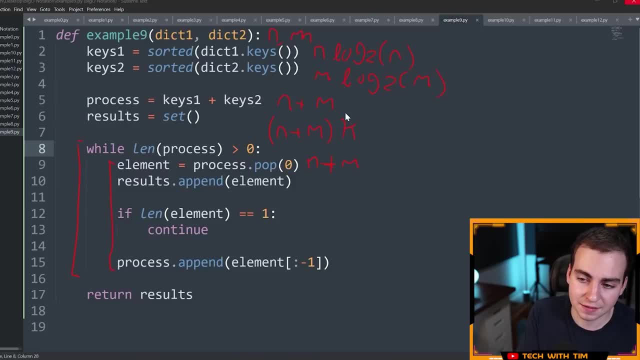 string by N plus M, which is how many elements are already in there, because for each of those elements they could be inserted a maximum of K times Um. again, I know we're getting into the weeds here. It's getting complicated, but I wanted to give you some advanced examples because this is stuff that you're going to have to learn at some point in time. So N plus M. 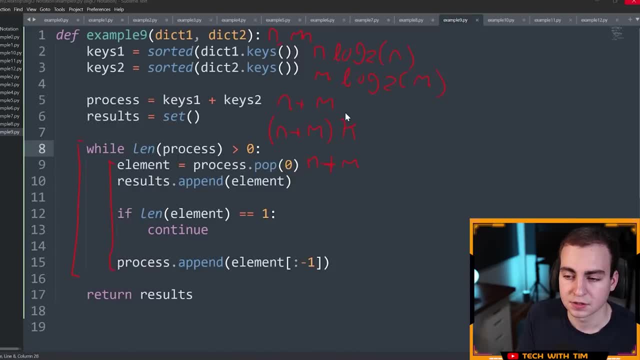 multiplied by K is how long this loop is taking. So now what we need to factor in here is N plus M multiplied by K, going to be more or less than N times log base two of N and M times log base two of M, because now we have to add these operations together. So really what we're going to have is N and then we're going to have log base two of N. Then we're going to have N plus M multiplied by K. 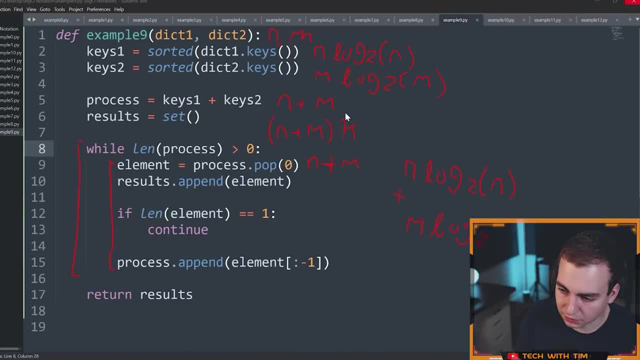 Okay, So we're going to add that to M of log base two of M. Then we have this operation, which is N plus M. Now N plus M we know is going to be less than N plus M times K, So we can simply remove that from our operation here And then we're going to have N plus M multiplied by K. Now we actually do not know if N plus M times K is going to be more or less than N log base two N and M log base two M, So we need to keep them in. So this would be our total time complexity here. Okay. 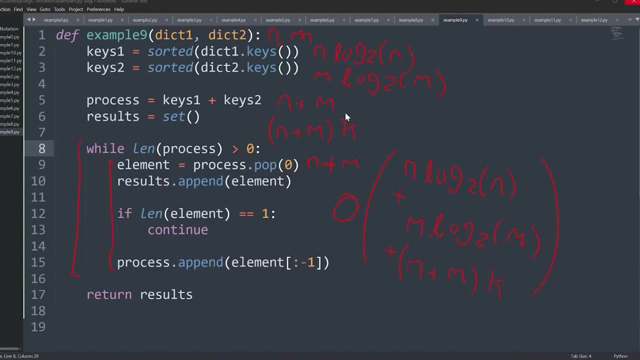 Okay, N log base two: N plus M log base two, M plus N times N times K. And then you would write after this what each of these variables mean: M is the number of keys in dictionary one, M a number of keys in dictionary two, and K the length of the longest string out of dictionary one or dictionary two. Okay, Again, I know, really complicated one, probably not one that you're going to get on like a computer science exam, but it's possible. So I figured we'd go through this example here. Okay, Let's look at example 10.. 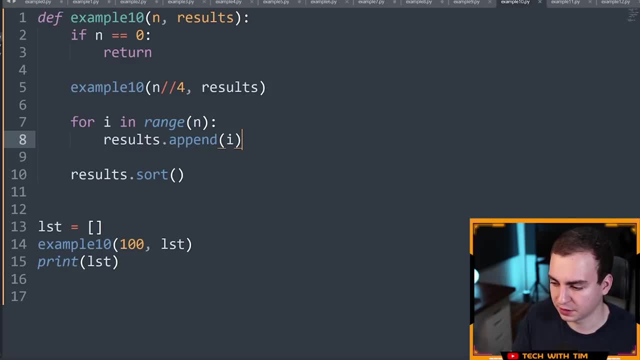 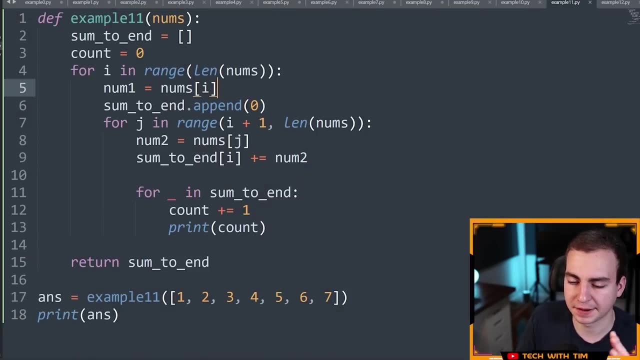 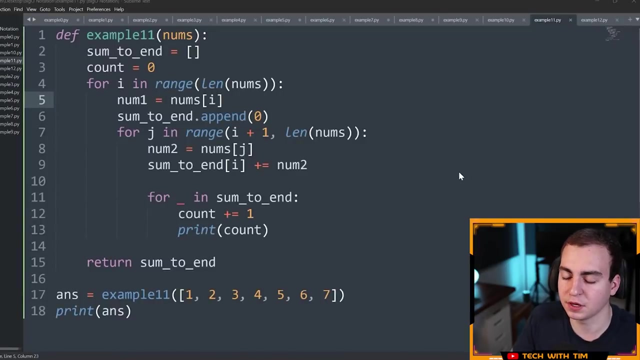 Okay. Okay Now example 10.. Again, we're getting into more complicated ones. Only got three left here. Let's take a snip. uh, pause the video and give it a go. Okay, So actually we're going to skip example 10.. I was just going through it and it's way too complicated to even try to explain in this video. So if you guys want to guess the answer, you can in the comments down below. Um, anyways, we're just going to move on to 11, cause it's a bit simpler. I don't want to overwhelm you guys too much, So let's just understand this code before we proceed any further. We have some to the end empty list count equals zero for I in range the land of nums. Okay, We're looping through getting one number. 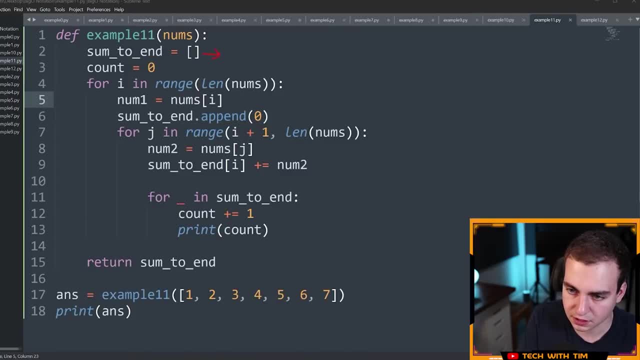 Then we're saying some to the end on a pen zero. So this is going to approach. and then we're looping through all of the numbers past this number in our list. Okay, Cause I plus one is the start of our four loop range up to the land of nums. So that's N right. Okay. Then what we're doing is saying some to the end: I plus equals num two. don't have to worry too much about the addition. We have another four loop in here that is going to loop through all of the elements in some to the end. So whatever the current length of this list is, that's how many times this is happening. 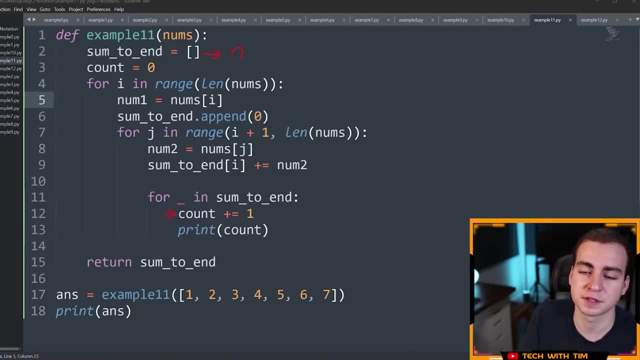 And then we're printing out our count, which is just how many times this for loop has happened in total. So you can read this and understand a bit more. I know I didn't really necessarily explain it. The point is, this sum to the end list is going to contain the sum of all of the numbers. 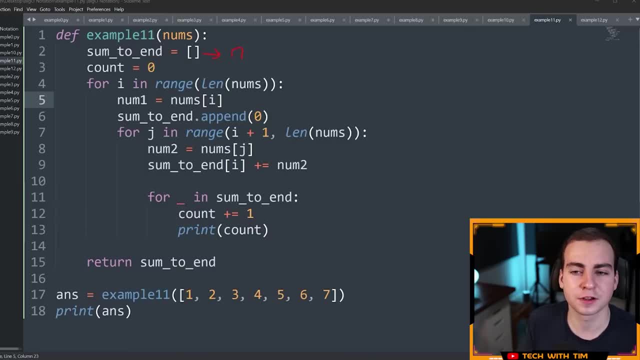 in the list past the current number, not including the current number, until we get to the end of list. That's kind of what it's doing. So if we have like one, two, three, four, then the result here is going to be whatever. two plus three plus four is So nine, and then whatever three plus. 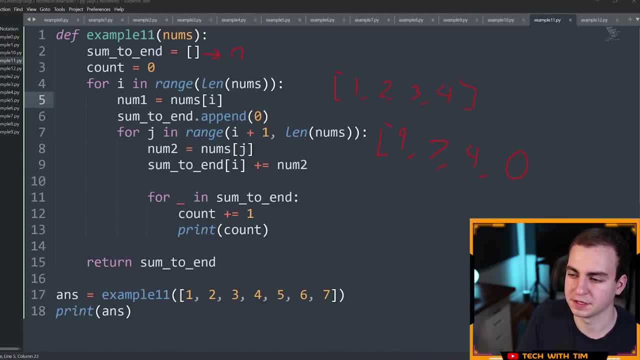 four is which is seven, then whatever four is which is four, and then zero. Okay, That's what the result's going to be, Cause we sum these three, then we sum these two, then we sum this one and place those in the appropriate positions in the list, And then we would sum the last. 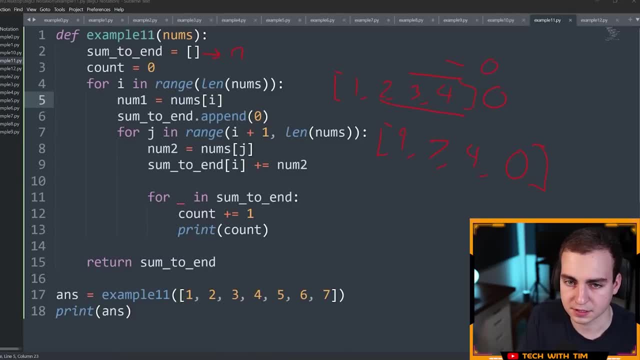 element which, which would be zero. So we place here at the end: Okay, Let's just get rid of those, though. That's what this code is doing, Okay, So now that we understand that, let us continue and do this time: complexity. So we're going to. 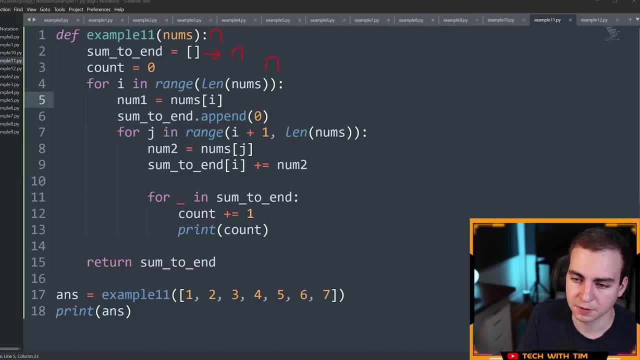 say: this is N All right. So that means this happens N times. And then here what's going to happen is: this is going to happen N times, then N minus one times, then N minus two, then N minus three, as I increases. Now, if you actually look at the value of the sequence, you'll see that it 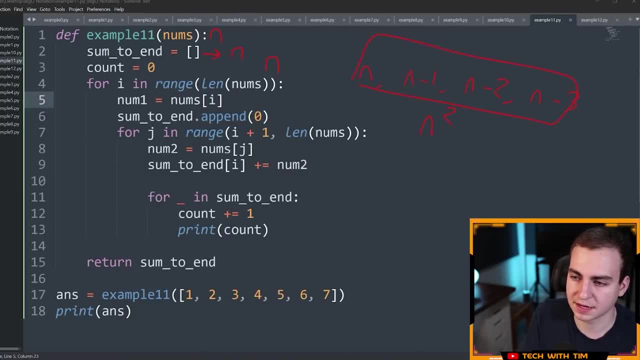 approaches N squared, So we can simply say that all of these added together is N squared, Okay, Which means that we can just kind of write this: as it takes N times, Okay, We don't need to factor in all the minus, ones or minus. 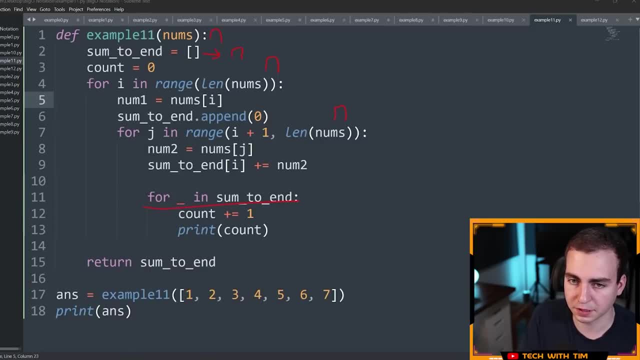 It's just going to be N minus two is minus three, so on and so forth. Now continuing, we have another four loop. Now this four loop is happening, whatever the length of sum to the end is. So it's going to happen first, one time, because that'll be the length when I equals one. then it will happen. 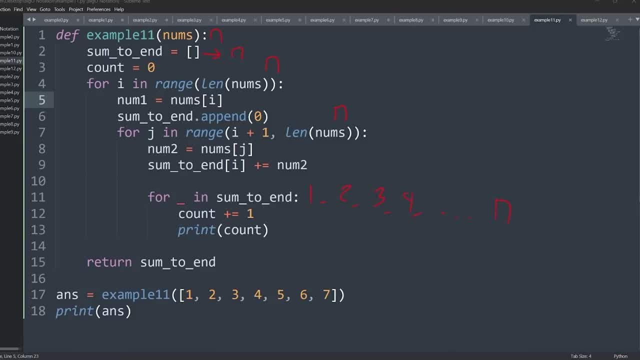 two times, then three, then four, all the way until it gets to N. So, similar to how we had N minus one and minus two and minus three here, that's exactly what we have in the reverse order. So we know that we can just say that this is going to take N as well, because one plus two plus three plus four. 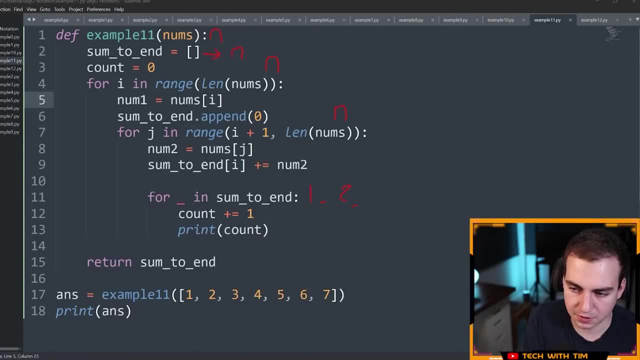 and approaches and squared Again. don't want to drive all the math here, but I'm going to write that this takes it. So we have n multiplied by n multiplied by n, And that's all that we're doing inside of here. 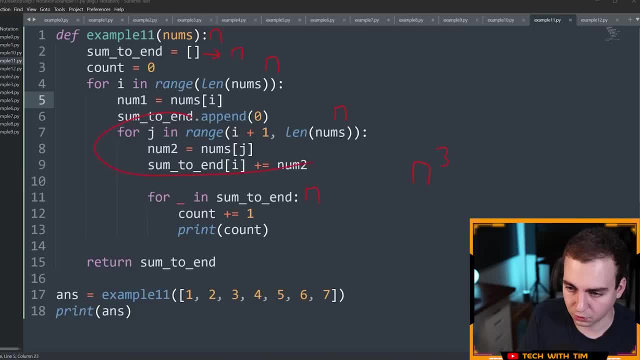 which is going to give us an n cubed time algorithm. So this for loop happens and times since inside of here, this for loop happens and times we get n cubed. So that's the time complexity, Big O of n cubed Great. 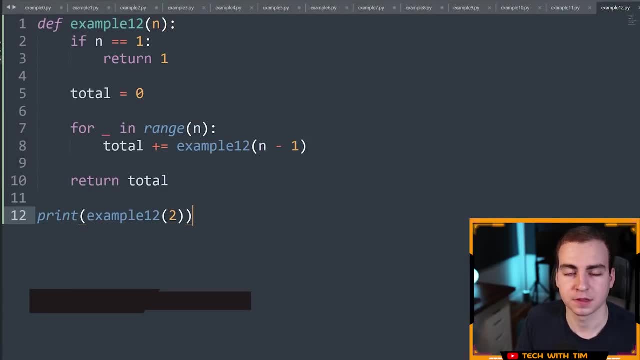 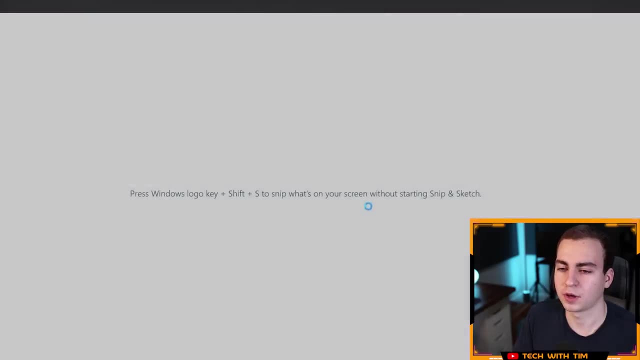 Let's move on to the last example here. OK, another complex example. Pause the video. Take a guess. Let's go through the time complexity right now. OK, so I'm just going to tell you the time complexity here is n factorial. 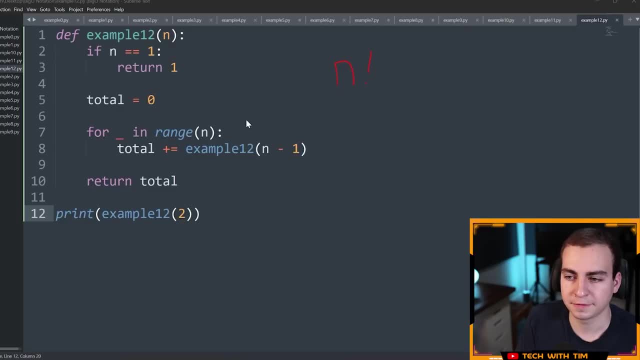 Now, if you're unfamiliar with the factorial, obviously you would not have guessed this, but a factorial is the following: So if I have something like four factorial, it is four times three times two times one. If I had three factorial, that's three times two times one. 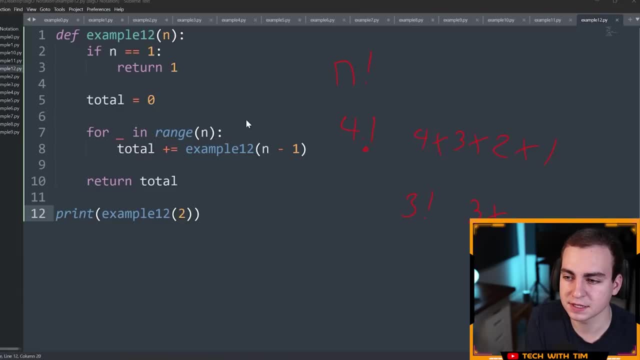 OK, that's factorial. So we see these in time complexities and a fact, or is one of the worst time complexities that we can have. Refer to that graph I showed earlier if you want to see exactly where it ranks. believe it's actually the worst. 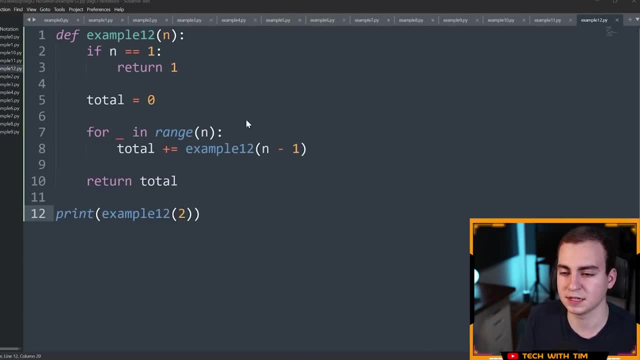 that was on that graph. So n factorial is this time complexity. But how do we determine? Well, this is recursive, so we're going to have to find how many times this recursive function runs and then multiply that by how much work is being done. 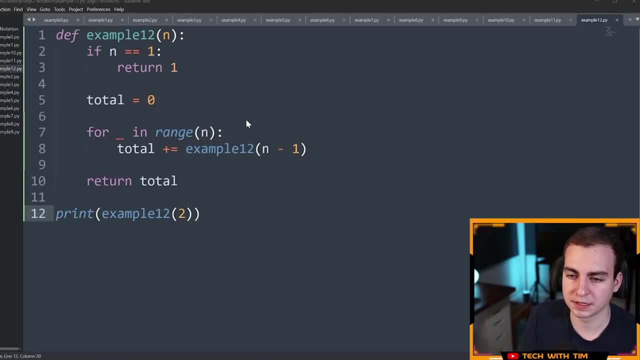 OK, so we have n work being done inside of the four. You know, before we do that, let's look at the recursive calls. So we say: if n is equal to one return, one total equals zero, Four underscore in range and total plus equals example 12. 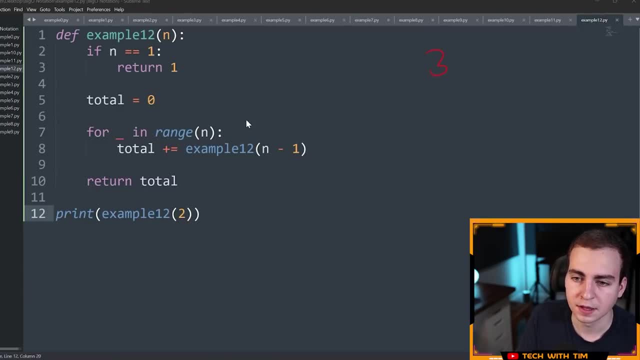 and minus one. So let's try this with an input of three. If we try this with an input of three, let's say n is currently equal to three, What happens is total is equal zero. or saying for I in range and, and then we're going to call. 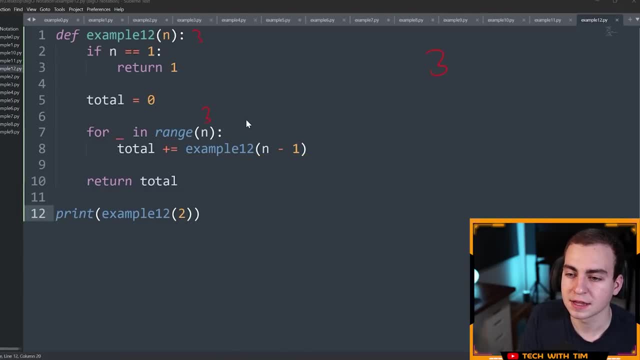 example 12 with n minus one. How many times we call this? three times. OK, we call it n times, or whatever the input to the function was. That's how many recursive calls we do. So we have one to three recursive calls. 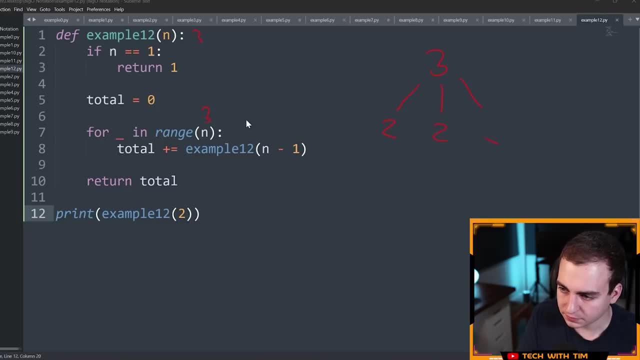 all to the same value, which is n minus one, which is two. OK, so there we go. Now, what happens is we come to the function and now our input is two. It's not once. we continue, So we're looping through two. 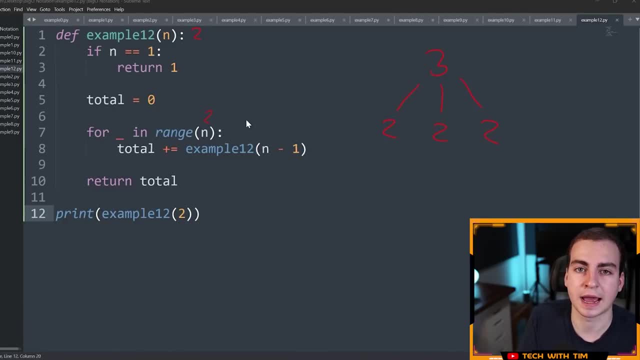 and then we're doing this How many times? Whatever n is, we're going to now have two recursive calls, with n being less than one. OK, so we're going to say one, one, one, one and one one. 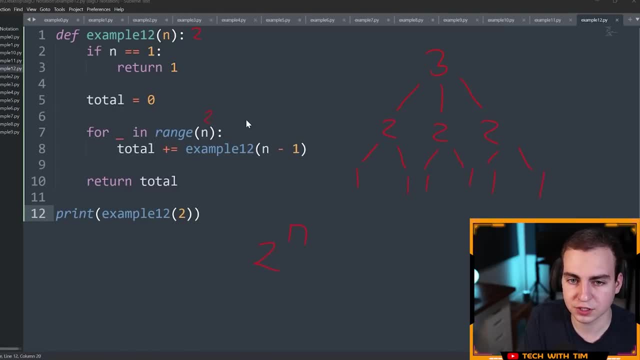 Now this is going to look very similar to the, to the exponent n, except what you're going to realize is that the levels in each tree, or the, I guess, width of each section of the tree, increases as the input increases. So if I have four, I have one. 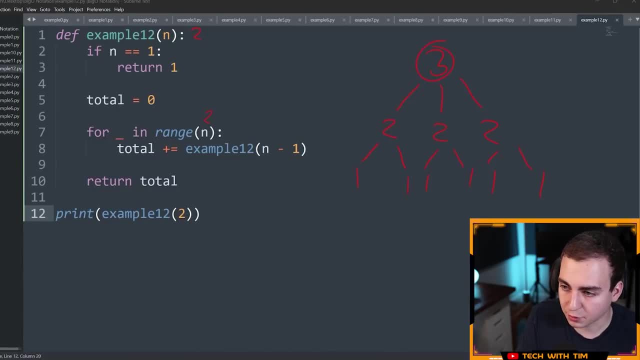 two, three, four, right? So let's say I have three levels here. Well, now what I'm doing is I'm saying, OK, I'm going to have three levels and I'm going to multiply that by however many levels this one's going to have. 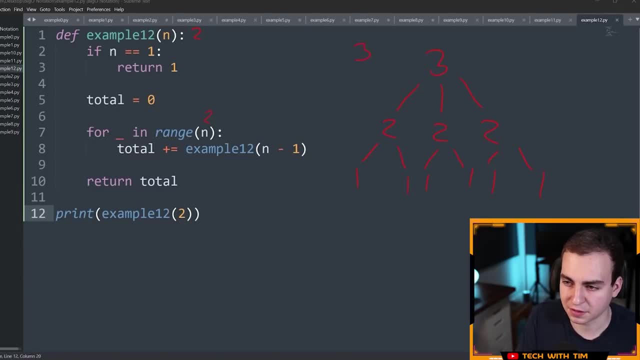 And this is going to have how many levels? is going to have two. So that gives me three times two levels. Then how many levels does this one have? It has one. This is a factorial. That's what the tree looks like Now. again, I know this is confusing. 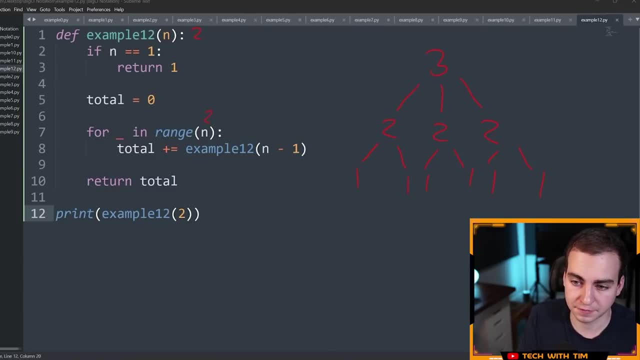 I know this is a little bit confusing. I know a lot of you are going to be lost at this point, but this is the factorial algorithm And if you look at this and I punch in a number, say like I guess what's the factorial five? 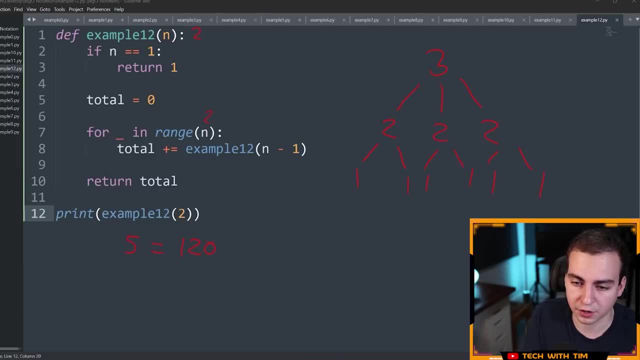 I believe it's 120.. We'll get 120, meaning we had to do 120 operations, because that's the way that we've calculated them. So that's what I was trying to illustrate here with the factorial. Let's just look at one more. 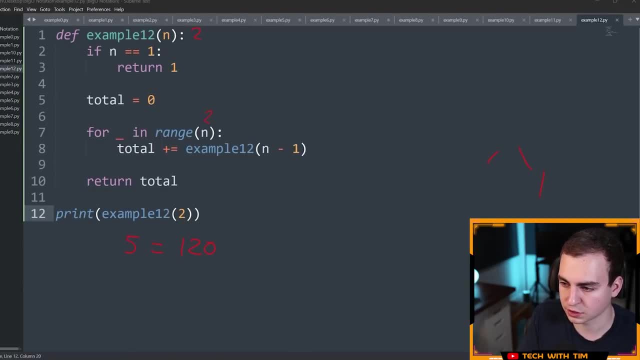 higher tree level of four. so you can really see kind of how this works. So if we have an input of four here, what happens is we get four calls for recursive calls that all go now to recursive calls of three, And then we get one, two, three. 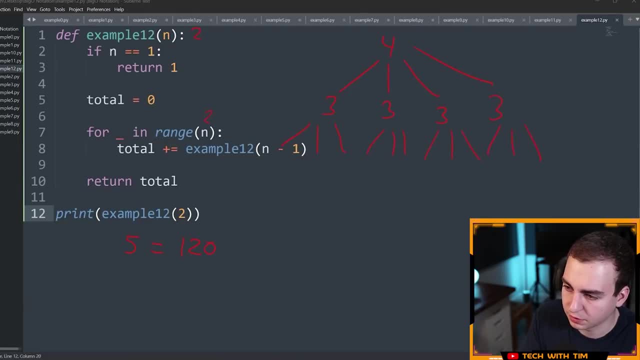 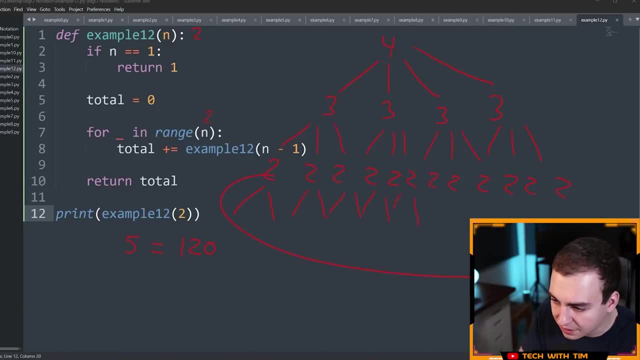 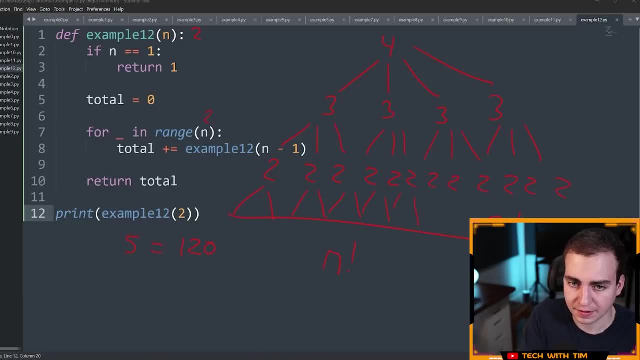 in the recursion that we have. This is n factorial. Now what we can say is that theoretically we're going to have an upper bound of two times n factorial recursive calls in total. So we hit the base case n factorial times but we're going to have in total. 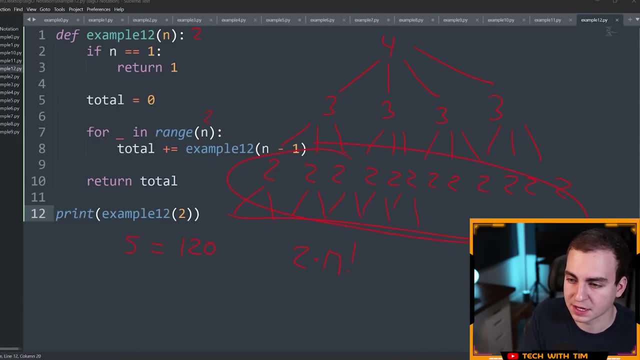 two times n factorial because to be able to hit the base case we had to do all of the other calls above. Now, since we have a constant, we remove the two and that gives us n factorial for the time. complexity of our algorithm. 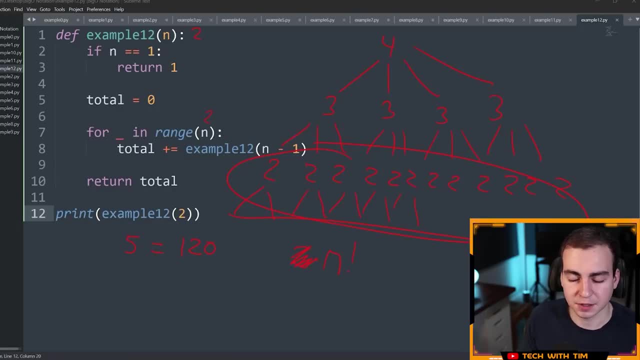 Again, hard to explain this in much more Definitely. But then this: for some of these things you kind of just get it or you don't, And you have to look at a ton of different examples to really see how this works. Understand factorials. understand math. 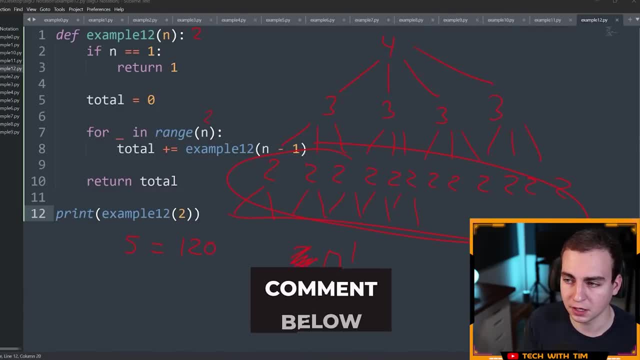 Maybe I'm just not the best at teaching it, Definitely open to your comments below, But that's really the best that I can kind of explain how the factorial works here. We start with four and then four, four. We're doing four. fact four: recursive calls. 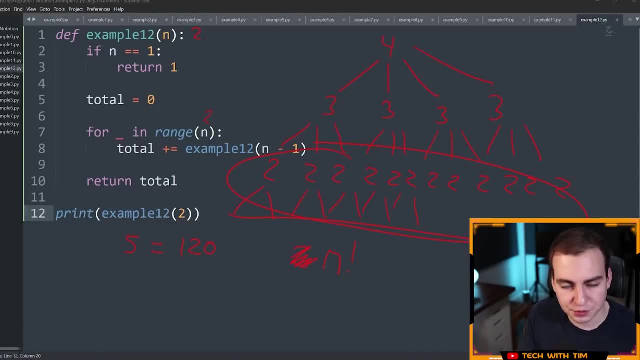 for every single one of those recursive calls. We're doing three recursive calls, Then we're doing two recursive calls, Then we're doing one call simply, which is just like returning one. So we're not really doing a call, but we're returning a value.